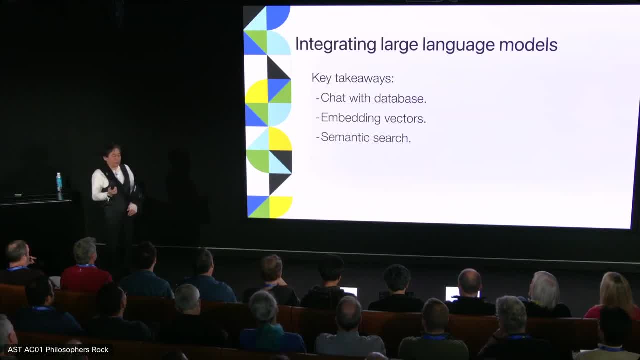 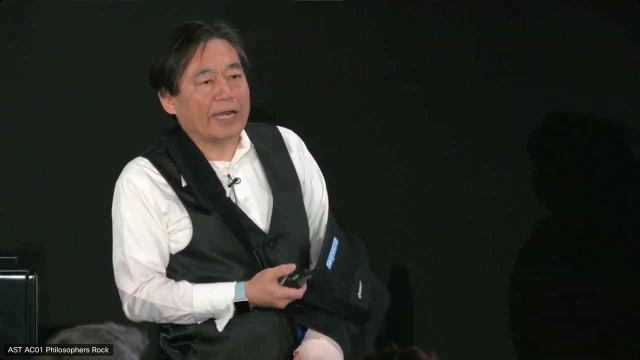 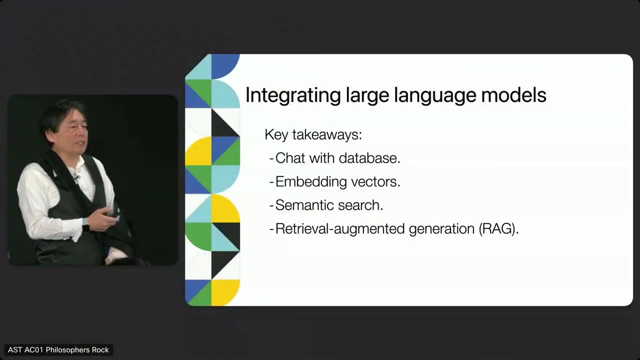 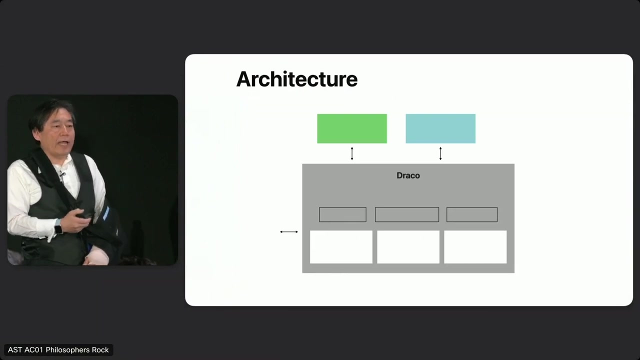 natural language besides the keyword search or regular expression you can have today. Then you will know how to do retrieval, augmented generation, the so-called RIG. Simply put, that's you can chat with document besides chat with database. So here is a high-level. 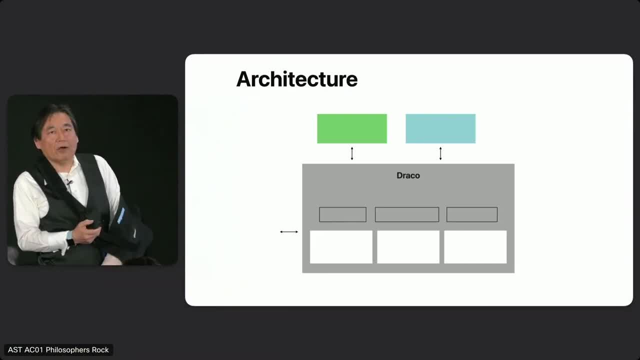 overview architecture we have enhanced to make the LLM integration. First, we build an add-on called App Assistant to help you to chat with database. So the add-on using the stuff you're familiar with: HTML, JavaScript, FileMaker script step. 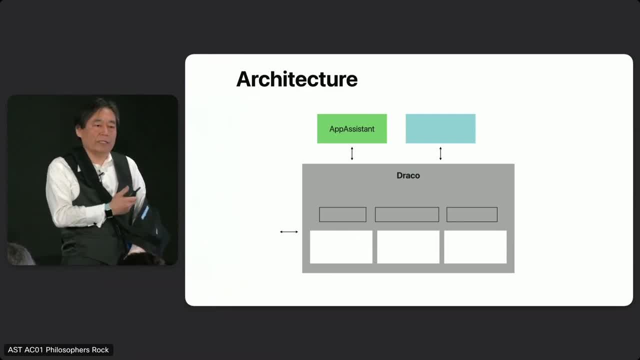 and the FileMaker calculation formulas. So it could be a good starting point for you and you can customize if you need And we build a whole new set of the FileMaker script step to support LLM integration, along with the calculation functions. 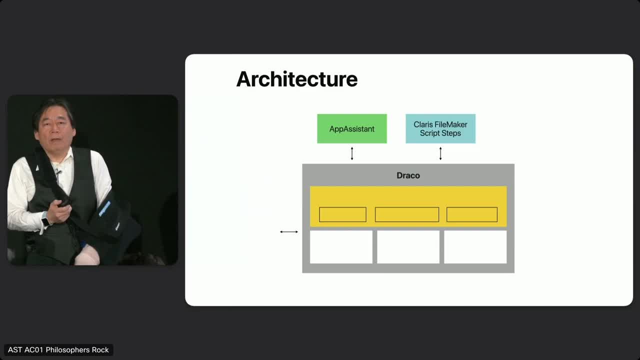 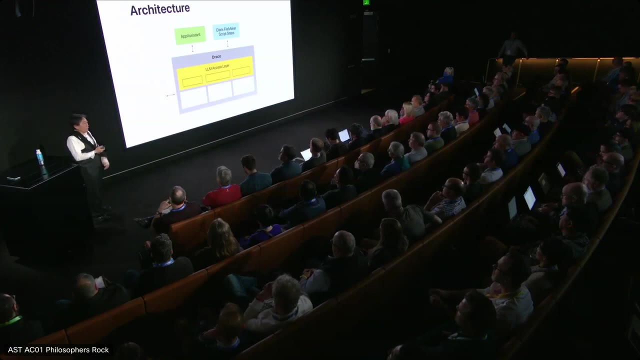 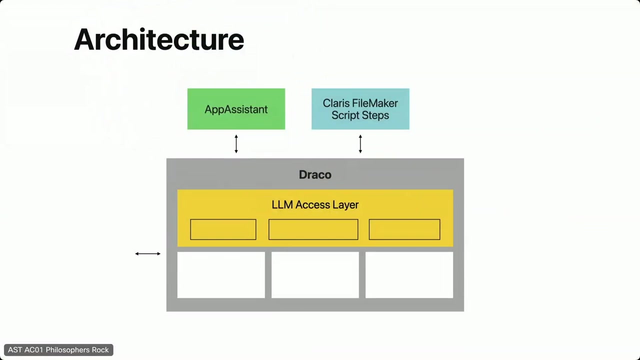 Inside the Draco database engine. we have built an LLM access there to encapsulate those command protocol and functionalities inside And we use a handle approach. Most of you probably are familiar with the ESS feature we introduced maybe 15 years ago. So remember you can integrate with other DPMs like Oracle. 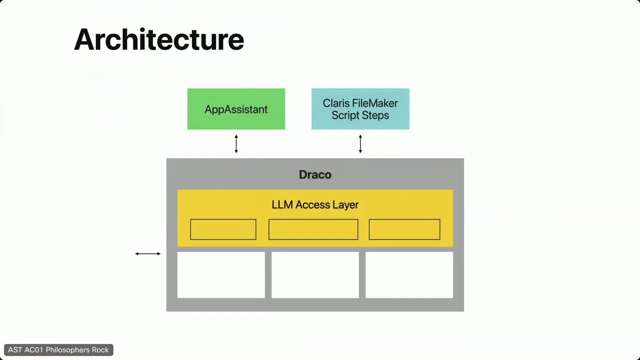 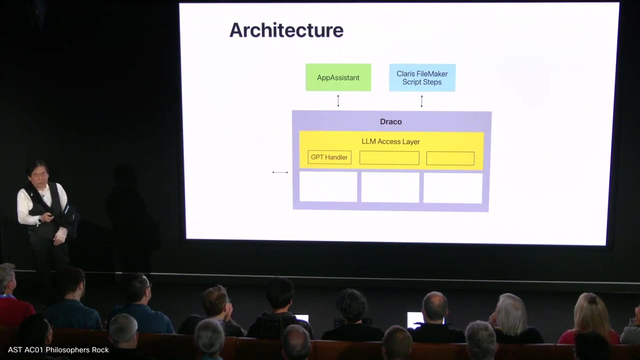 MySQL SQL Server. so we have a handle inside database engine. So we use a similar approach here, So we build a GDP handle inside it. to talk to the open AI GPT, that's a GPT 3.5, GPT-4, GPT-11-06, up to your choice. 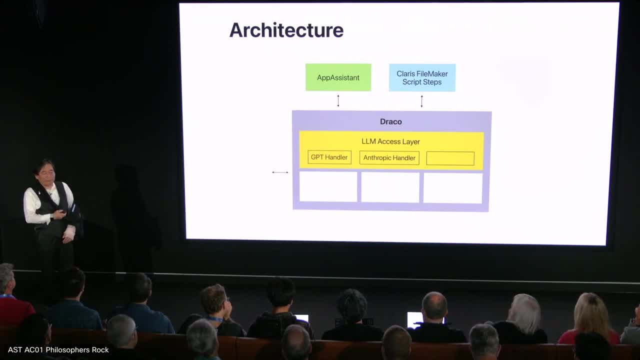 And we build an anthropic handle to talk to anthropic handlers. And we build an open source handle to allow you to talk to open source LLM. if you choose to kind of set up your own LLM server So underneath it we also enhance other modules to support it. 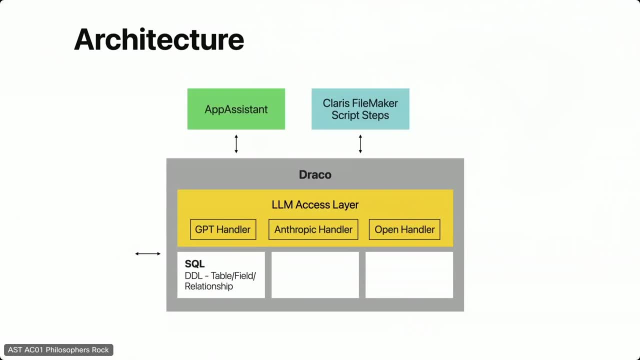 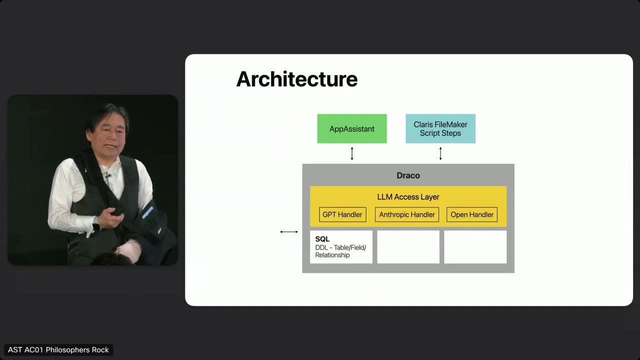 For example, in the SQL module. we improve in the SQL parser And we add the DTL to support it. DTL, the data definition language- there to encapsulate the schema that's needed to send to LLM. The reason you need a DTL is to support check with database. 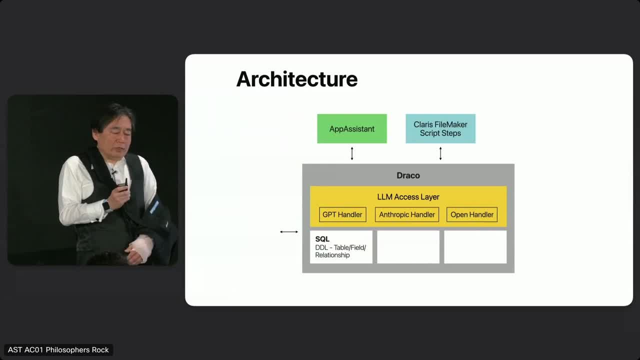 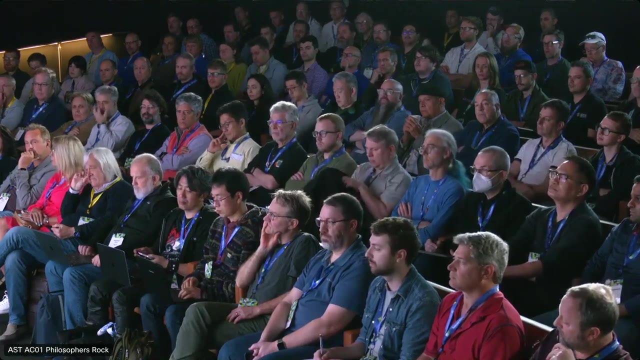 We need to let LLM know what kind of your miniature schema is. So then LLM will be able to generate correct SQL statement for corresponding to the user's natural language prompt. So later I will go through some detail about the DTL. 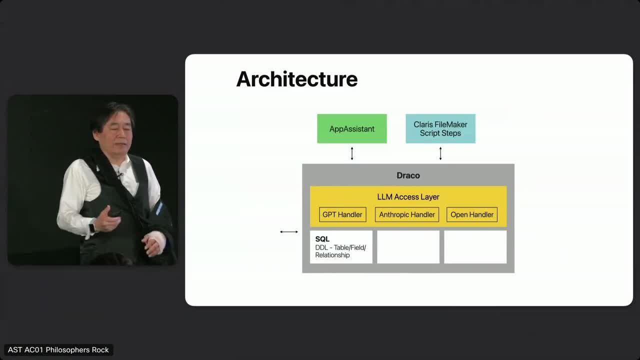 But in a way it just needed to do a little bit of things And the heavy lifting actually will be done by the Jericho database engine for you. So we support embedding vectors. So most of you are probably familiar with the search index. 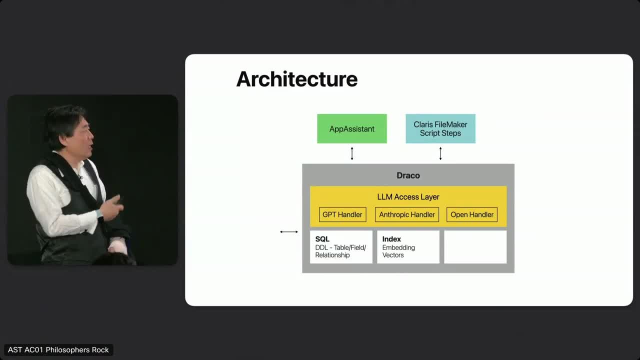 sort index the Jericho database engine has for years So embedding vector. actually, in certain cases, in a certain way you can think that's just another kind of index. But this index actually is based on the natural language meaning, But the dimension is much, much higher. 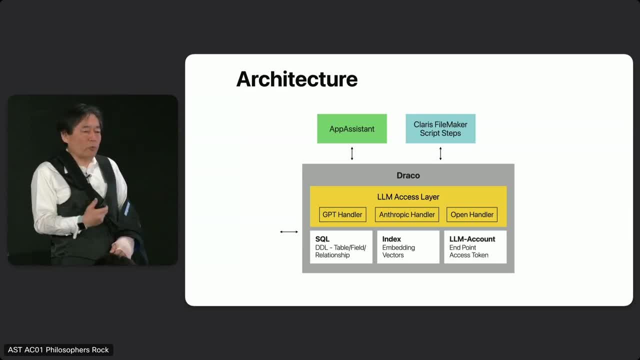 And we ask support for the LLM account. So each one has the endpoint access endpoint of the LLM server and including your API access token. So in Jericho database engine you can have multiple LLM account running at one time if you'd like to. 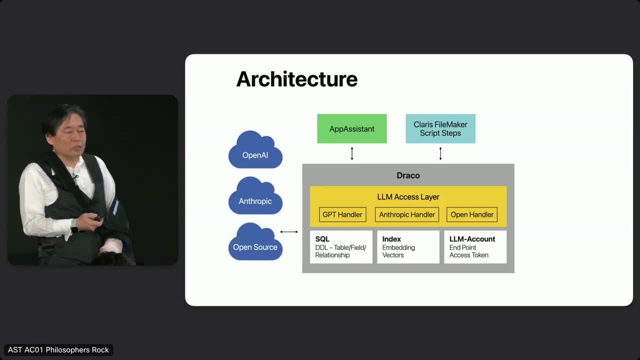 So with that, then, the Jericho database engine will be able to allow you to talk to OpenAI LLM or Anthropic LLM or Open Source LLM, or you want to have some of them access at the same time And once you build a solution. 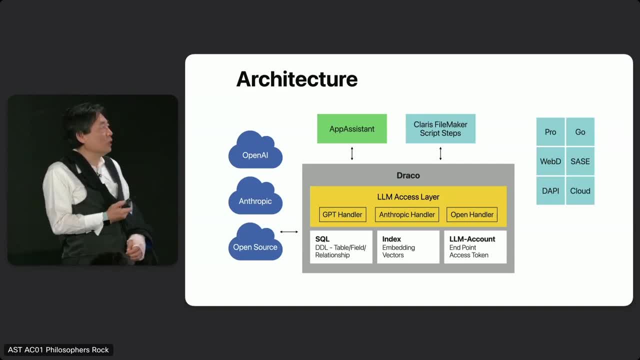 it will be able to run on FileMaker Pro, Go, WebDirect, Script, Engine, Data API or even Cloud if applicable, And we make that the cross-platform. on the OS, we support Mac OS, iOS, Windows and Ubuntu. 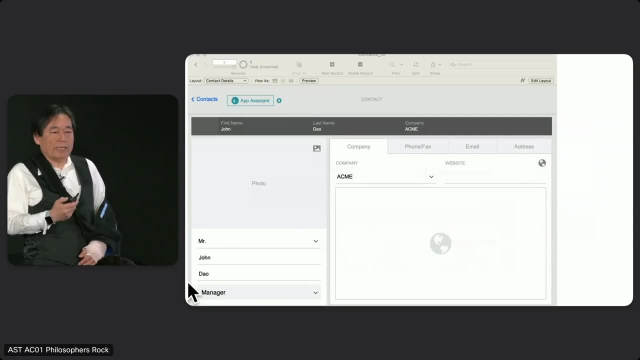 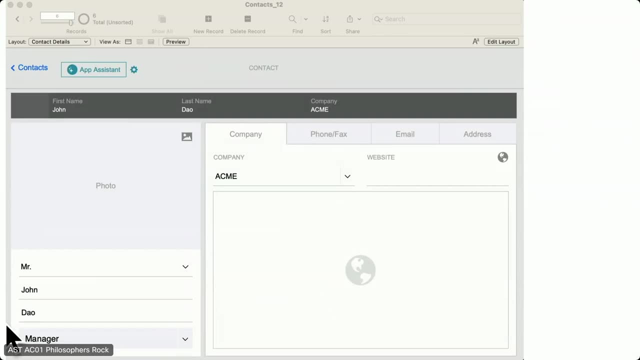 So now I'm going to show you a quick demo to check with the database. What you see is a familiar FileMaker Pro with the contact database. So the app assistant is the add-on. So this, Let's modify the record. So I have a John Doe here. 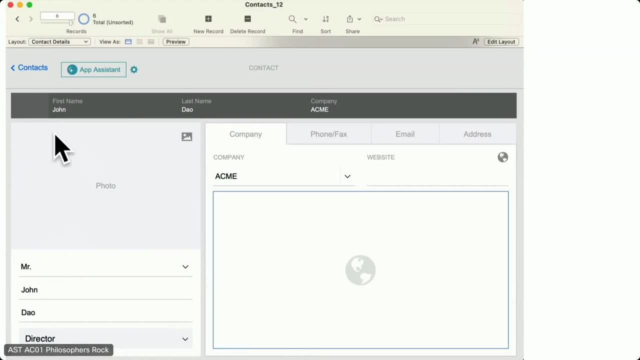 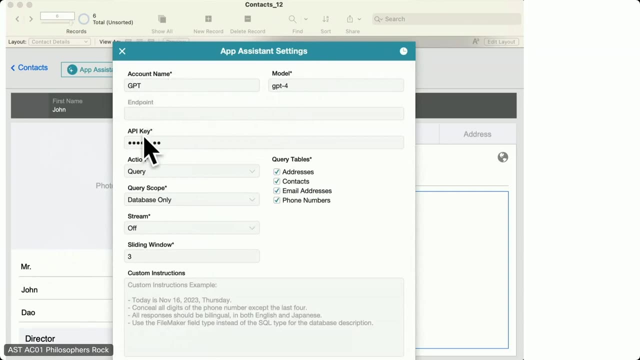 So John Doe just recently promoted, So I update it to new title: direct And let's check the app assistant setting. So I'm going to talk to the GPT-4 with my API key. In the action I need to select query. 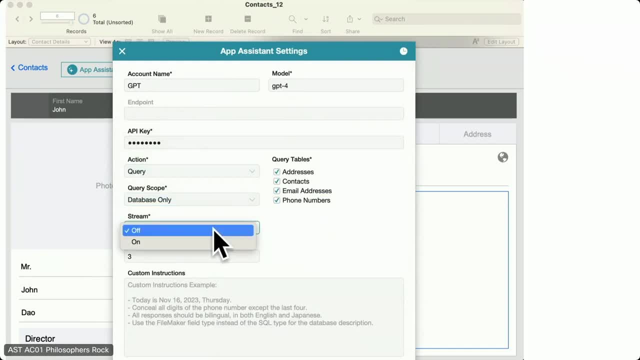 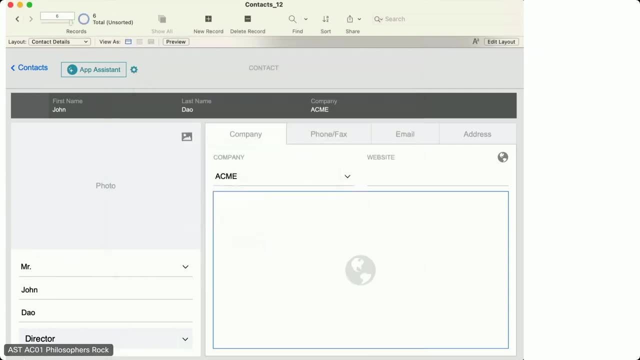 So, because I want to check with database, I want to set scope with database only, So don't worry about the option. I will go through detail with you, Okay, so now I have the setting I want. I double-check. I have everything for John Doe. 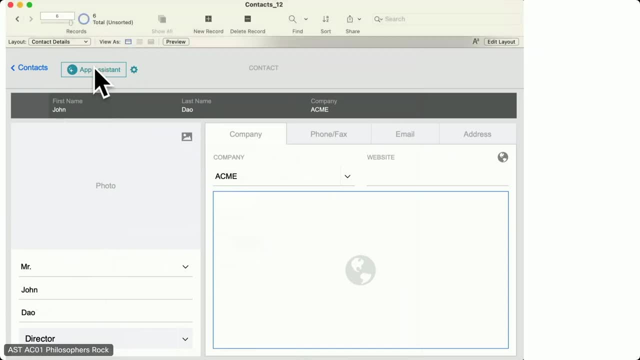 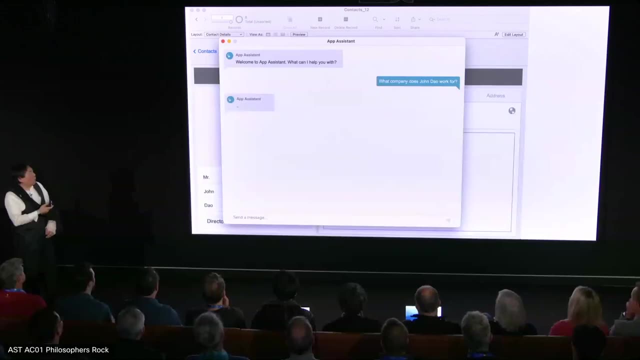 John Doe work for ACME. I have a phone number, email and so on. Then I click the app assistant. it pop up the window. So I start asking: question what company John Doe work for. So it check with database and get to the ACME. 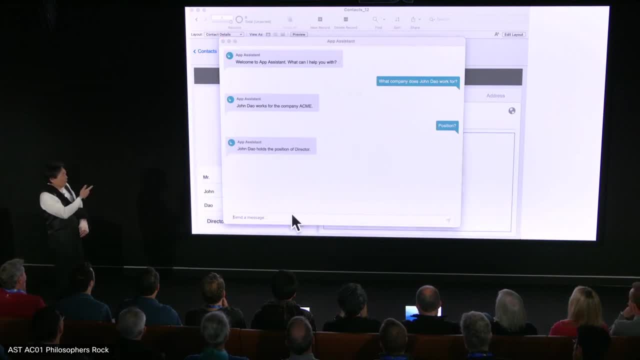 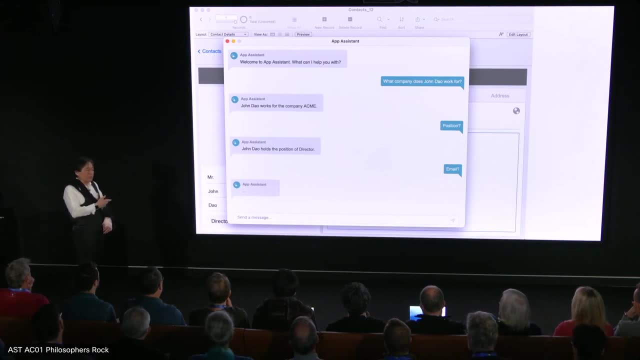 I continue to ask what's the position. So remember, I update to director If I direct. I keep asking what's John Doe's position or what's John Doe's email. Pay attention, I don't need to ask what's John Doe's position. 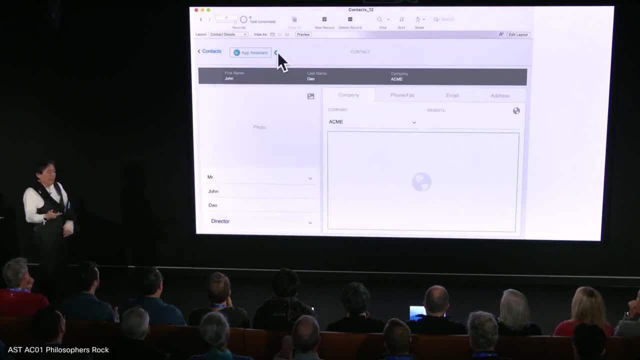 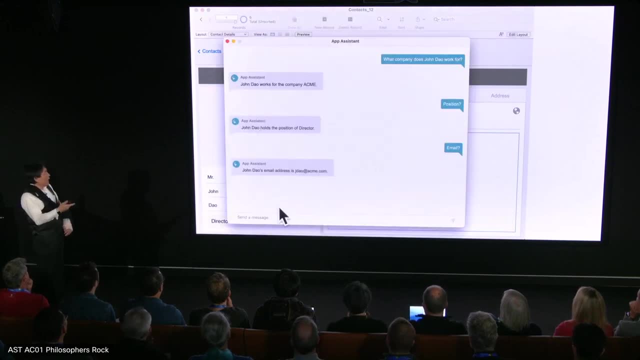 or what's John Doe's email. And you understand, I'm asking for John Doe, not for Peter, not for Mary. So now I want to show you the DDL. So now, if you want to debug or you're curious, you can repeat the question. 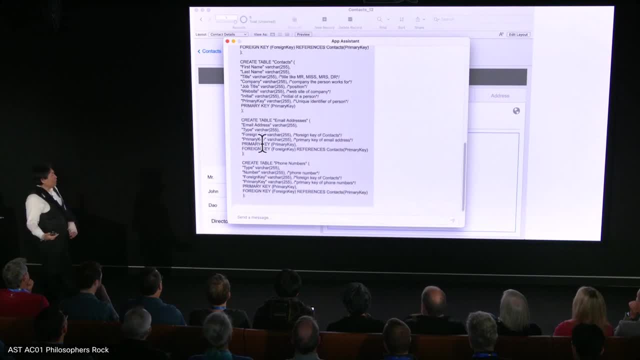 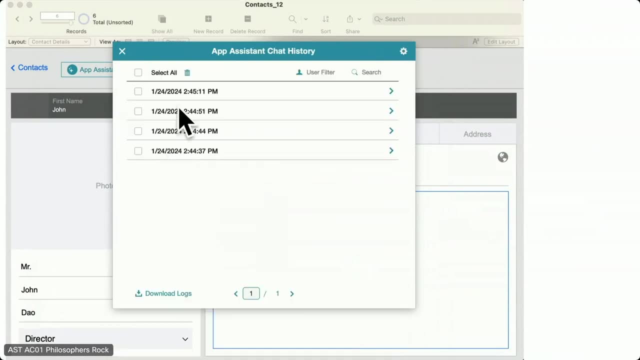 Now you see, this is the data definition language which Draco database in general for you send to LLM. This is the industrial standard SQL statement And we also have an including history So you can use that as an audit log. So we include a message response in the token use. 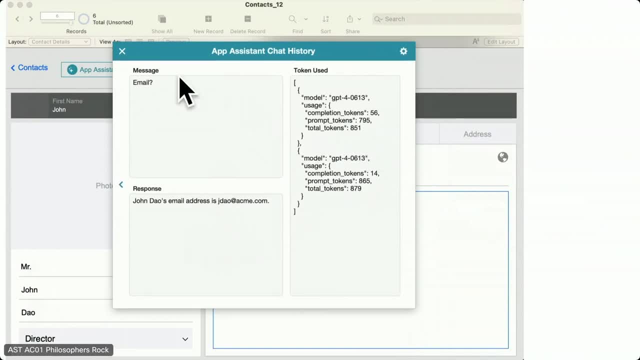 And about who did that and what time. And for admin, if you want to delete it, delete it differently than delete it. So that's a quick demo. we check with database, So you can check with database and you also can debug it to see the DDL, to see the SQL. 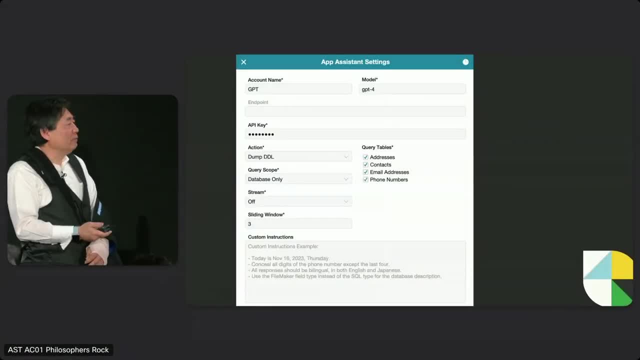 Thank you. So now let's take a look at some settings of the app assistant. So, from the top, the account name: the account name: you can specify any account name you like. And the model: you specify another model, Because I'm talking to OpenAI, I'm using GPV4.. 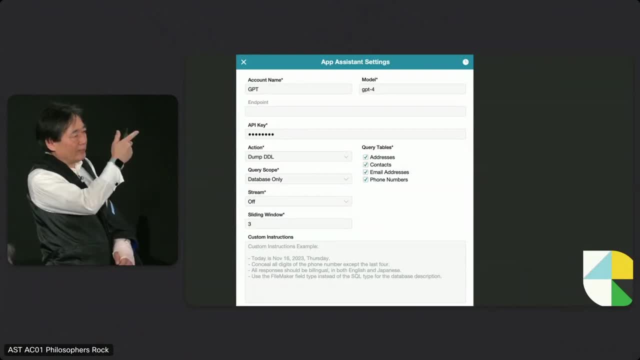 So I just type GPV4.. That is the case sensitive and also need that. the, the, the minus in between. yeah, And the endpoint is well known, so I you don't need to to enter it, We know that, so we can handle the endpoint for you. 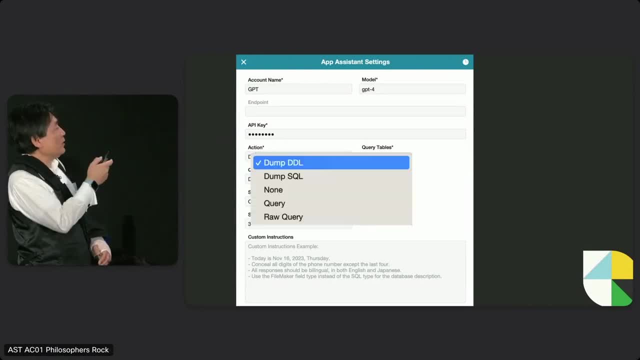 But you do need to enter your, your API key And actions. there are five actions available for you to choose. What you just saw is dump DDL. You can also choose to dump SQL, If you are curious about what SQL got got sent from LLM to. 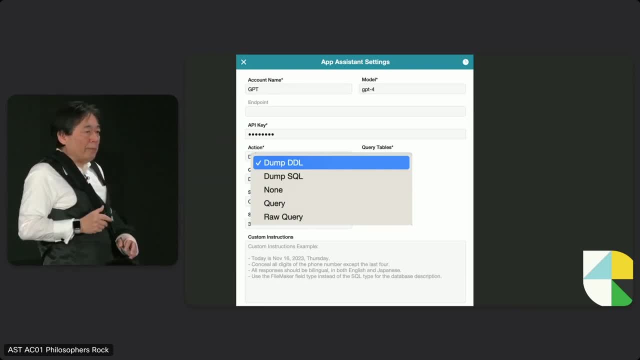 to database engine. Now, if some people make some complicated problem problem, that sometimes could be more than one SQL. So if if there is one SQL you dump SQL, you'll see one. If there are more than one, you will give you all the SQL we have in exercise. 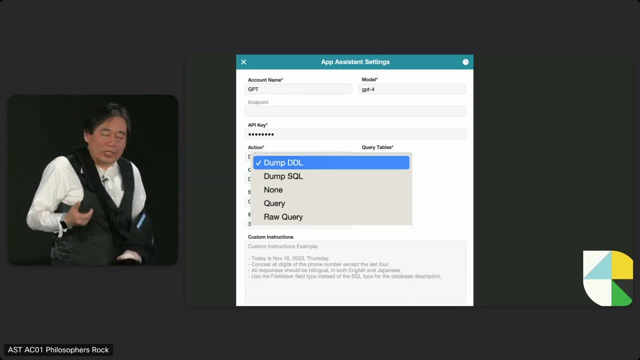 The option now means you don't want. you don't want to do check with the database. You just want to do like, check GTP, like, Or you want to do the RIG, the data. I will show you the check with document. 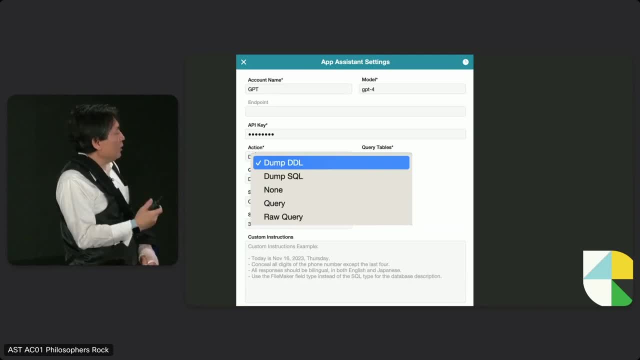 All right. And the next two: one is a query, one, another one is a low query. So the difference of these two- these two are both for check with database. The difference is that the low query primarily just give you the results directly from Draco database engine. 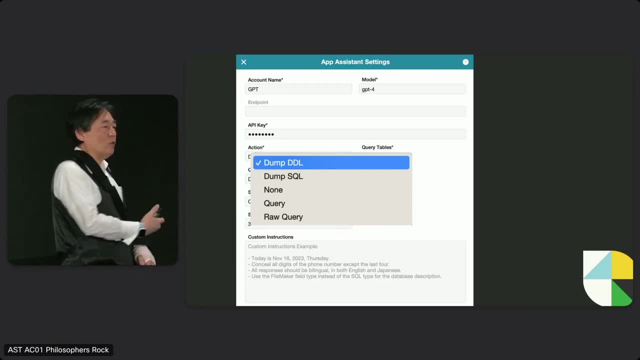 Yeah, And clearly we are sending that result to LLM to format it with natural language. Yeah, So that's up to you which one you want. Yeah, The scope: have two options Now. one is the database only, the other one is no limit. 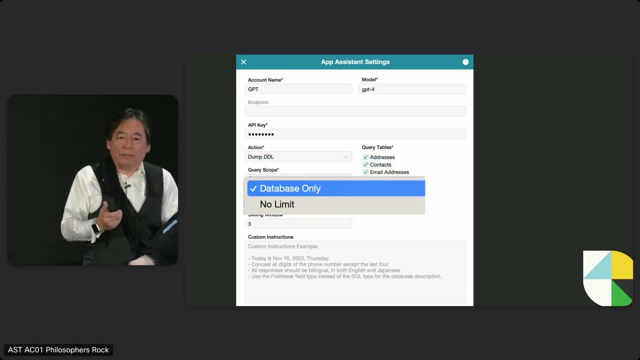 So, as we all know, the LLM is powerful. However, LLM has a tendency of hallucination. So if you design a solution you don't like hallucination, You want limit your user only to the database. the check with database. 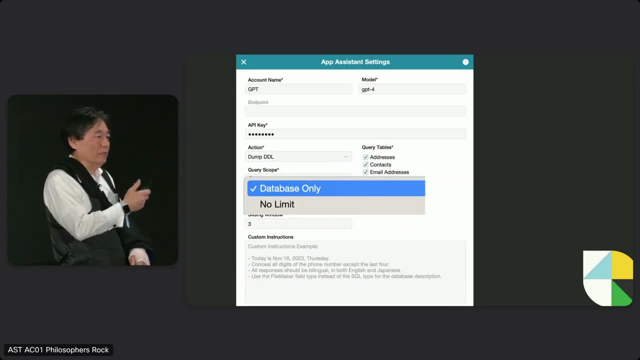 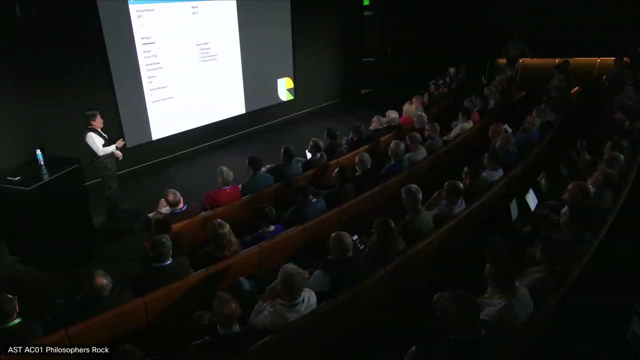 You can pick the database only. Yeah, so we try to cut it out. So in the hallucination stream mode have two modes: on or off. So if you pick on, it will send the data output continuously to the UI, So instead of the user waiting there. 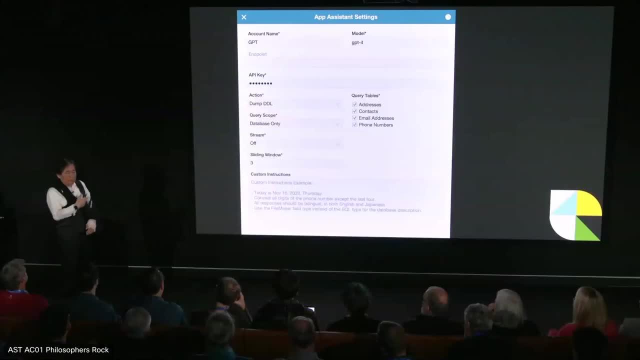 because sometimes the LLM take long time to process. So if you use the stream mode off, the user sometimes will see the beach ball keep running there 30 minutes. one minute, Yeah. so in general speaking, the stream mode on if you expect the long output. it's more user friendly. 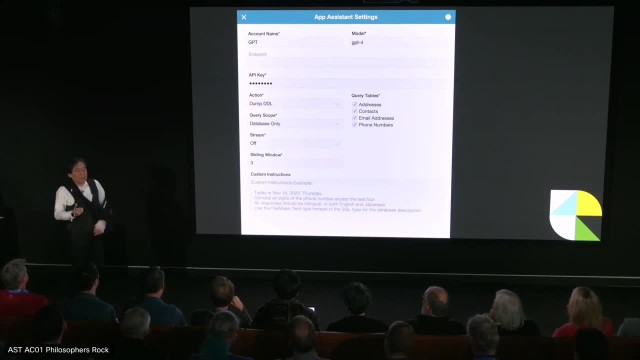 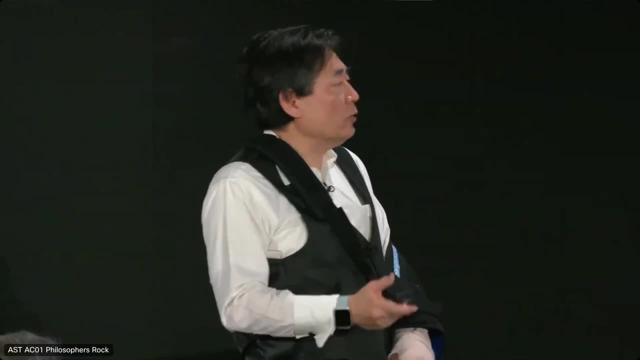 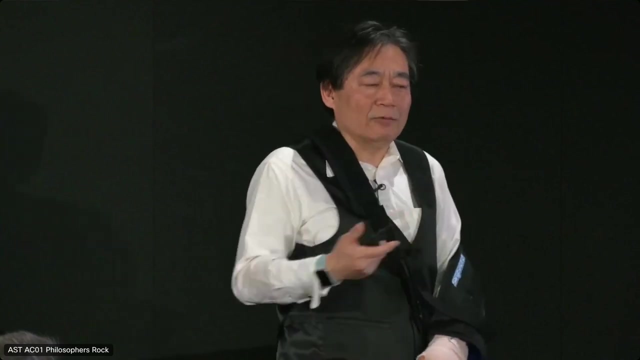 Sliding window three means it will send the three prior prompt and completion pair besides the current prompt. So that's the way to let it keep a context And I think that some of you might ask me a question: say why you pick three. 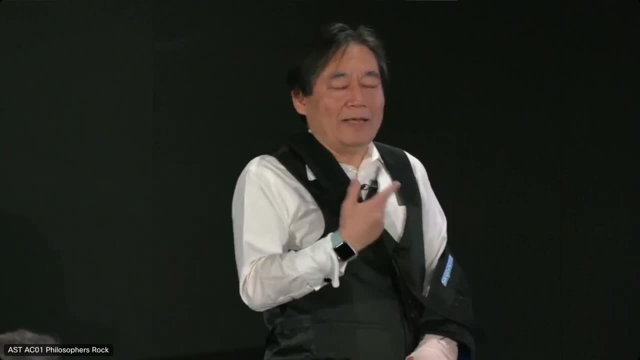 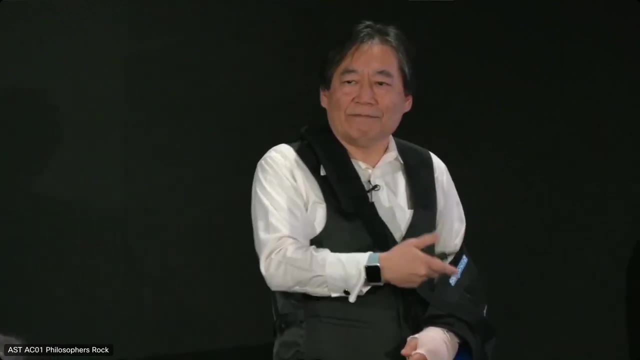 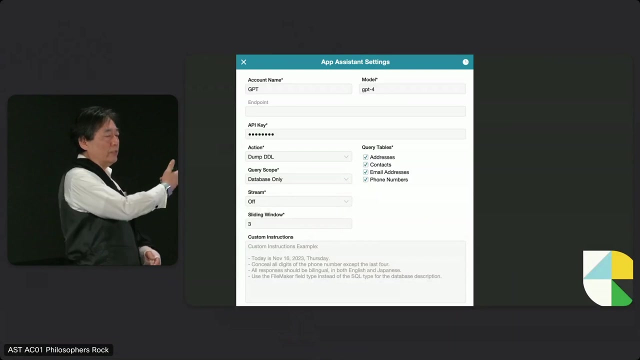 Yeah, what's the optimum number? So? So here is: I don't know the optimum number for all solutions, So for now it's just that if you pick, maybe that time we can find some suitable optimized solution. And so right now that you pick, one reason is the more you send over. 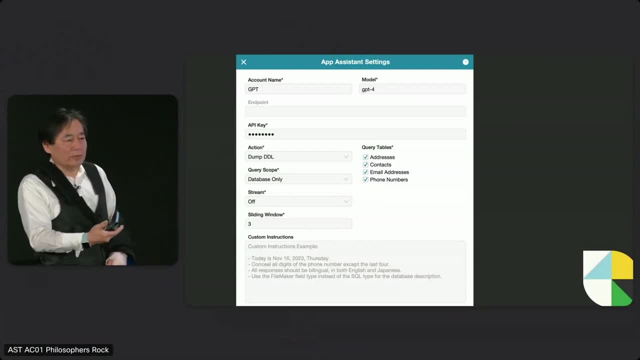 to the LLM. they will charge more based on tokens. And also, the thing is, the more you send over, the process, time is longer, right? So here the demo I show you. basically I use the three And on the left hand side the query table. 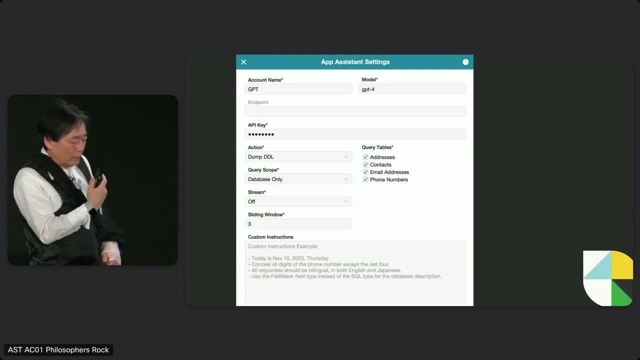 you see, they are for table occurrences. So the database engine we are giving you the list. It check the engine. I find how many table occurrences you have, so we're putting them out here. What you need to do, you just need to. 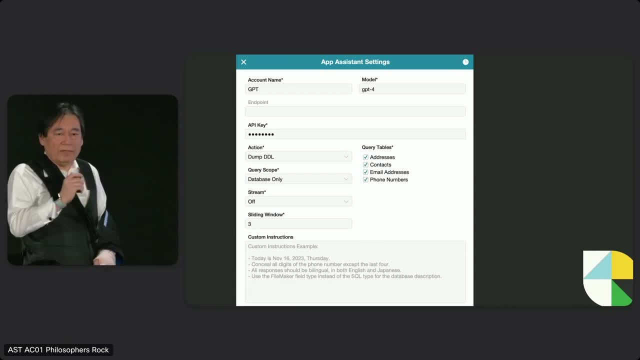 put the checkbox under those you need. I will recommend you only pick. the minima are set. So the reason is The first. again, This is a table. it is a. I assume you use the one near charge, not your own free one. 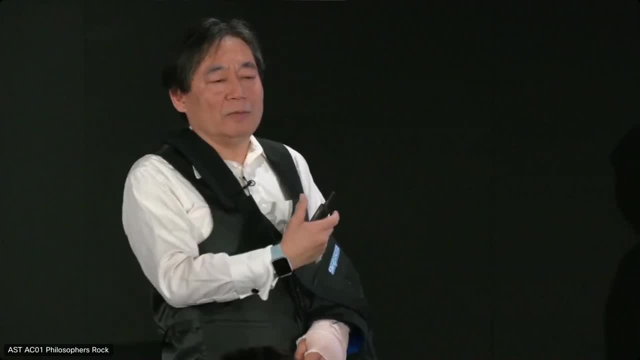 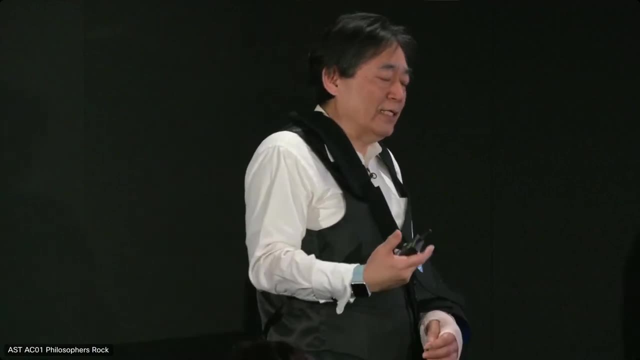 So they charge you by token. The second thing is the more stuff you send over, it take a long time to process And it's not necessary why you want to do that. And another thing, another consideration. some of you- the schema- might have some IP concern. 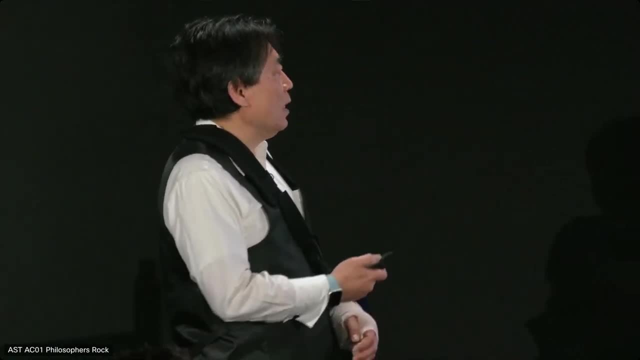 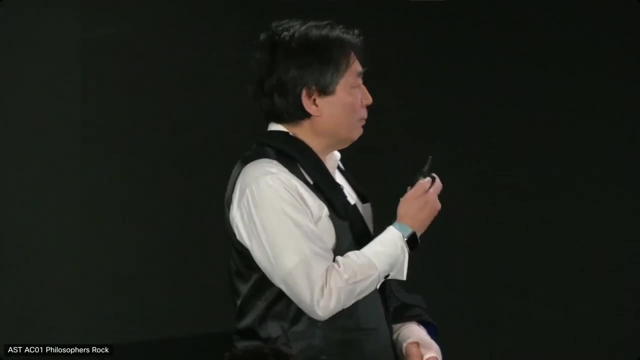 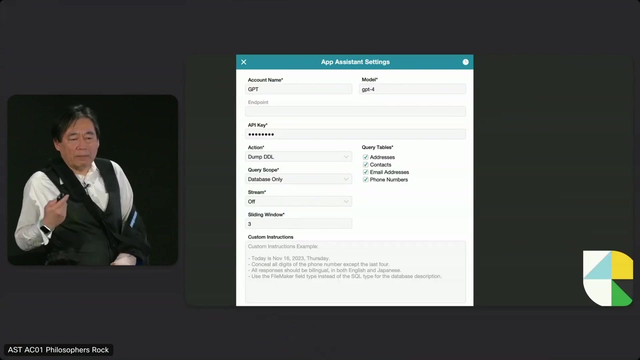 So you don't want to really send it too much, Right, and the custom instruction, you can use it for palm engineering if you need. So you can put actual instruction or put some example. So one shot on the mini shot. So in here the grayout text: 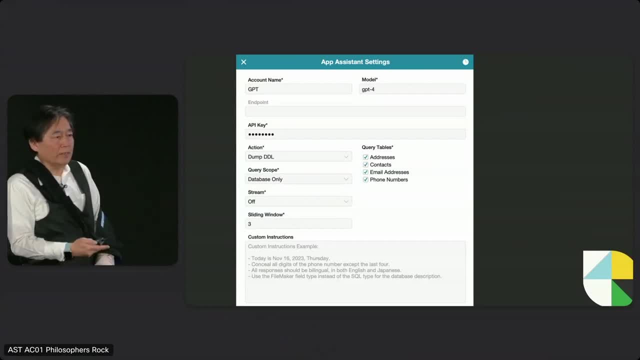 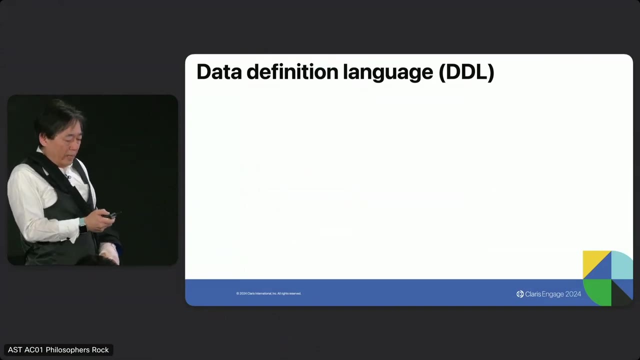 they have some kind of example you can try out And, if you have some extra, actually in the early ETS I saw some people make a very good use of it and have a, So Some great results. Okay, so now let's talk a little bit about DDL. 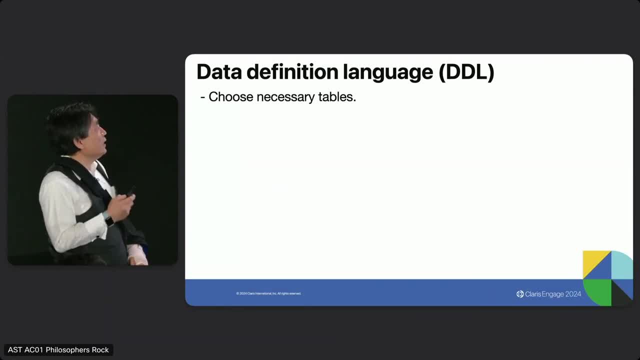 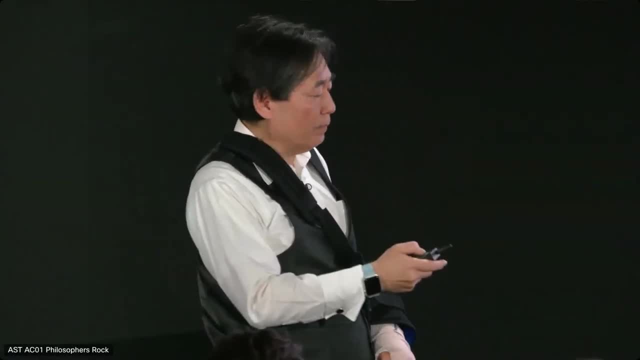 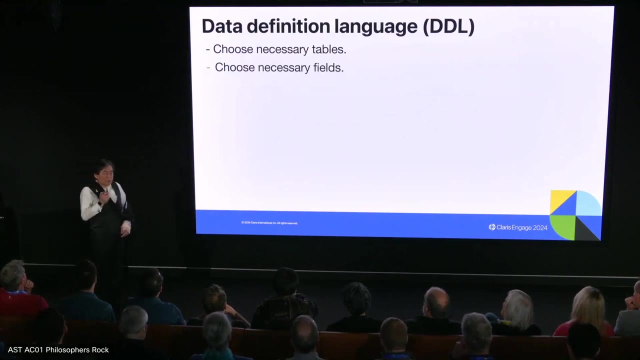 So, first, what you need to change is you need to pick the necessary tables And, just like I put the checkbox over, you pick those you need. And also inside the table, you need to choose the necessary field. Now you have option. 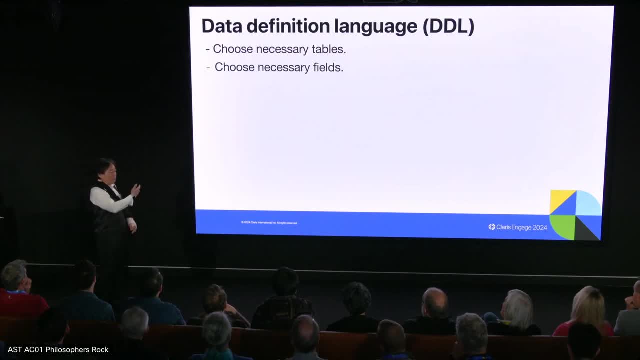 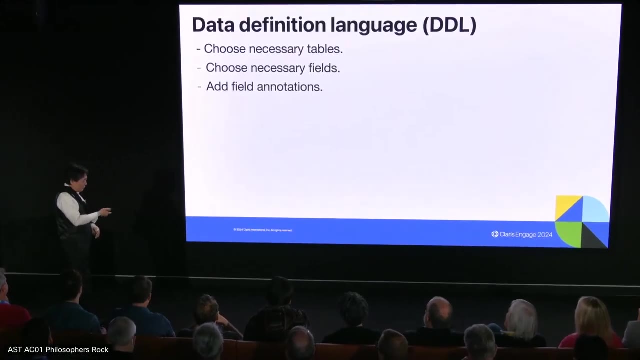 If you don't choose, then the DDL will send all the field of your table Over, And I saw some people's solution. Some tables have more than 100 fields, So that's probably not a good idea to do that. So to choose the necessary field: 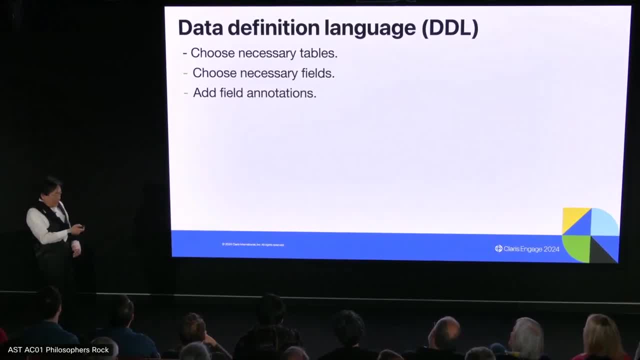 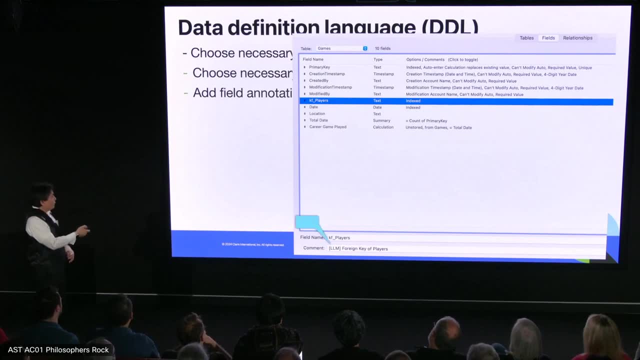 so you can add, go through this field, annotation. Let me show you the screenshot. So here is a screenshot from the Manage Database. So I have this KF underscore player. So in the common field KF underscore player, I put this bracket: LLM bracket tag. 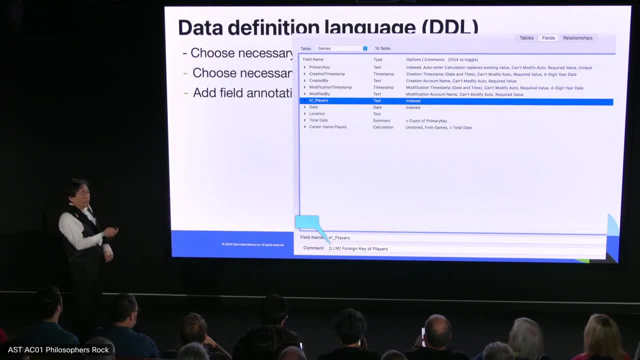 To let DDL understand, I want to include this field into the DDL for this table. So once you add one, the DDL will just follow your instruction. So if you put only one, it's just one. You put a 10, it will include 10.. 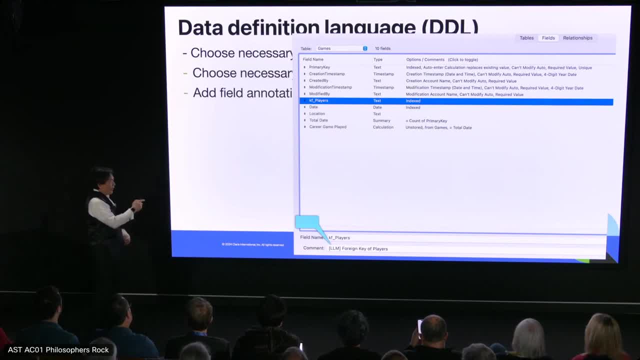 And whatever annotation you put after the bracket LLM bracket, that annotation will send the as a comment along with inside the DDL. So the purpose for that one is to let LLM understand what you mean for this field, the minima schema. 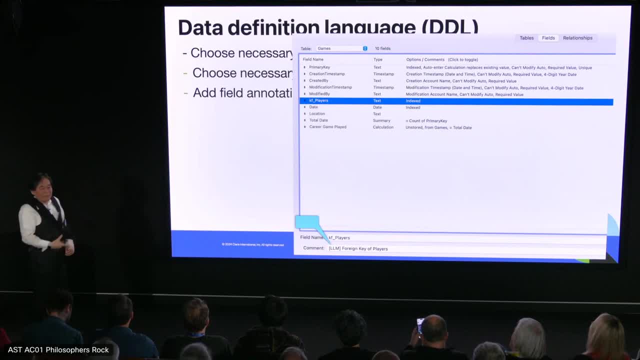 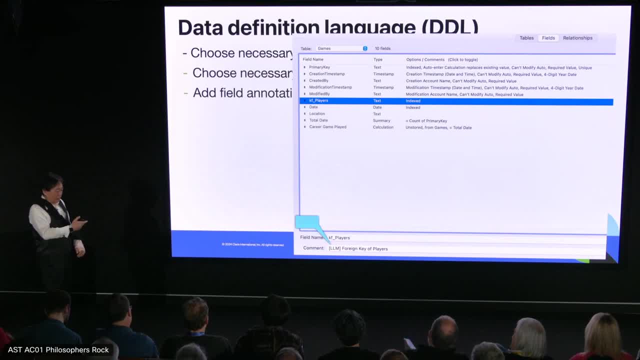 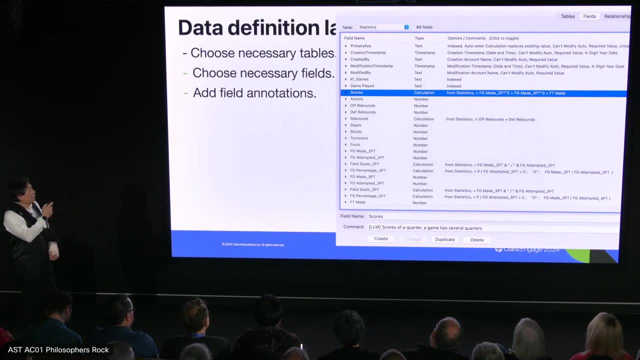 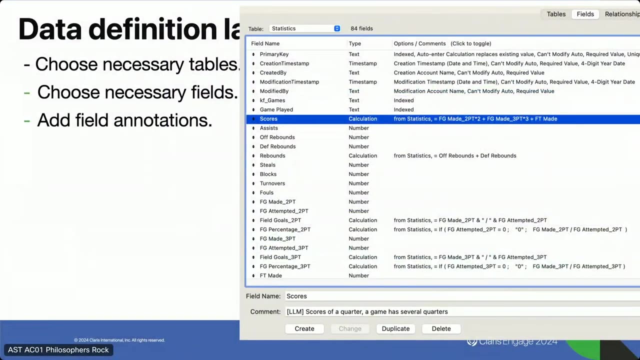 good annotation there. The LLM help LLM make correct decision. So let me show you another example. In here I have a calculation field score. This score basically calculate to the best basketball score of a quarter. so you can see the calculation is sum up. 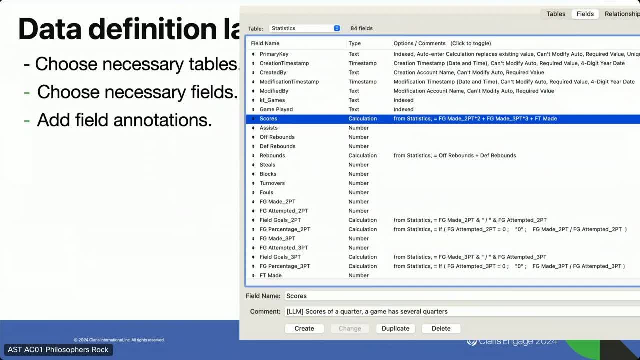 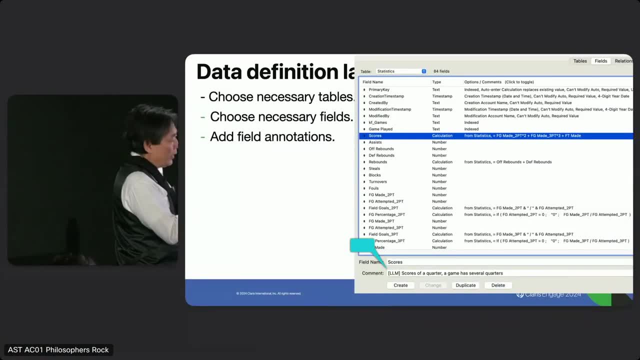 all the three pointers, two pointer and three throws So you can including calculation. So you can fill the for DDL And the same. I put the bracket LLM bracket there And I put annotation scores of a quarter. 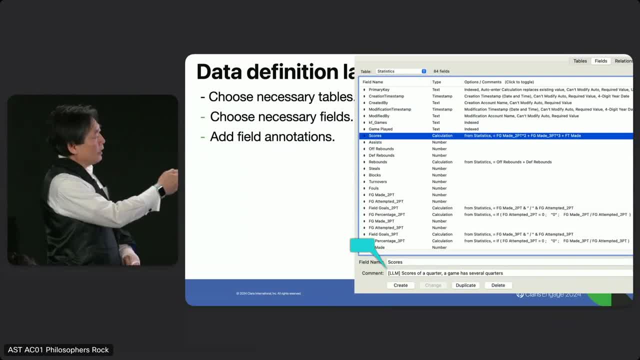 And a game has several quarters. So that's very important here to let LLM know that. So, because this is one-to-many relationship, particularly in this solution, A game sometimes has three quarters, sometimes four quarters, sometimes six quarters. 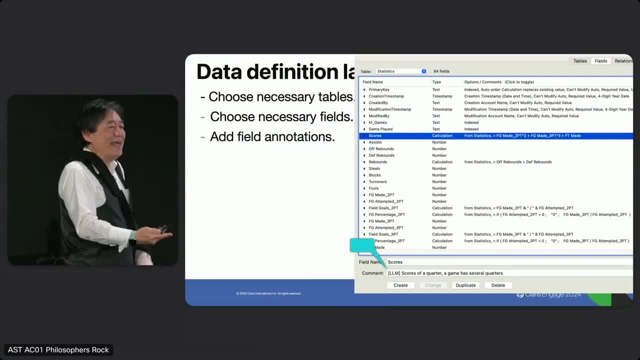 Don't ask me questions, Don't ask me why. That's not a bad thing, But, however, once you put this annotation there and send it to LLM, LLM can generate correct aggregation SQL statement, and regardless of how many quarters. 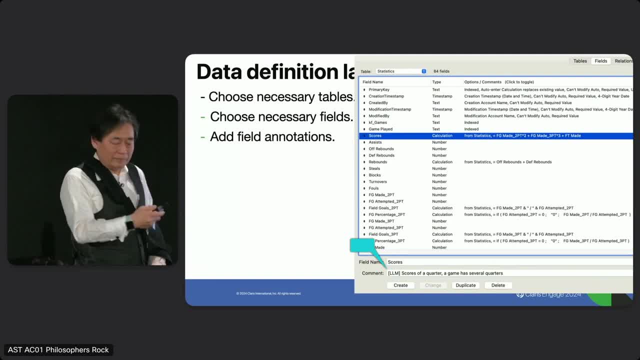 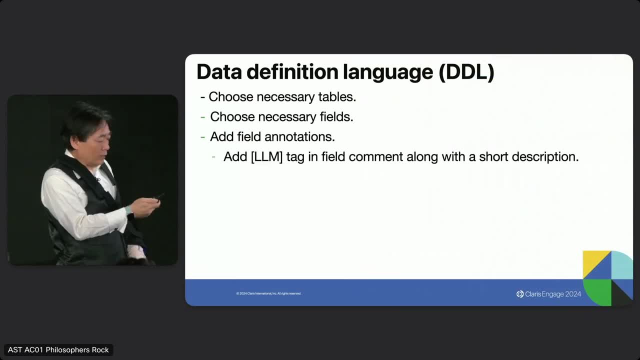 you have for your game, it will give you a correct result. Okay, so here are some tips for the to have a good, good LLM for DDL. So first add the bracket LLM bracket tag in the field comment. 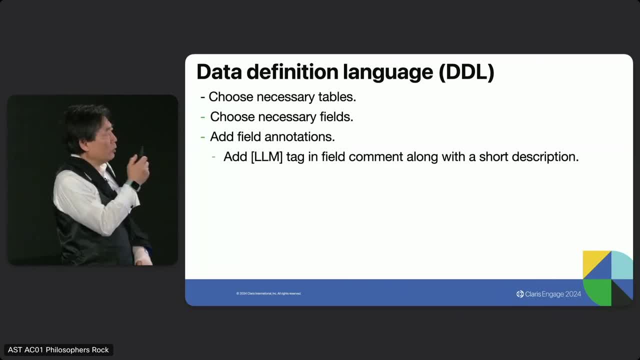 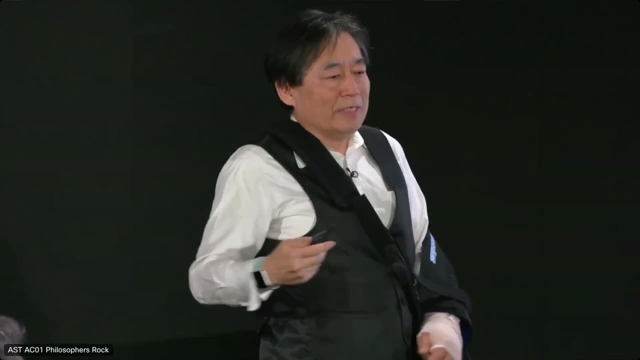 along with a short description, And this short description actually is for LLM to understand the meaning of your field and the schema of your field. So if you don't do this, that might still work, but the thing is that I remember. 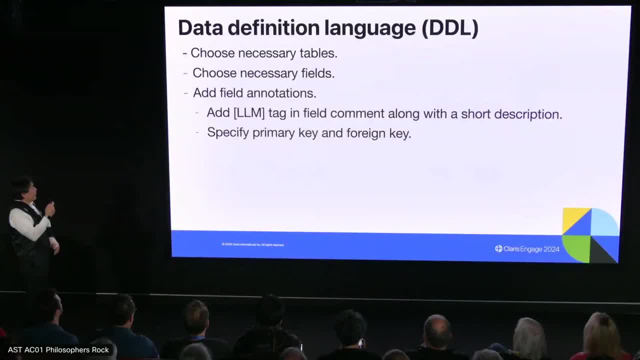 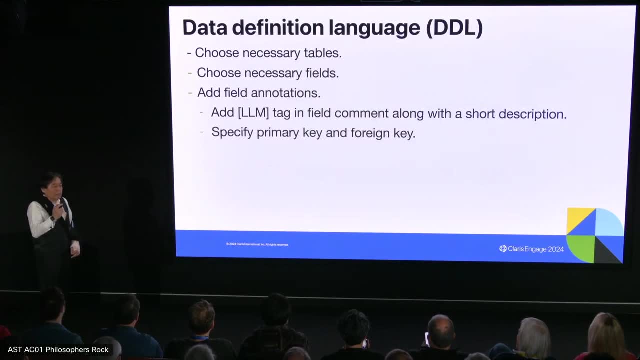 it will send all your field for a table over. And the second one is specify primary key and the foreign key. So this is for the relationship. So if you get, if you run your solution to check with database and you find out, you have relationship. 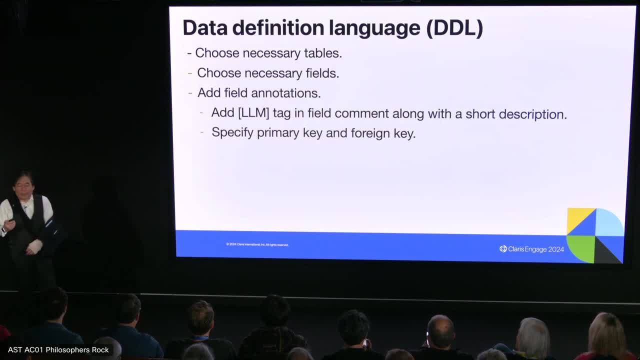 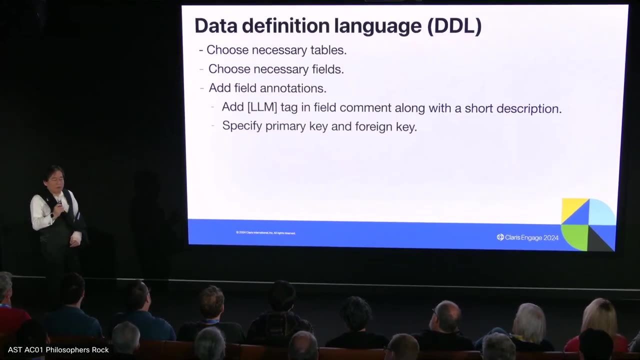 and you find out, the result is incorrect. and when you dump the SQL you see a lot of nested SQLs, potentially because this one done special right. So when the especially like a GPT, when we test it if you're not sure about the primary key. 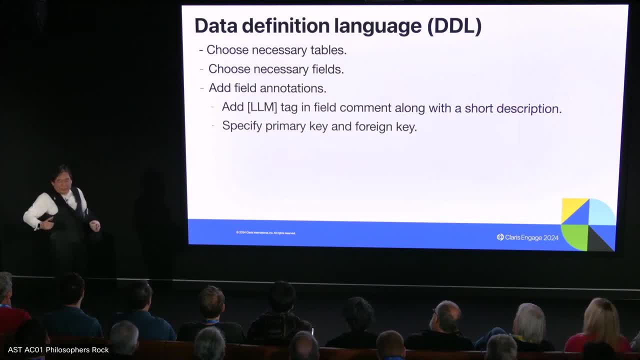 foreign key relationship, it has a tendency to generate nested SQL. So nested SQL, sometimes you still get correct results, but on the other hand, as you know, the nested SQL is more expensive than joined SQL. in general And describe the relationship one-to-one or one-to-many. 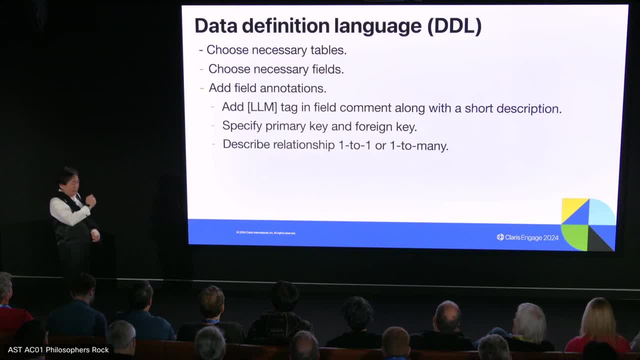 Technically speaking, one-to-one is the default one. you don't need to specify that unless, say, in the schema. it could be confusing And if you have one-to-many relationship, please specify that. Now the example I showed you before. 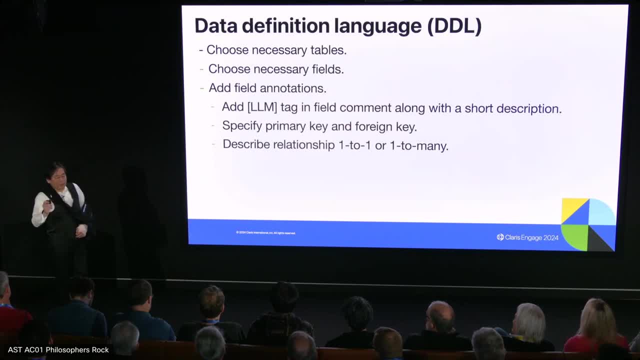 I specify one-to-many in the scores field. Now you can specify that in the foreign key as well. If you specify foreign key it basically the LLM will understand for this chart table actually one-to-many Again have the multiple quarters. 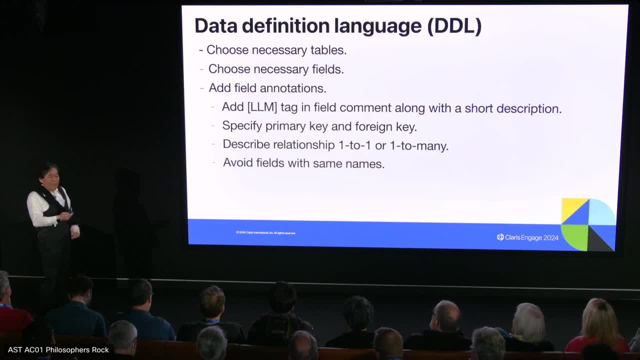 And avoid field name fields with the same name, The name for different table for the one DTL. Think about this. if you say you have schema like a lot that's also confusing to a human being. I can see that when you're in discussion in a meeting, right? 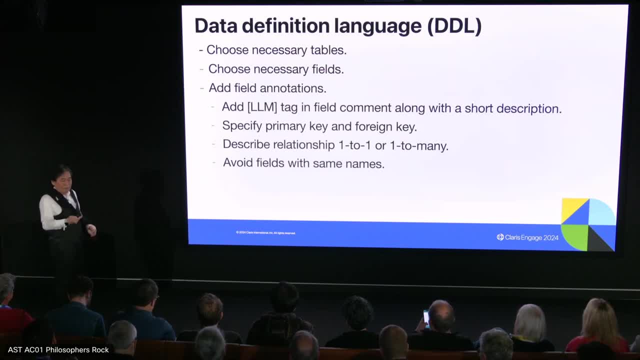 There are several tables have the same field name. then when people asking about here then which one, which one, So the same thing, that if you do have a lot, the LLM potentially can become confused. And this all valid item for field with a value list associated. 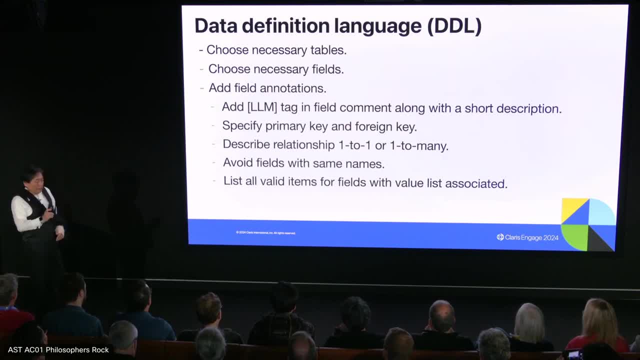 So if you have very specific value list item for a particular field and if you can list that in the annotation, that will really help in LLM to make a good decision to generate correct SQL statement for the user's prompt And don't include the summary field. 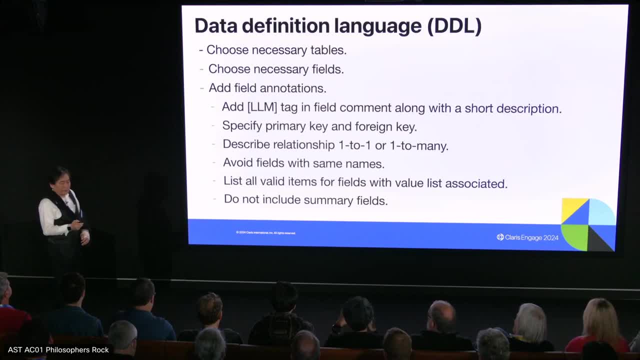 Now, as you know, the five-acre summary field. working on functions All right and LLM. very difficult if it's not impossible to figure out which funcet for your summary field. On the other hand, if you specify clearly the following key: 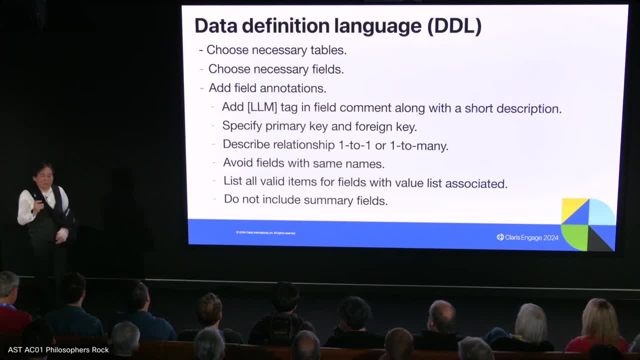 basically parent-child relationship, and you specify the one to one, one to many. clearly, In most of cases the LLM will be able to generate good aggregation function for you to get it the same kind of summary you need. So another thing is to use a check database with LLM. 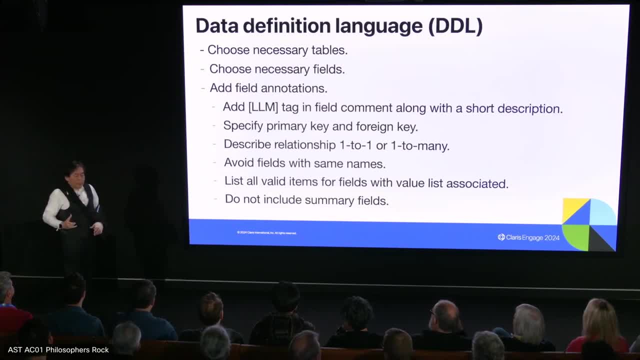 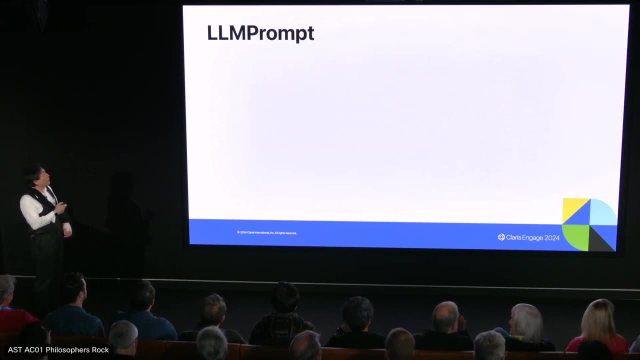 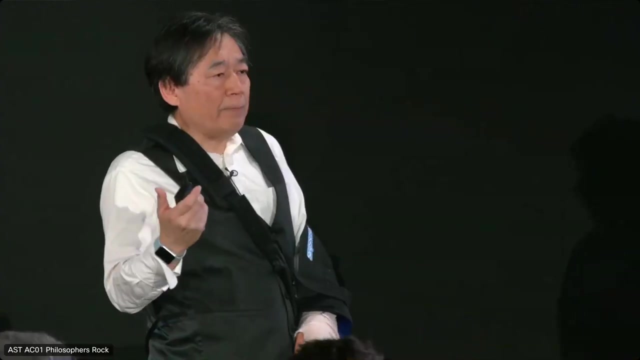 In general speaking, if your database schema is normalized, that works better with LLM. Okay. so now let's take a look at the LLM prompt script step. So this script step is the primary one to check with database. The APA system basically called this script step to perform it. 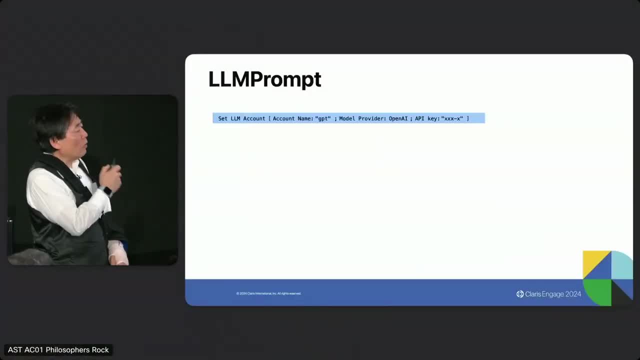 And to use the LLM prompt you need to call set LLM account script, step first. So the example I give here is: I have a set LLM account. The first parameter is account name, just like an app assistant- And second parameter, specified provider is open AI. 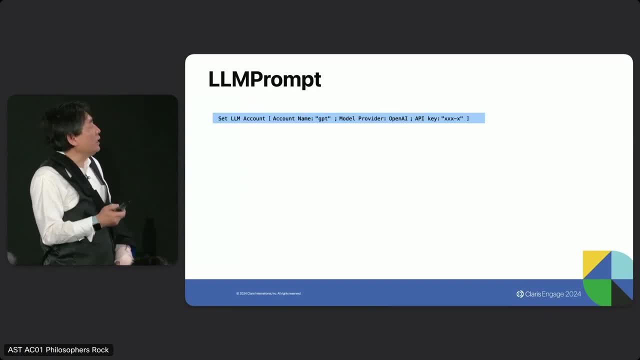 And third parameter, I have my API key. So once you execute this script step, this account information will go into the head of the database, And this is the first step. So once you execute this script step, this account information will go into the head of the database. 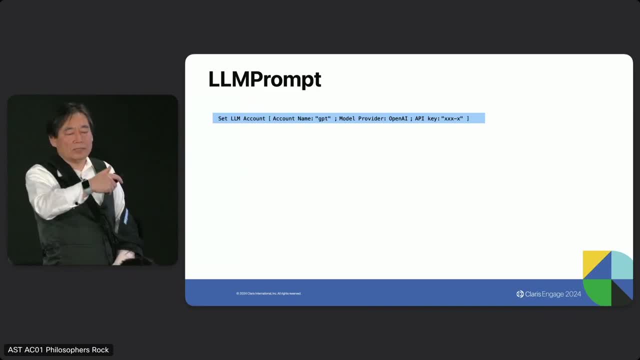 So once you execute this script step, this account information will go into the head of the database. This is the first parameter specified in the dash table of Draco database engine. So you just need to set it once for the lifespan of Draco database And the daytime script step can just refer to the account. 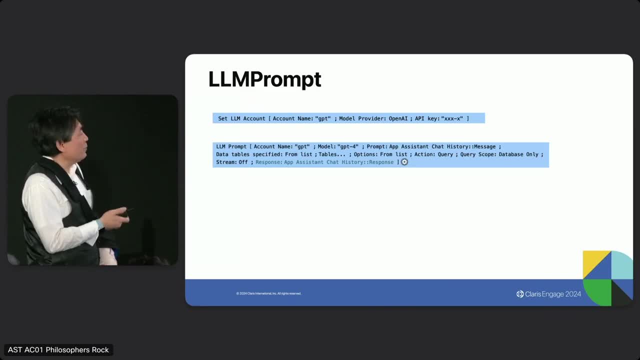 And here is an example of LLM prompt script step. So you can see the first parameter, account point to GPT, which was set before. And second parameter, I specify GPT4.. And third parameter is error is the primary one. that's the content of the prompt. 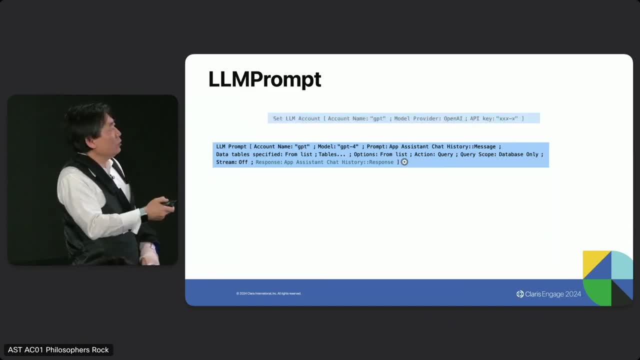 So I get it from a field. And for the content itself, there are two choices. One is you can give a plain text with natural language And another one is you can use a JSON object. So the example I have here, the JSON object. 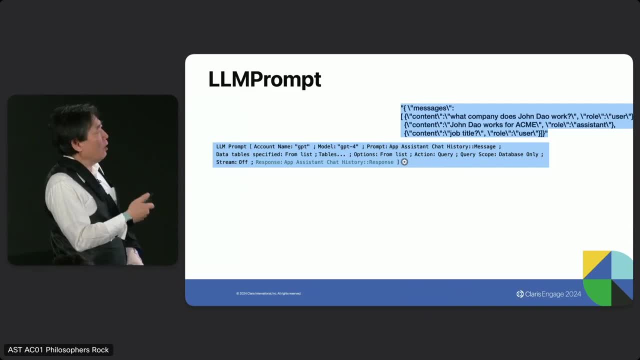 have a key messages And the value is a vector of JSON object. So the first one is the previous prompt, The second one is the previous completion, The third one is the current prompt So you can have a multiple set in there. So remember the sliding window three from the app assistant. 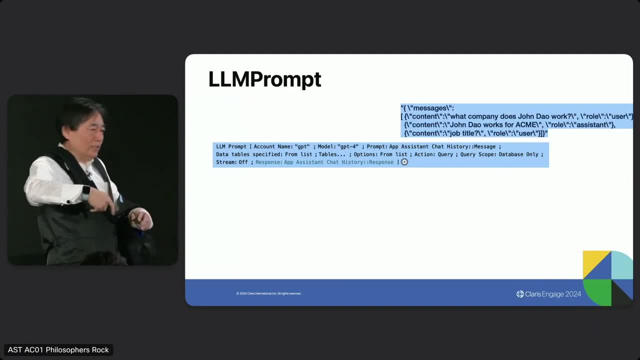 I have three, So if you have more than three shutters before then you will see the three. Previous Previous. Previous. Previous Previous. Most recent prompt and the completion show up in the JSON structure For the data table specified. so this one had three options. 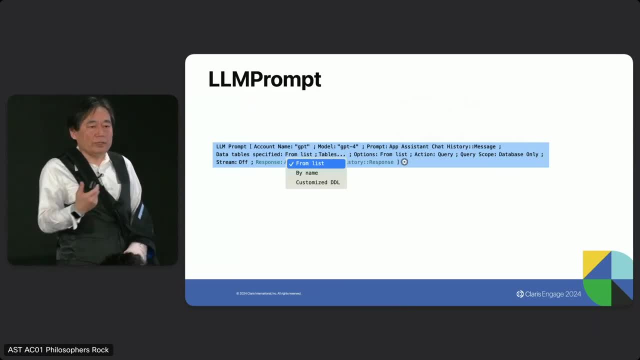 So you specify the table occurrence to be including in a DDL. You can pick from list, Or you can specify by name, Or you can then inject your customer DDL. For example, you use I show you before And then you modify it. 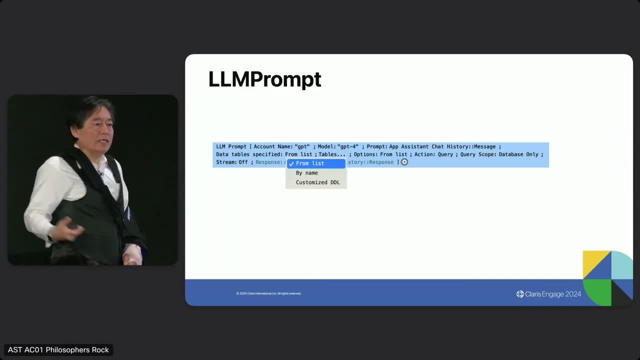 Then you can use the customized DDL to inject it. Instead they generate new one. In case you see some problem, you don't want to go to field annotation to change it regenerate. So you can use a customized DDL. And here is the specified table. 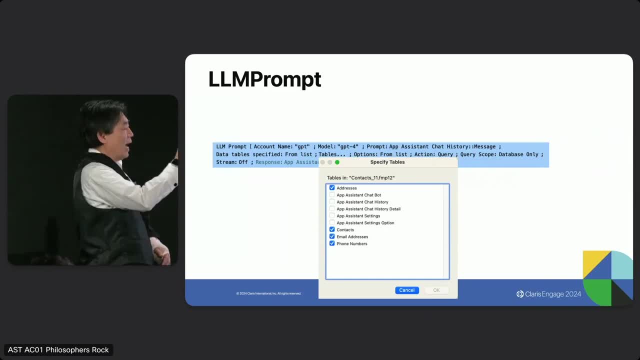 So what you need to do, just like before you put a checkbox on the table, It's a table of currency you need. You might notice there are five more tables in here than the app assistant. That's because the app assistant create five more tables. 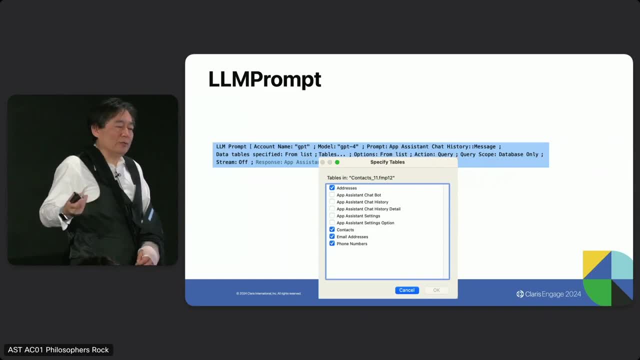 And app's assistant is smart enough, There's no reason to send app assistant scheme to the LLM, So we don't need to waste your money to do that. And the actions: there are five actions, So basically that's the Eglite XM use. 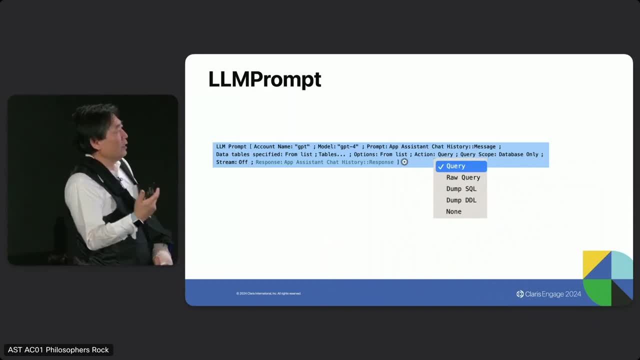 Eglite XM. the exact same five options possible to pick as the app assistant, And QueryScope is the exact same, the database only or non-limited, And StreamMall and also the same Response is where you can store your response. 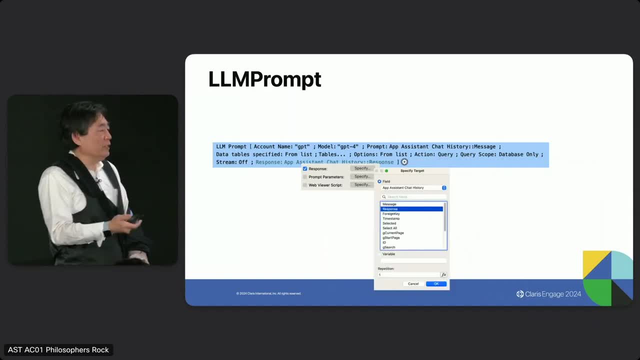 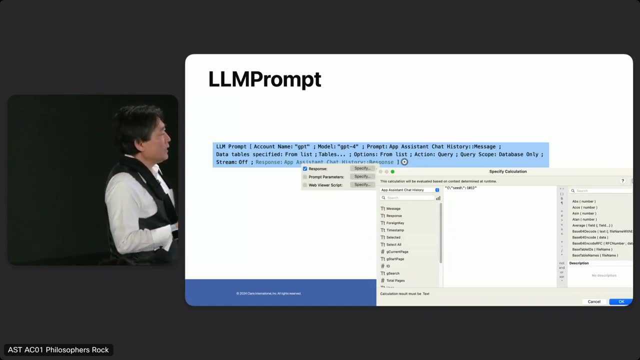 So the response. you can store it in the file maker field or in a variable And problem parameter is option. In this example I set the seed to 101.. The format is a simple JSON format, So I set the seed number to 101.. 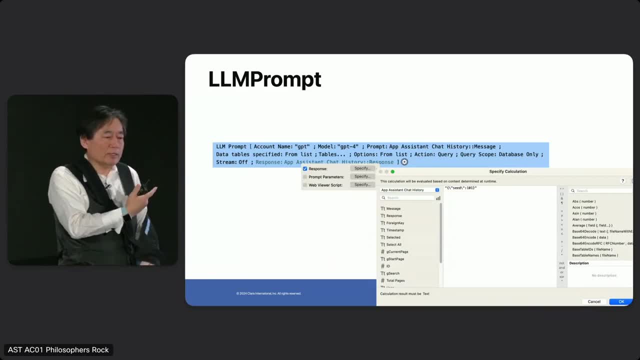 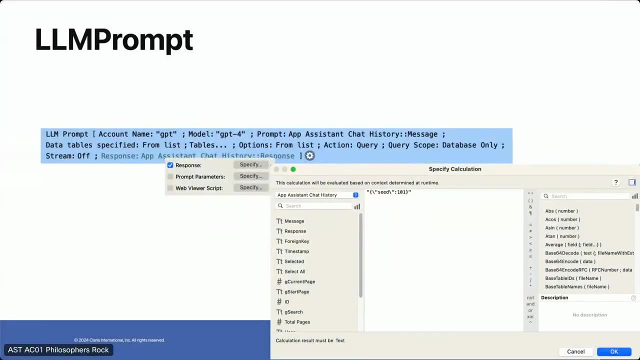 This one for GPT. actually, this is a recent improvement. they made during the December- sorry, during November- last year. So once you set the seed number, you will set the seed of the random number: the generation of GPT. 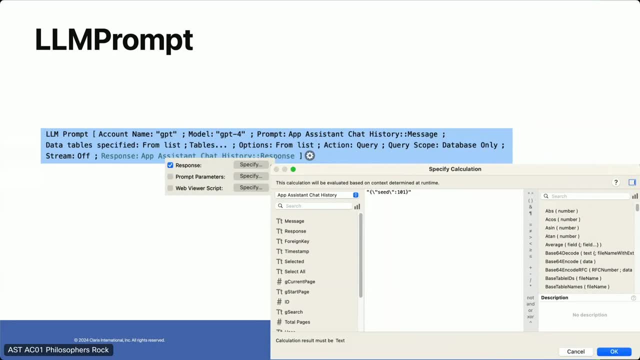 So if you need, sometimes, if your solution, if you wanted the most deterministic results, you can set the seed number to a fixed number And also you can set another parameter called temperature. For GPT the temperature is zero means the most deterministic. 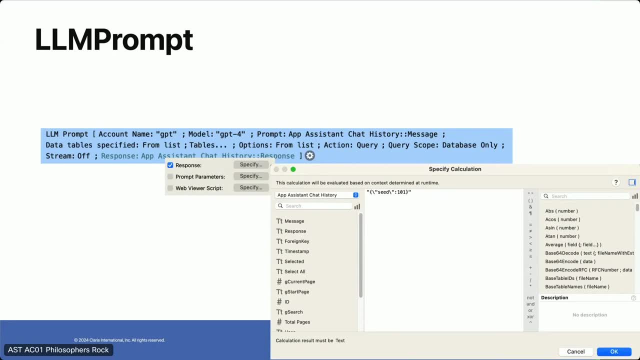 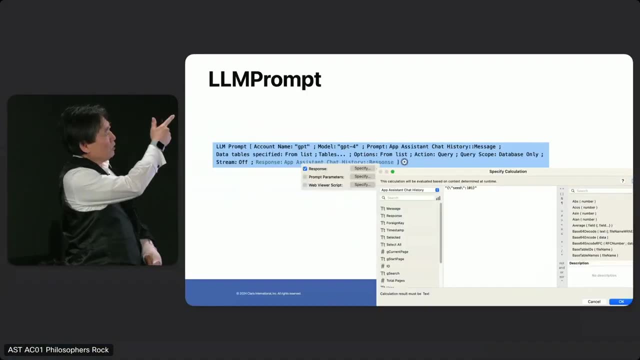 And 1.0 means the most creative And for different LLM. actually there are different definitions, So some of them from minus one to one. So when you use a different LL you need to check their document. But again, this one, the problem parameter is option. 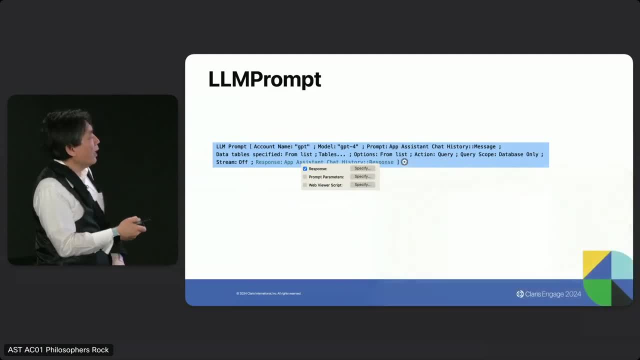 So you don't need to set it. if you don't need, The WebViewer script is also option, So the app assistant basically uses the WebViewer script to communicate with WebViewer, and WebDirect can leverage that as well. So once you kind of set up your solutions. 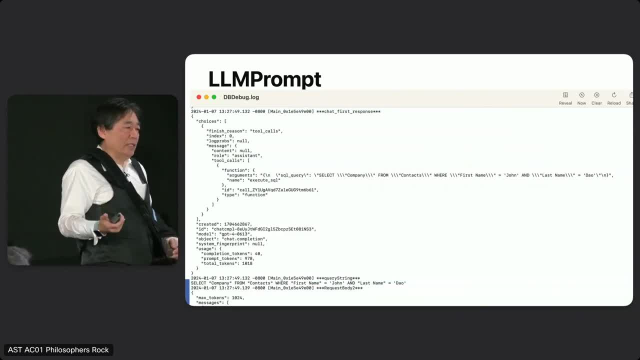 start chatting with database. sometimes you might need to debug- or maybe you're just curious- what's happening between the LLM and the Draco database engine, so we at least debug log mechanism. So here is the screenshot, like I did before, So you can see the sequence statement. 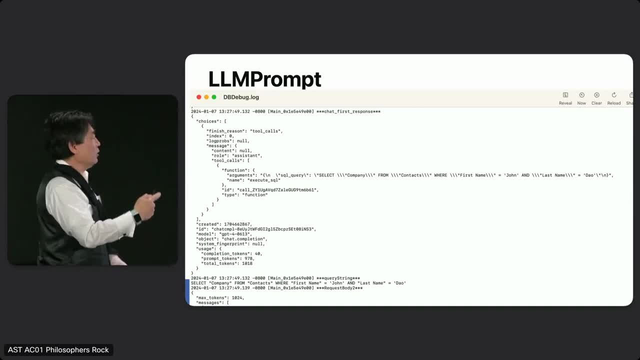 that come in from the LLM to FileMaker Draco Database Engine. We create a new script, step LLM debug log, so you can use that to control when to start, when to turn on, when to turn off, and you also, if you don't like the default name. 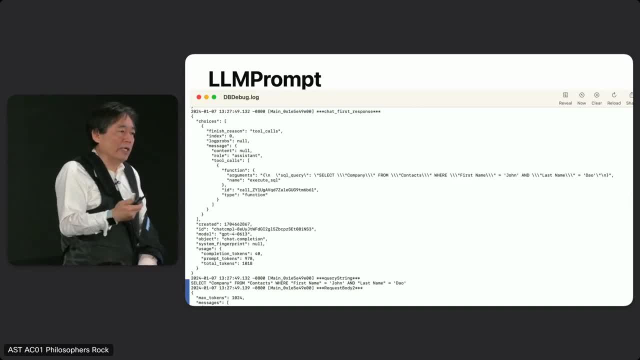 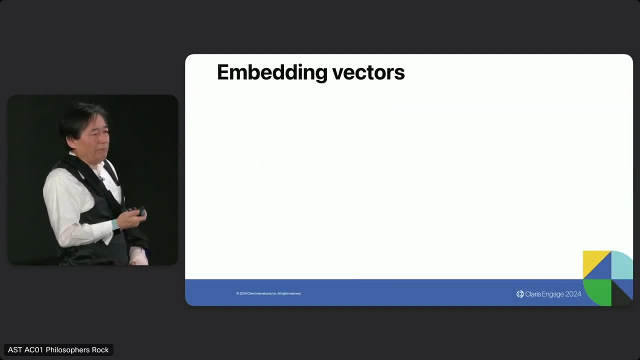 you can save to any different file name you like. You can also set it in a proposable, if you'd like. Okay, so the next topic is embedding vectors. So embedding that vector is a very exciting feature from LLM. So what embedding vector is? 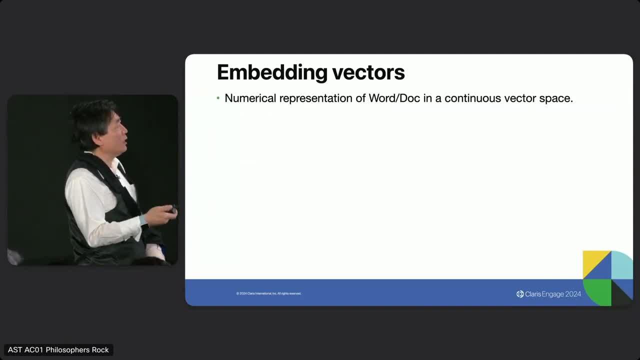 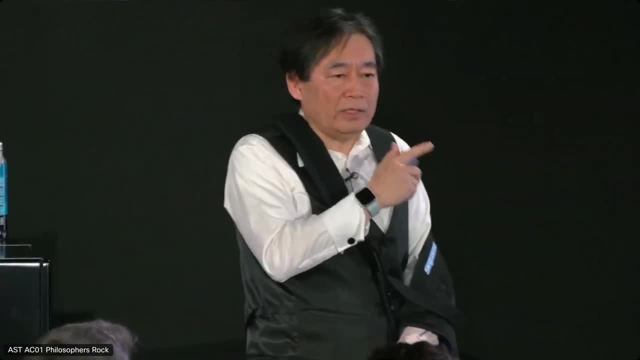 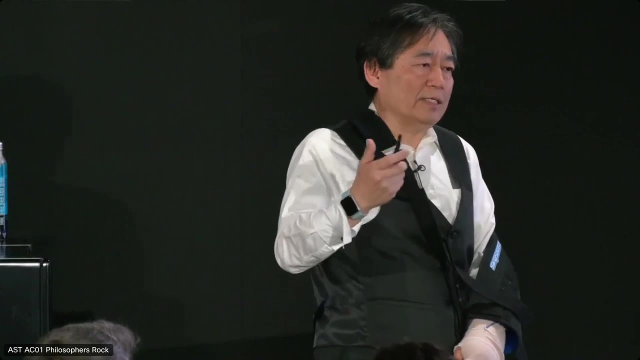 numerical representation of some text or document in a continuous vector space. So this definition, technically speaking, need to update. Majority of LLM actually going to support multiple model. So what that means is that besides the Dutch language model, it can support well some of them already right now. 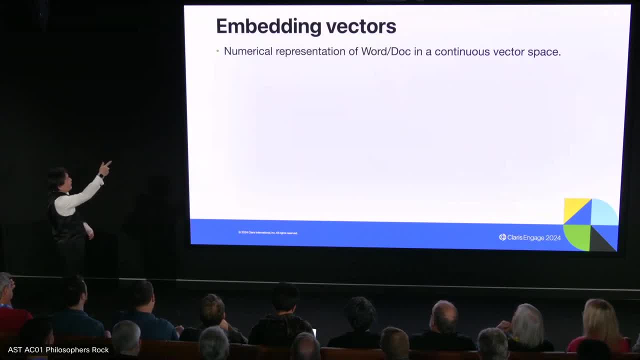 it can support like an image, audio video, So then the numerical representation could be something beyond the text. However, in this section we just stick with this definition, The one I show you. actually, the embedding vector actually means some text. 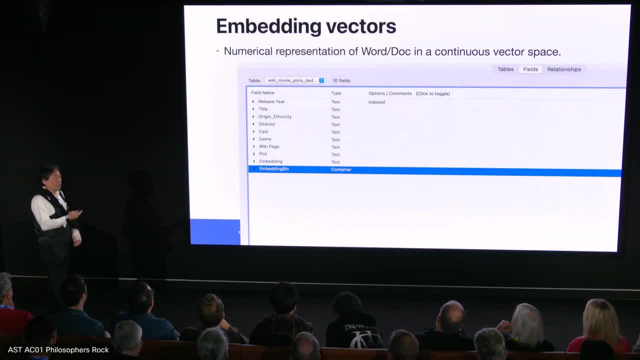 To get the embedding vector into a FileMaker database, you need to create a field to store it. So there are two options. That example I show you here: the binary embedding field. I create it as a simple container. So if that's a container, 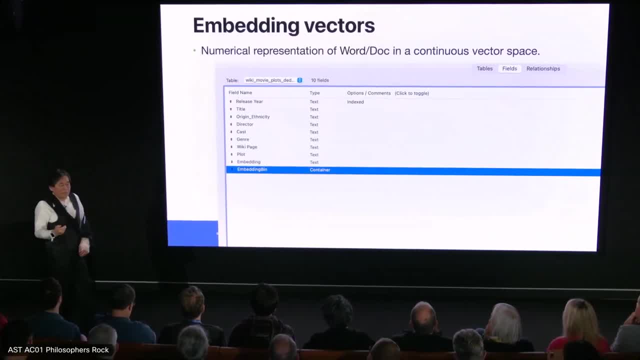 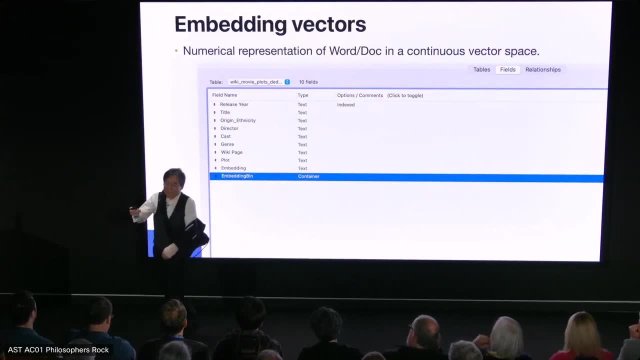 the embedding vector will store in binary format. If you create like the embedding here and create as a text field, the embedding vector store there will be text format. Okay, I highly recommend you use the binary format because the binary format, the processing time is much faster. 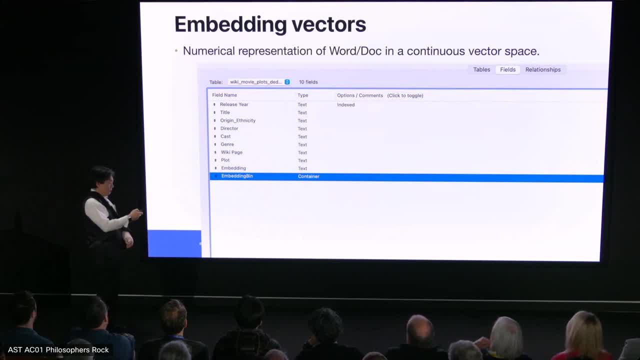 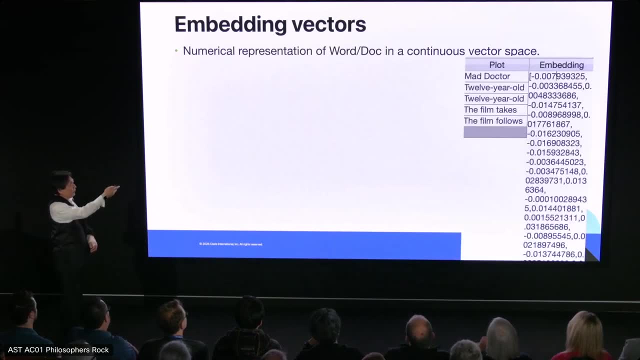 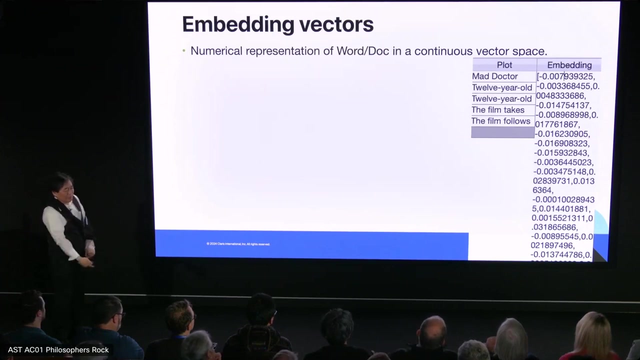 and it costs less in storage. Here is an embedding vector I got from OpenAI before. You see quite a lot of numbers and actually it does have a lot of numbers. So the dimension is 1536, 1536.. So I cannot print all the numbers for you. 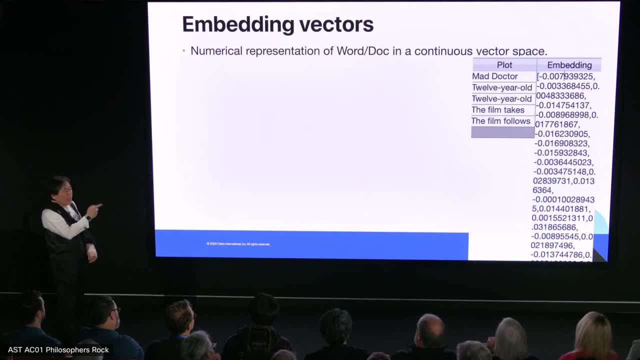 That could be more than 10 pages And for now we store that as a double. So for the particular vector there are 1536 doubles. So we have tried to use the 14 points, but sometimes the calculation seems to lose some precision. 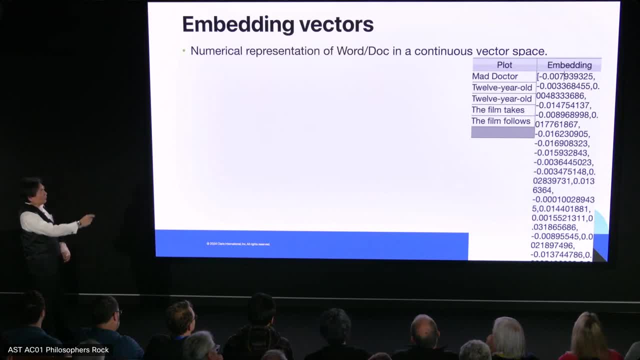 So for now we just cite it to the results. So just use a little bit more storage memory for you And if you notice that you see the numbers are all quite small. You don't see any number bigger than one or smaller than minus one. 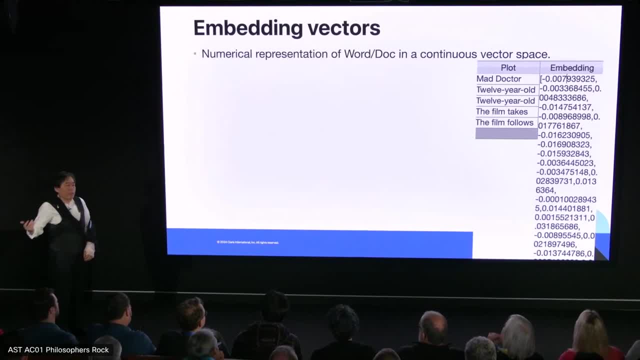 The reason is: from OpenAI, all the embedding vector you get are normalized. A normalized vector simply means the length of the vector is one, So the number basically you cannot. If you see something bigger than one, that means that the embedding vector is not normalized. 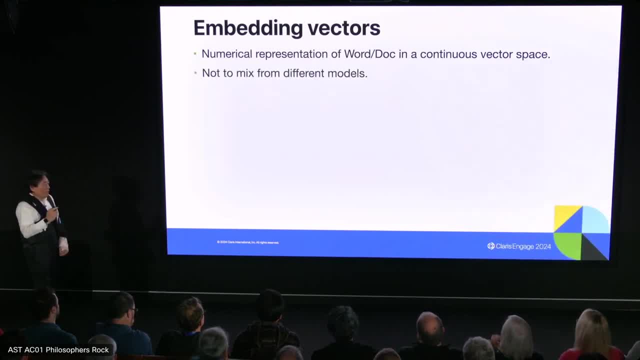 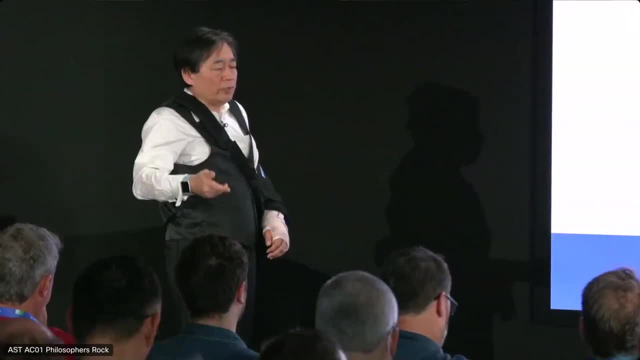 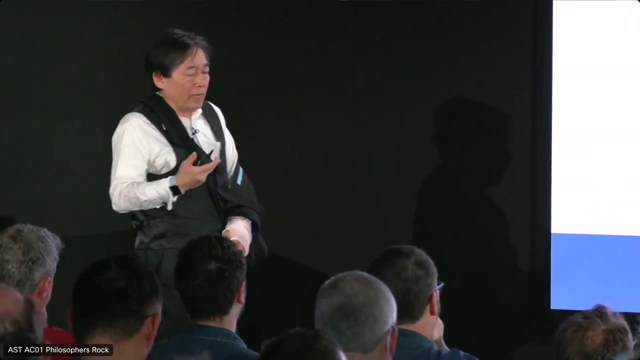 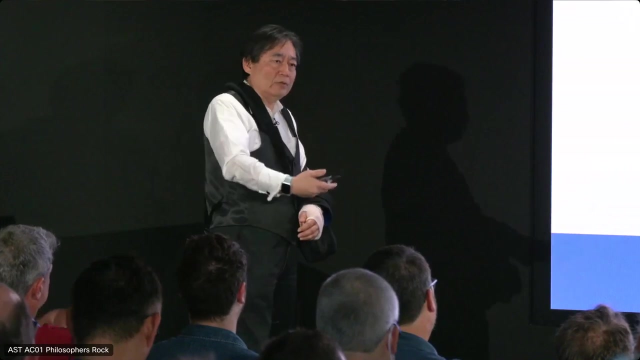 And please pay attention, Don't mix the embedding vector from different models. So Draco database engine allow you to connect to multiple LLM at the same time. But it's fine say you have one table connect to get embedding vector from one LLM and another table to get from another LLM. 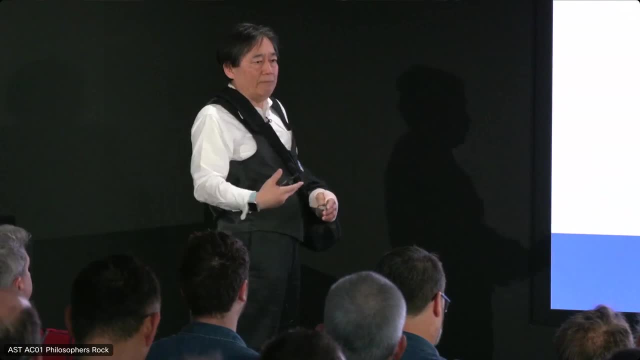 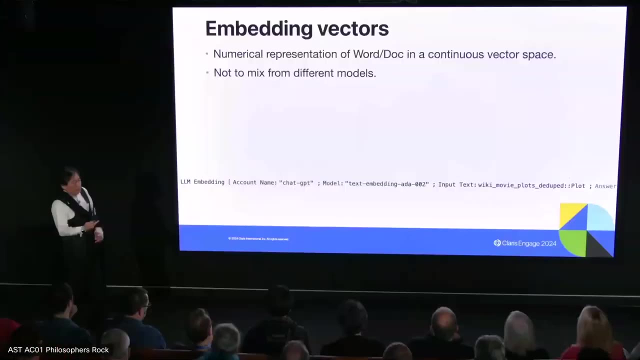 And you do a comparison. But please pay attention, Don't mix them. If you mix them you might get some unexpected result. And here is a quick step you can use to retrieve the embedding vector. So LLM, embedding, first parameter. again, the same is the account. 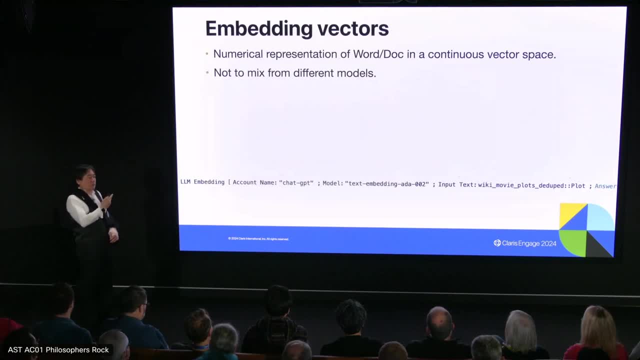 Second parameter, model. You need to specify model to get embedding vector. Please pay attention: Here I use the text embedding 8.002.. So even you talk to OpenAI, you don't get embedding vector from GPT-3, GPT-4.. 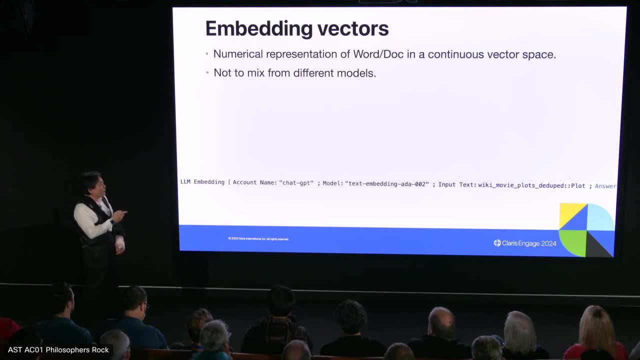 It's a text embedding 8.002.. And the third parameter, input text, is where your natural language text you want to generate embedding vector. And the last one, the answer is where you want to store your embedding vector So you can store in a field or in a variable. 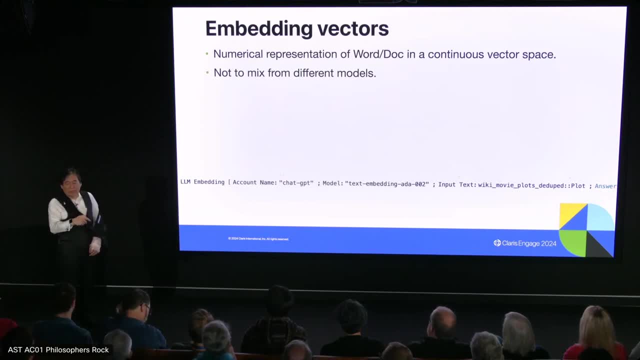 If you store a field- it's a container field- the embedding vector will be in binary format. If a text field, that will be text format. And if you specify a variable, the variable 1 will be text format And correspondingly we have another. 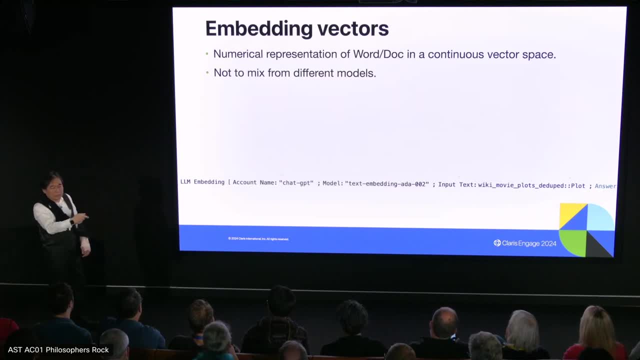 we have a calculation function to get embedding vector. So if you use the calculation function to get, by default we return a binary format for you because binary format is faster. Okay, so basically, you use the split step or a calc function: get embedding vector. 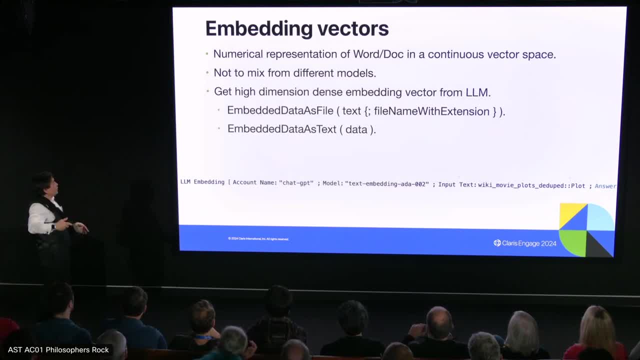 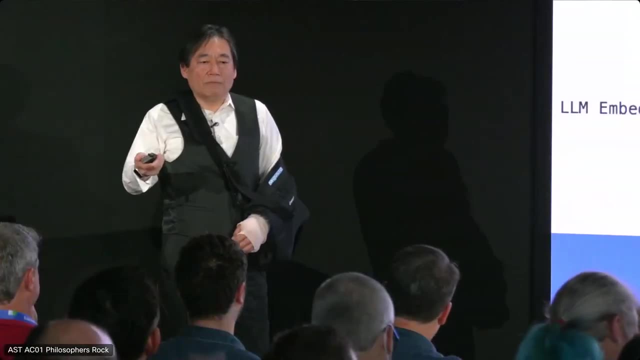 What is a 1536,? it's definitely high dimension, intense, And because we support two formats, so we provide the two calc functions to help you convert between these two formats. For example, if you want to export, then you probably want to export with text format. 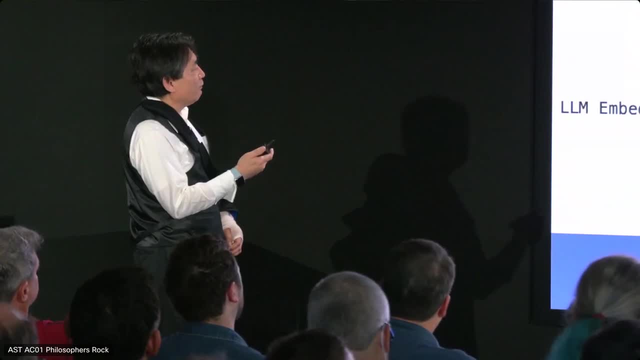 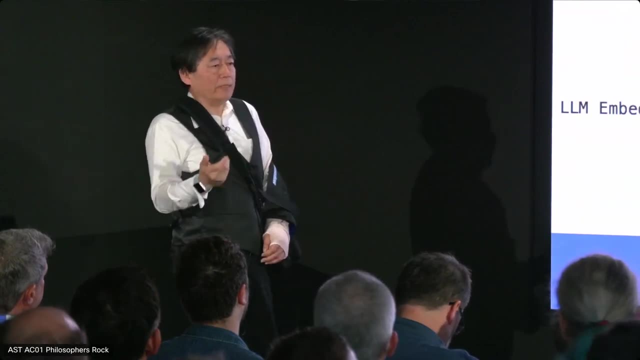 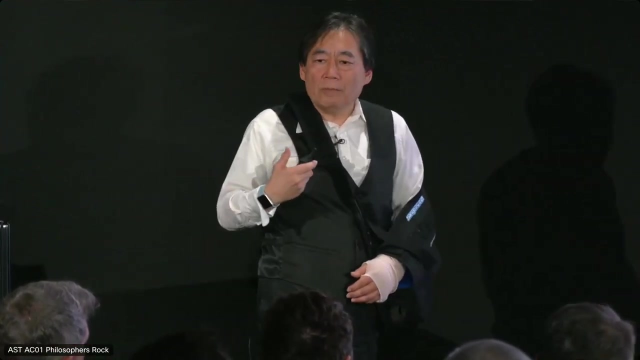 So then embedding data as file will convert text format into binary format. Embedded data text will compare from binary format to a text format And assume you need to get embedding vector for the table. So we provide another script step to help you to say: 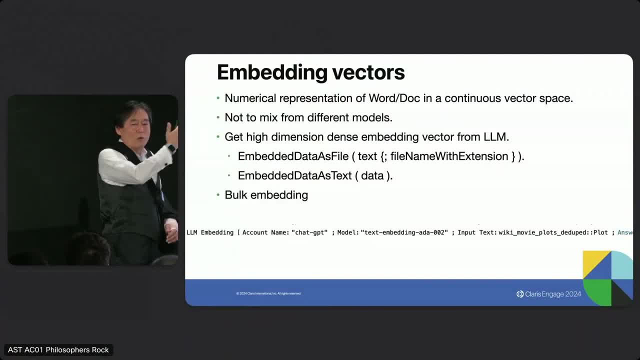 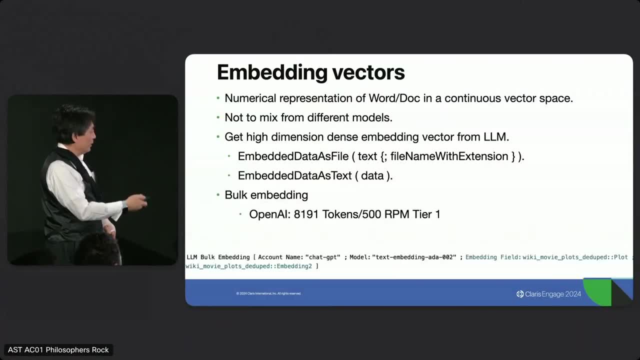 use one script step and we'll get the whole table for you. So the syntax is very similar to the LL embedding vector. So LL and bulk embedding. the parameters are very similar, But the difference is this one: we use dispatch queue multi-thread. 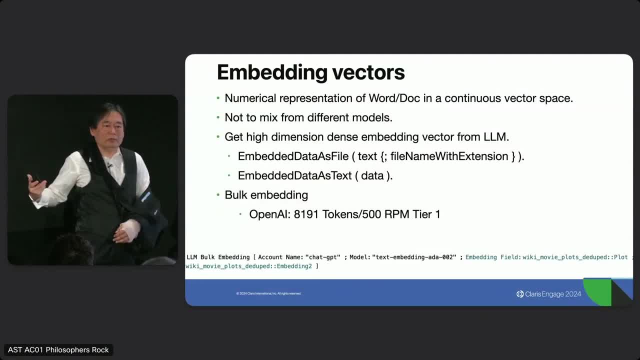 and try to get the embedding vector for all records in your table as soon as possible. However, most LL providers have throttling mechanism. For example, OpenAI have 81, 91 token limit and for tier one account have 500 RPM limit. 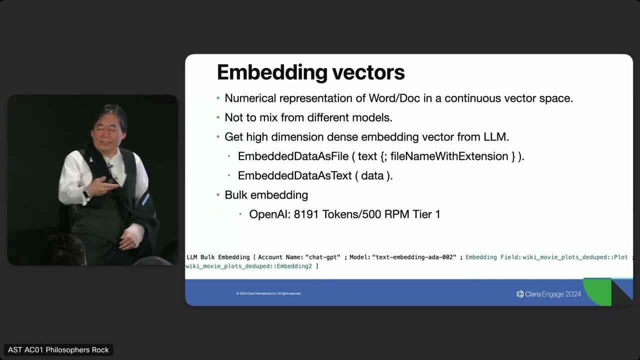 But you don't need to worry about that. If we encounter this kind of rate limited, token limited, we'll try to back off, slow down a little bit, But still try to get all your embedding vector with one script step, unless you encounter some photo error. 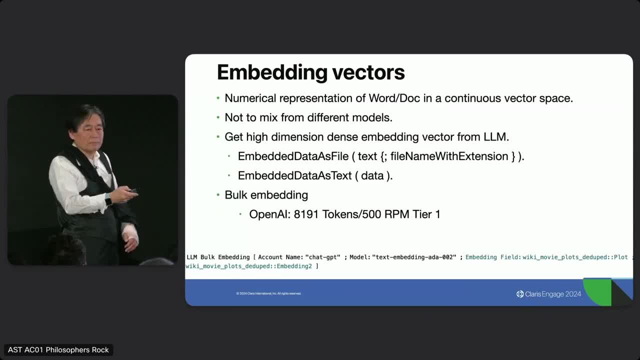 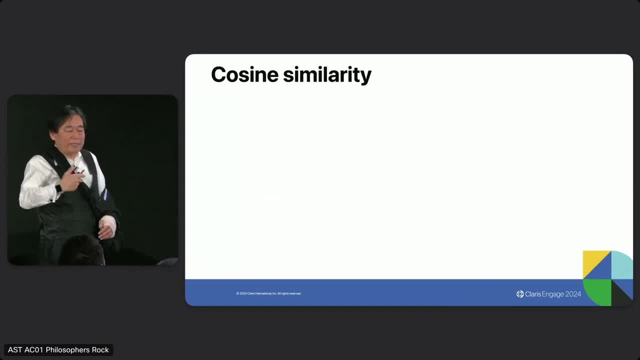 Otherwise you will try to finish it in one shot. Okay, so the next topic is the cosine similarity. Since right now you have an embedding vector in your database, then you can try to process it, And then you can. a lot of times you want to make your. 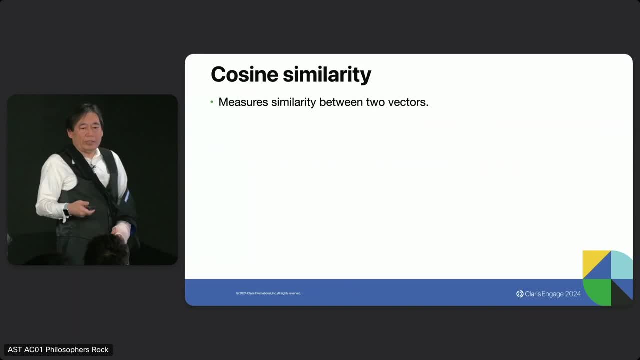 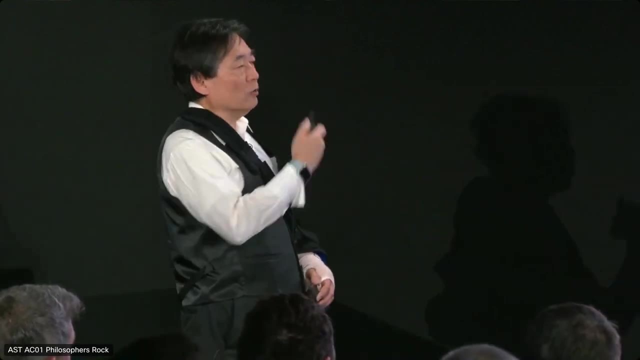 similarity between two vectors. So cosine similarity is the most popular algorithm to do that right now. So there are several different ones, For example the Manhattan distance, the Cartesian distance, So and we implement the calculation function for you, Just call cosine similarity to compare two vectors. 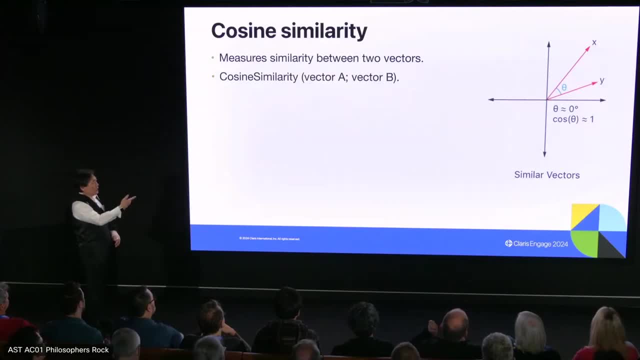 And I make some illustration here in two dimensions. I apologize, I'm not able to draw a 1536 dimension for you, So I will just use just like you learn in high school. So for similar vectors, theta is close to zero. 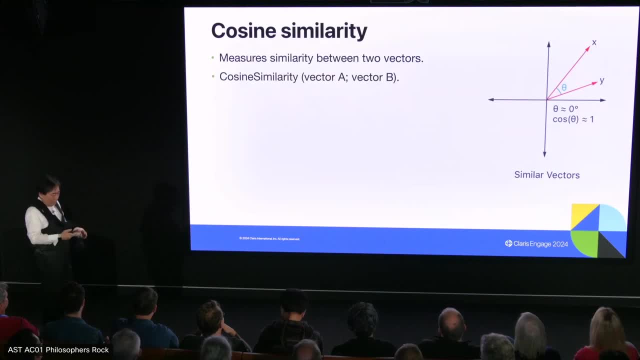 The cosine similarity will close to one. That means they are very similar or could be identical. And for orthogonal vectors- theta close to 90 degrees. The cosine similarity will be close to zero. For opposite vectors- theta close to 180 degrees. 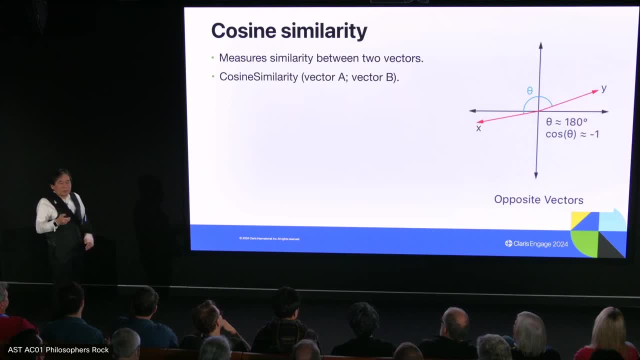 The cosine similarity will be close to minus one. So simply put, the gentleman range for cosine similarity you expect from the calc function is between minus one and one inclusively, And we made a decision for you. The only normalized vectors that store in the five megadatabase: 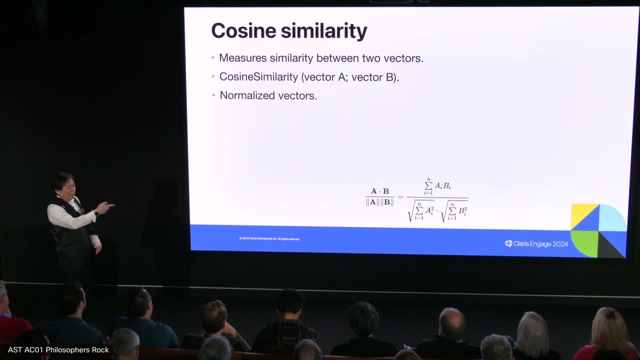 And let me explain why we make this decision: The scientific evidence of this. So if you don't not familiar with the math formula, don't worry, I'm not going to give you a quiz, but I just want to explain. 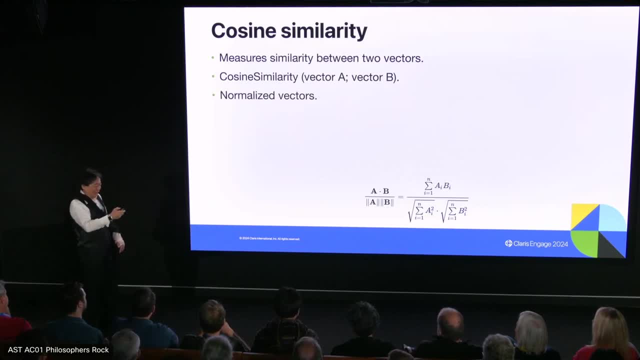 Why we make that decision for you. If you disagree, feel free to Yeah, yeah, yeah, So for the denominator, you see the denominator and then you have to see the summation i from 1 to n and it sum up the a sub i square. 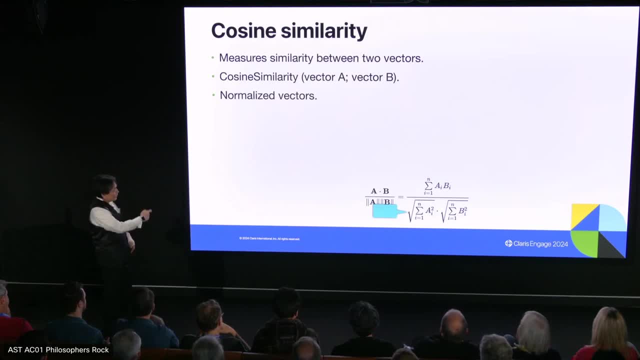 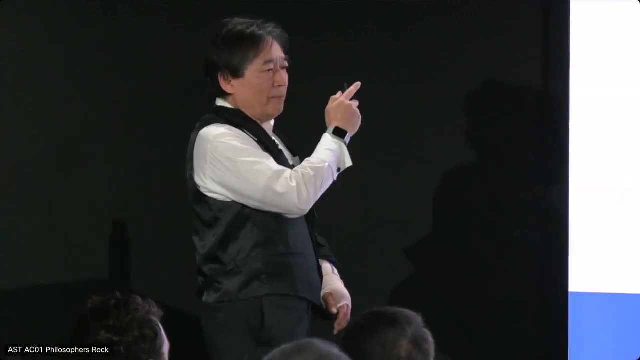 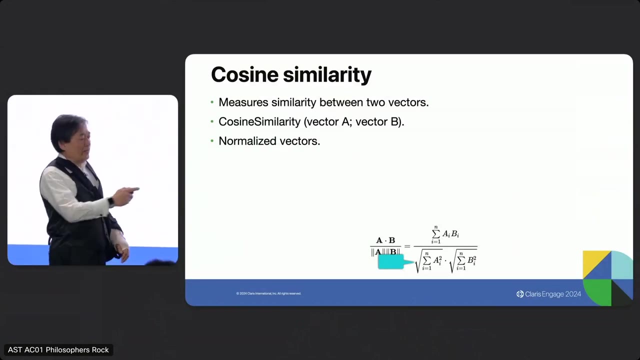 and then make a square root of it. So what it does, this complex calculation, is to calculate the length of vector a, And if the vector a is the normalized vector, then after all this calculation, the result is one And the same thing for vector b. 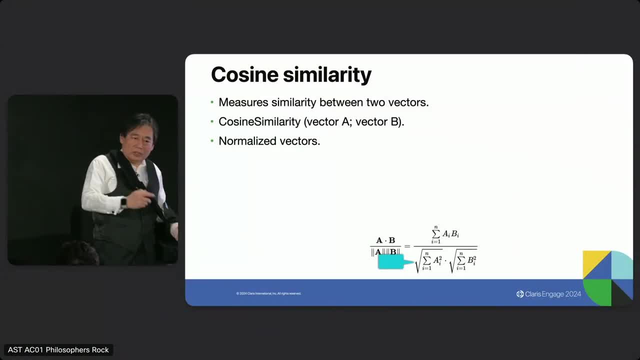 And remember I told you that open AI all return normalized vector and majority of LLM provider give you normalized vector. So why I need to waste your computer power and energy to do this calculation? the value I already know And one times one, then divide it. 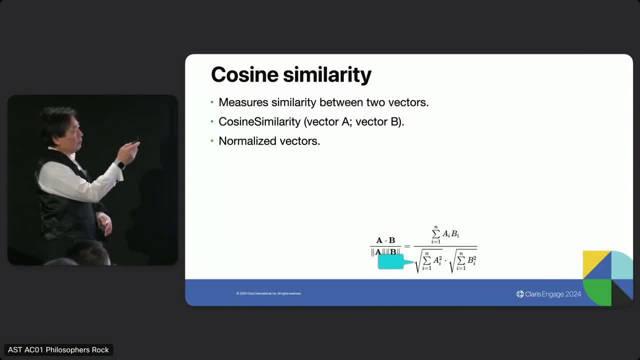 So we can save that. So just calculate the top part of the a sub i times b sub i and sum it up from i equal to 1 to n. Mathematically, this one is the top part of the a sub i times b sub i. 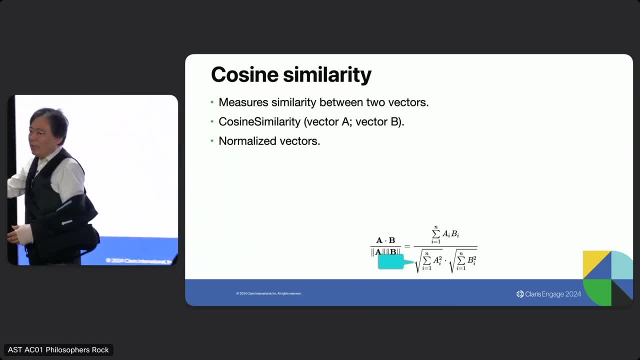 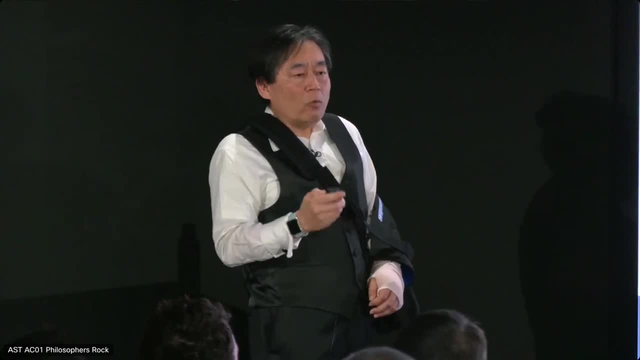 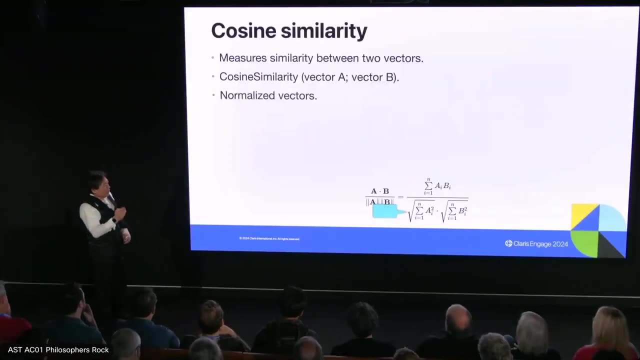 And this is the so-called dot product or dot score. So there are another one like a cross product, But cosine similarity, need a dot product. But think about that. Even that one, the full open AI case, just a simple cosine similarity between two vectors. 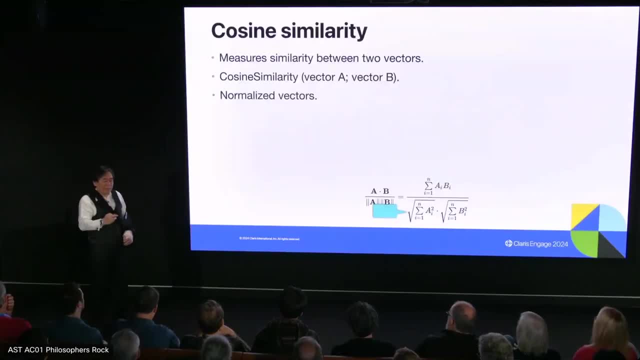 It needed to make a 1536 multiplication and a 1535 addition. And you think about it. if you want to do this for your all your vector, you might have a million vectors, So that could be also tons of calculation. 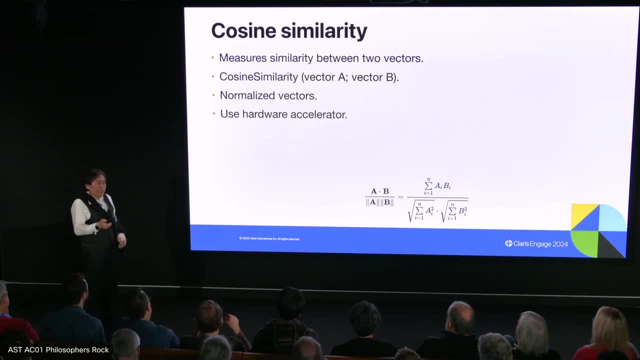 So for that we try to use hardware accelerator if your computer device has So. for example, if you have a AVX2 from Intel or AMD, we will try to use AVX2.. And if you have a AVX512 from Intel, 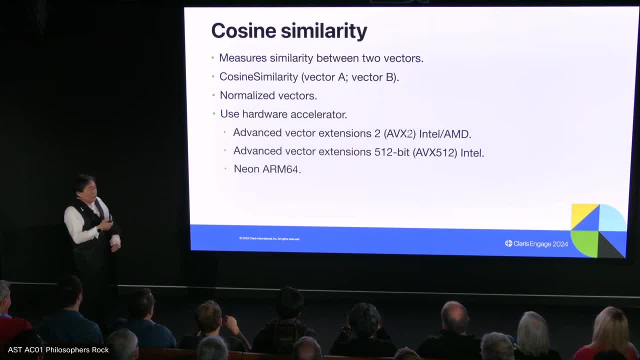 we will try to use AVX512.. And if you use ARM64 with Neon, we will try to use Neon. If you don't have this, don't worry, it still works, Just slower. But once you upgrade you will faster. 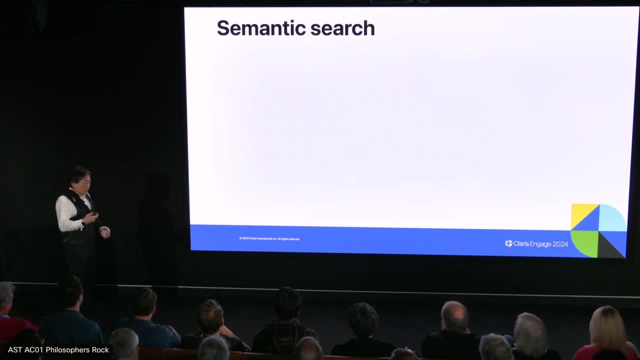 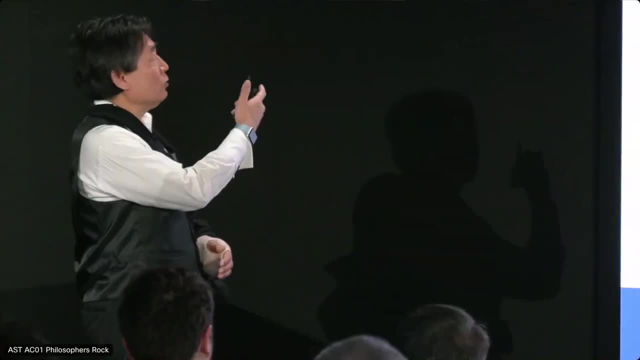 OK, so the next topic is semantic search, Since right now you have embedding vectors and you have this cosine similarity, so we can use that one to do the semantic search. So semantic search In modern keyword search it's based on the meaning. 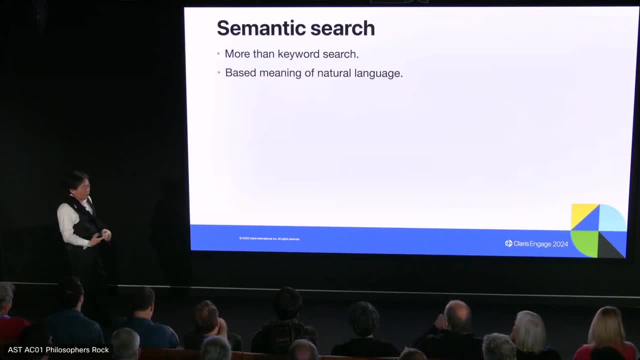 of a natural language And remember the cosine similarity compared to two vectors, And these vectors are from LLM, So that one actually can tell the meaning difference between the two texts. So we use the cosine similarity for the contextual reference And a lot of the time you probably 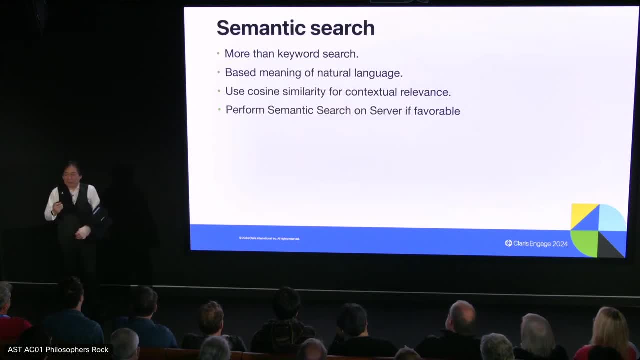 say you use the FindMaker Pro or Go and connect to server, So the server is based on the remote side. When you want to do the cosine similarity, the Draco engine protocol will check whether it's favorable to perform some semantic search on the server side or client side. 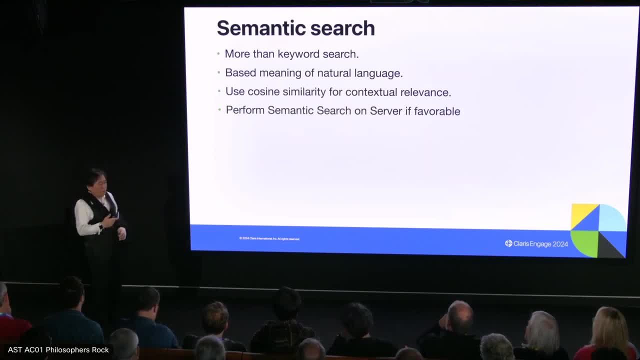 So, for example, if the server is not overloaded, say the CPU usage is under 25%, and you do have a lot of records and the majority of them are not downloaded yet, OK, It will implicitly perform that remotely for you to get the semantic search. 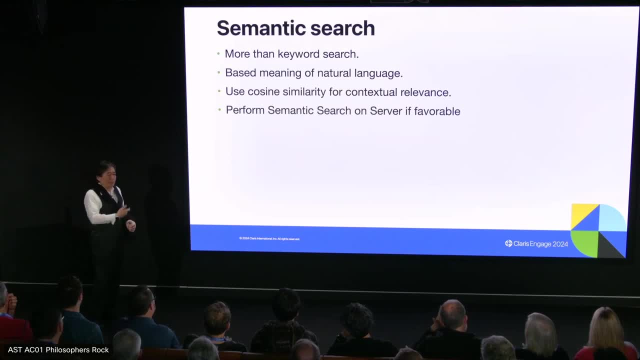 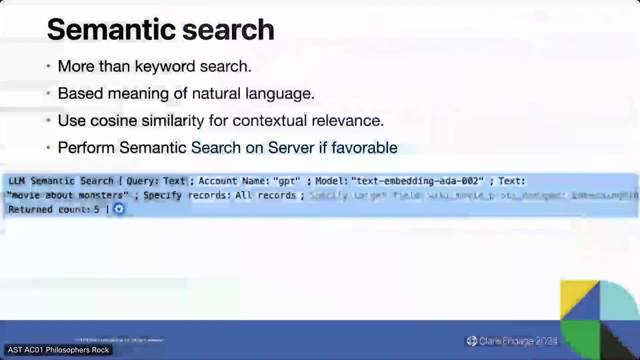 Otherwise you download all the records into your local machine and perform that. And here is an example of the semantic search script step. So this one, actually this one we just recently updated according to early ETS feedback. So let me just read it in English: 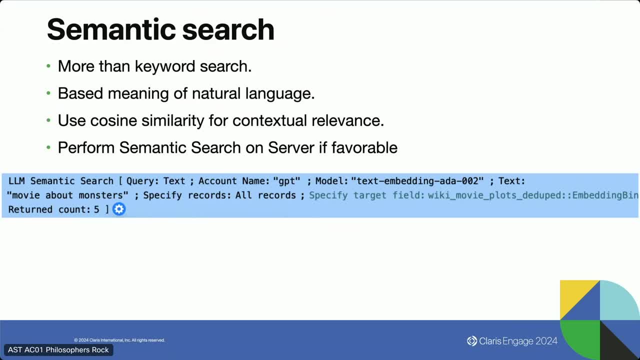 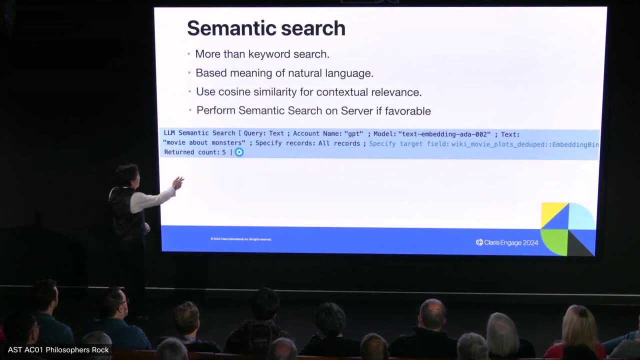 It looks complicated but not really complicated. So what this one is looking semantic search for movie about the monsters for Ulrich on the binary embedding vector And I'm looking for the top five. So previously we only can specify a text and to perform. 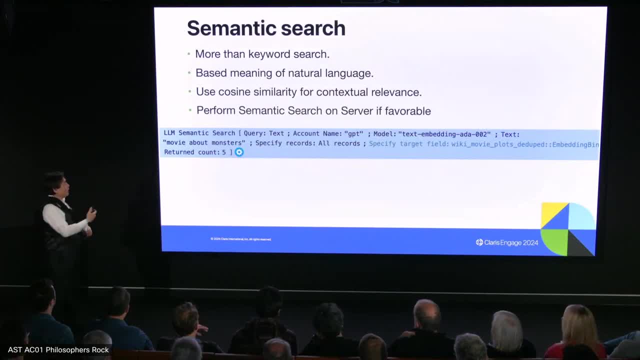 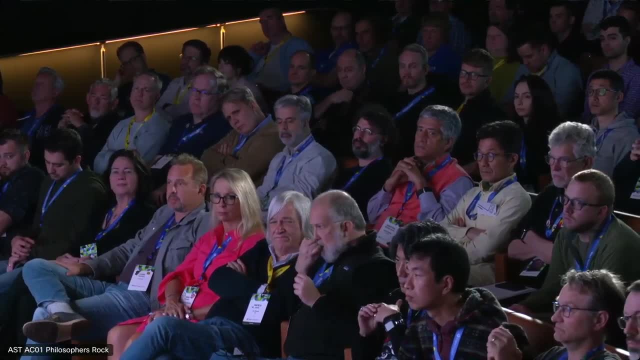 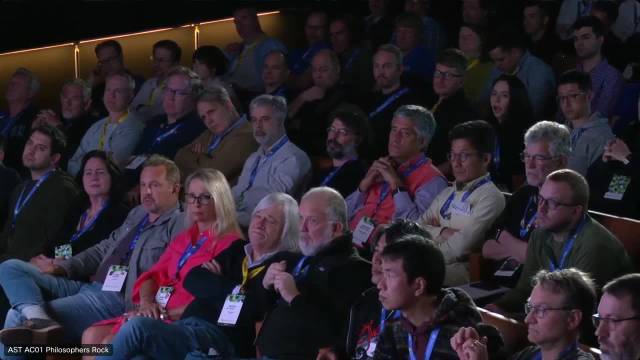 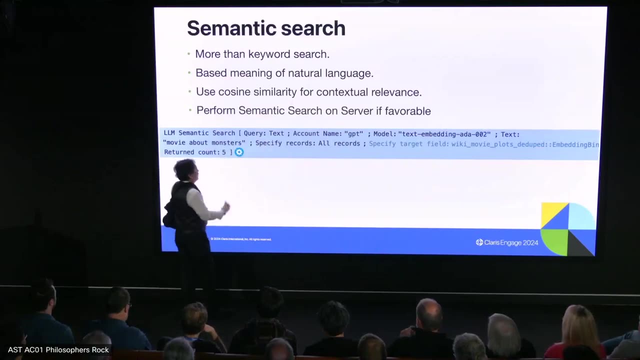 So this is the first one in the linear Python, And this one is going to show you the originalывайтесь of what we've done, And then the other one is going to show you how you can do the same thing. So, for example, you can have one line user ID text. 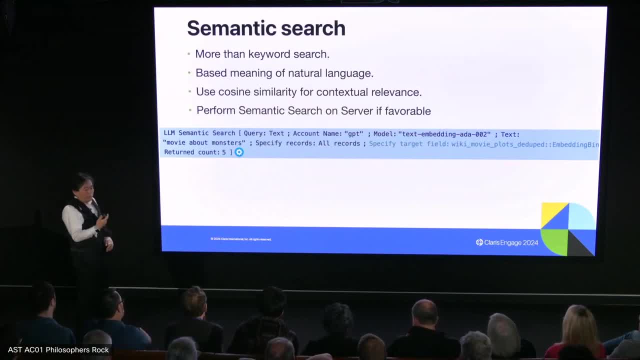 which we call a Vmode, And this one is the library ID text. And then the other one is going to show you For OpenAI, I use the text embedding 8.0.2.. And pay attention that model need to be the same model used. 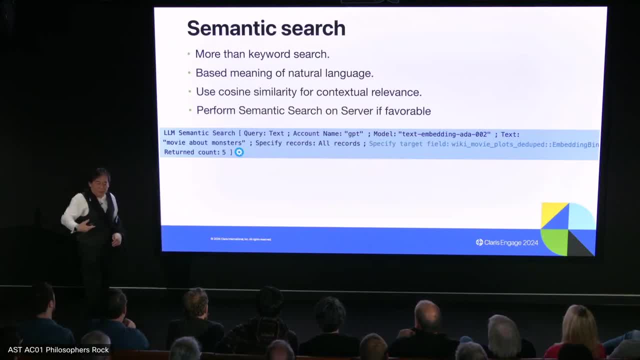 to bulk embedding or embedding for your record in the table And the text is quite straightforward. so I'm looking for movie about monsters. The specified record will have two choices. You can choose to do a semantic search on the whole table, all records of the table. 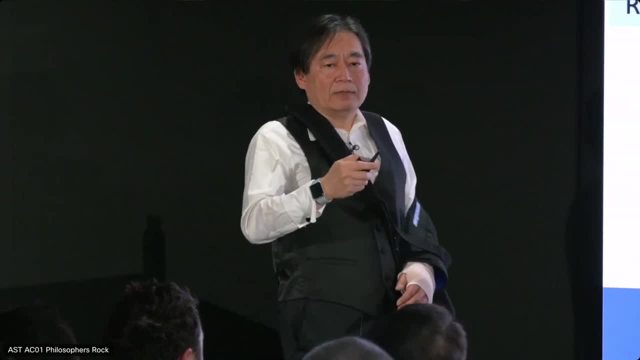 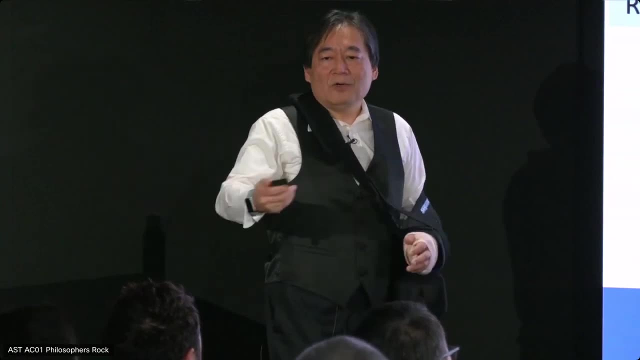 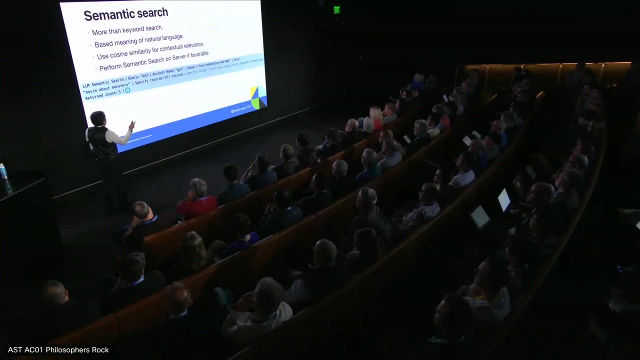 Or you can do that for current font set. So if you have font set, you have minimum record. you already narrowed down the font set to maybe 200, right, There's no reason you need to perform on the minimum record again. And the target field basically the field which you generated. 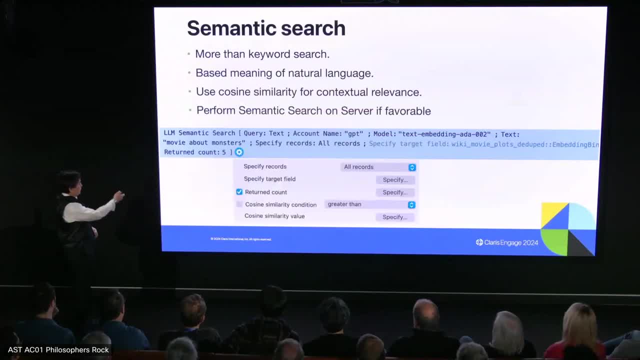 embedding vector before And we can count. we just say that. So here, if you click the parameter, you will see the option for you. So specify record: you can pick either all records or current font set And specify target field: you basically specify the field. 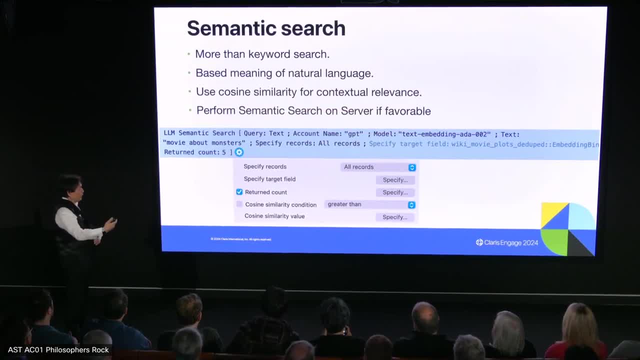 which you already have the embedding vector generated. So you can try that if the embedding vector is on container field. in binary format you are much faster And text form format still works, but slower. The return count: you specify a number for the return count. 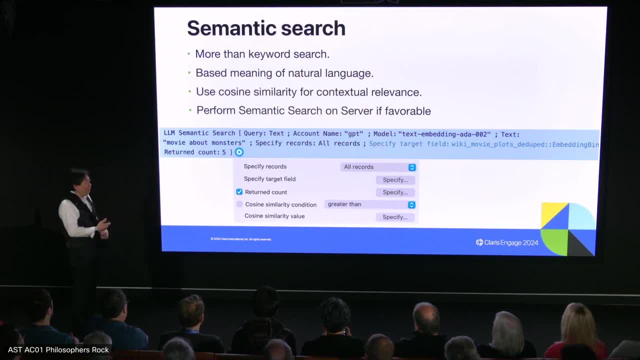 So, like a five, I specify in the case it's top five And you also can specify the condition for cosine similarity. But the default one is greater than, And you can pick greater than or equal, less than, less than or equal or even simply equal. 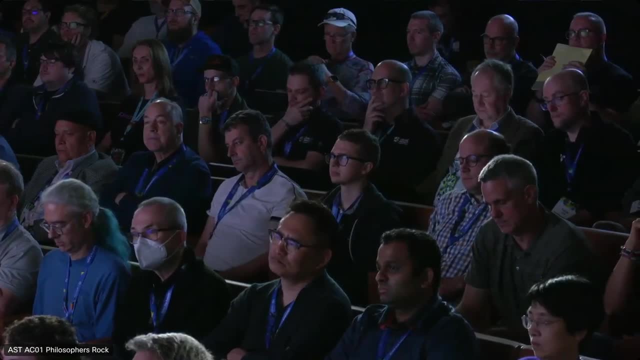 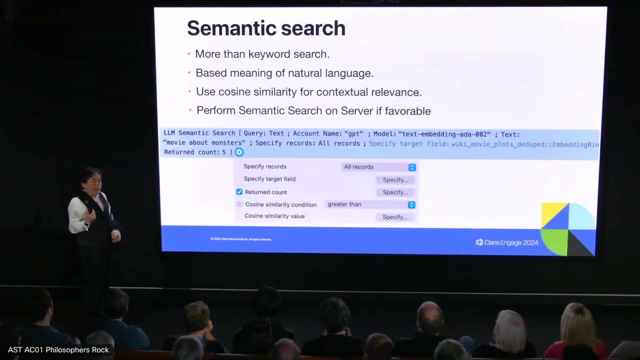 And the cosine similarity. you also can specify the threshold you want. So say, maybe you want to specify 0.9 for really close And on the other hand, if you want to check outliner the anomaly detection, maybe you want to set to the minus 0.9,. 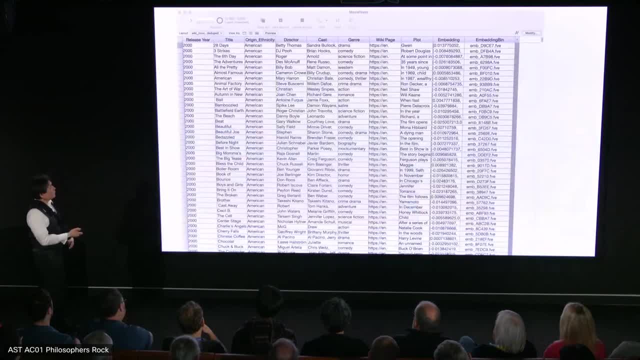 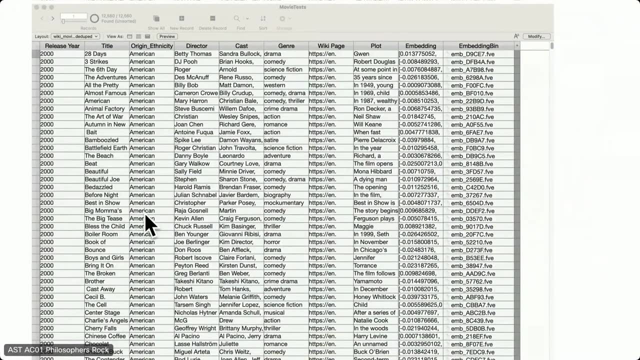 not minus 0.8.. Okay, so here is a quick demo about semantic search. So I have more than 12,000 records for movie database And each one have the description of the movie. So the plot field, basic description, I generally post the text form. 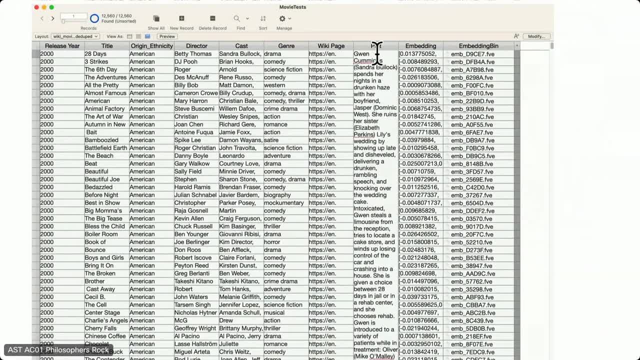 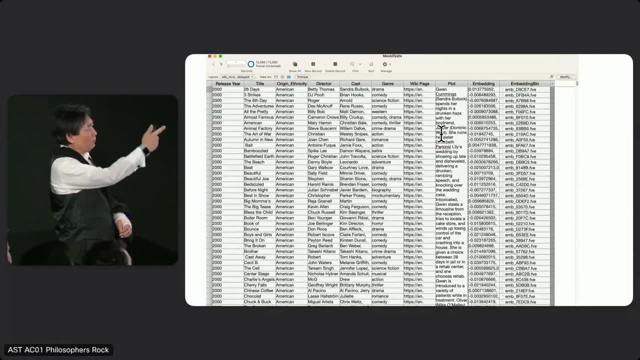 text format embedding and binary format embedding. You don't need to do both. So I do that for testing and for illustration purpose, So you can see the description describe the movie, And some of them actually are not in English. Okay so, because I already have the embedding, so 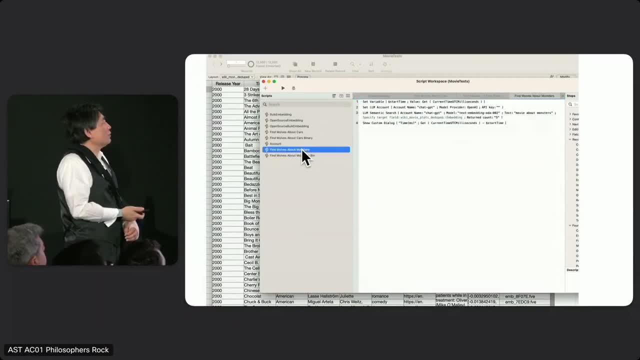 I can use a script to perform the semantic search. So for this simple script: basically, I'm looking for the movie about cars and on the binary field and I'm looking for top five. I also calculated the many seconds spent doing this semantic search. 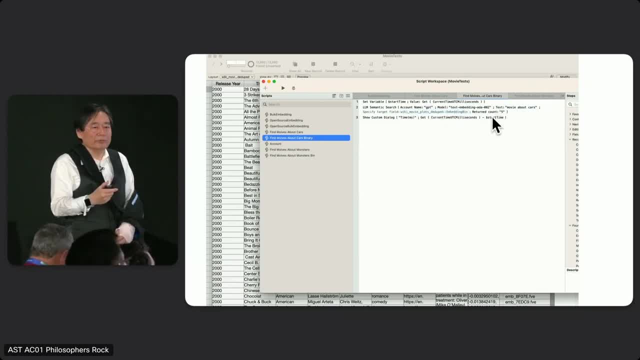 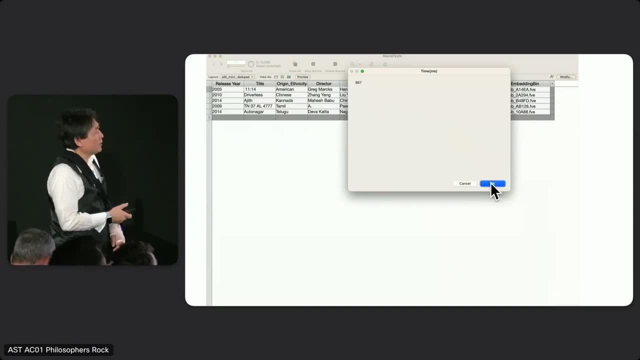 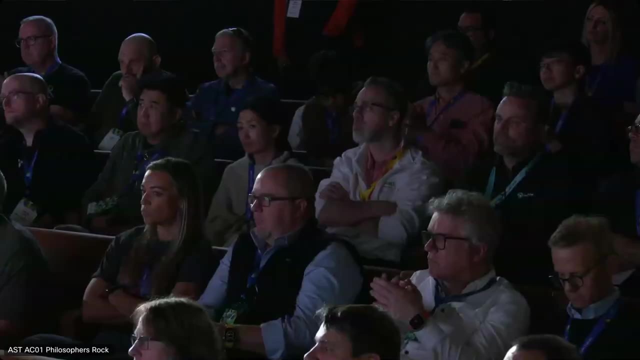 This was done on the M1 Mac's MacBook Pro. Okay, so let's click it and you can see. that's a finish in 0.957 seconds. Thank you, And you can see that the thing here. if you use the regular expression over keyword search, you cannot find it. 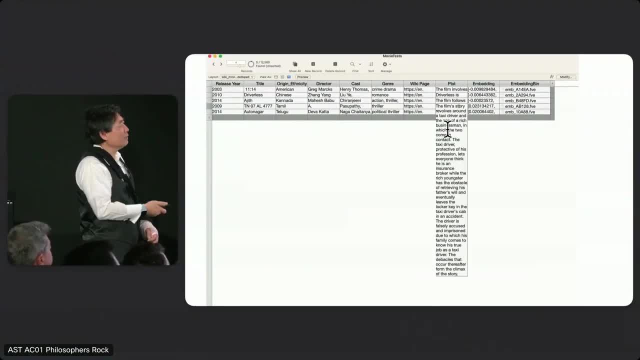 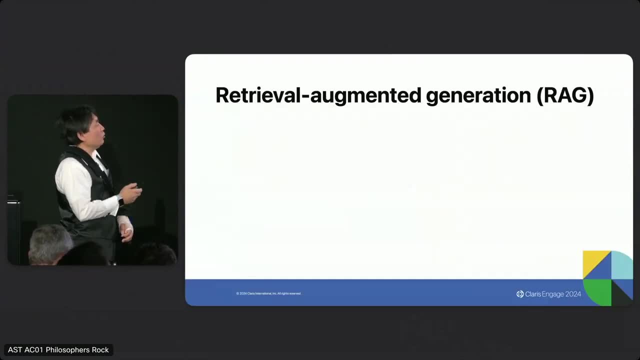 Like a driver that has a taxi driver. Okay, yeah, so that's it for demo. So the next topic is the retrieval, augmented generation, the IAG. So this is to check with document And we implement the IAG as a server. 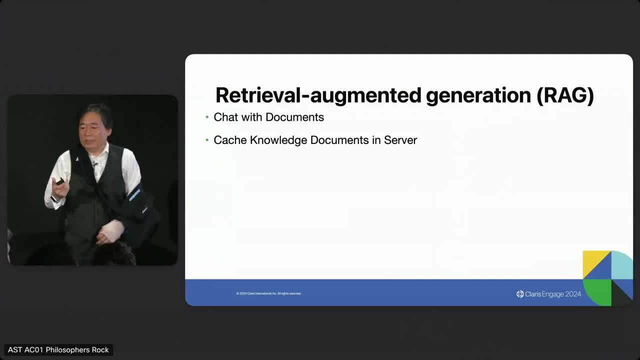 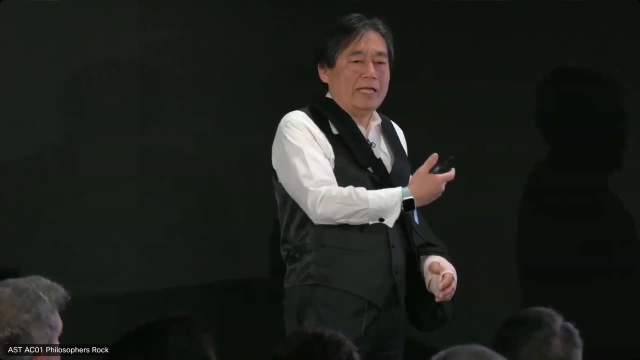 So IAG itself is a server And you can have IAG On the same machine of your FileMaker database server Or on a different machine. So say that in the development that I have the IAG server, FileMaker database server and the FileMaker Pro. 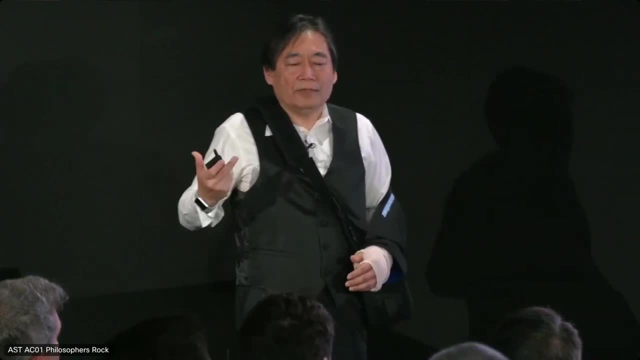 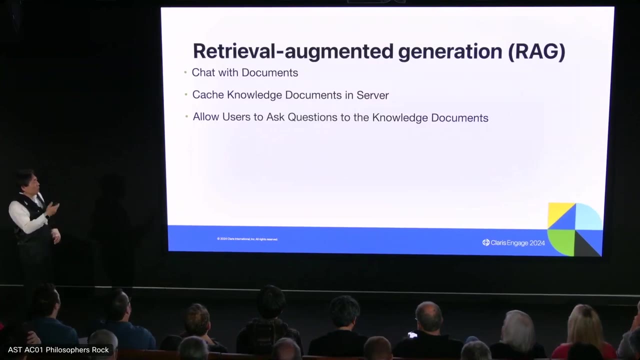 Even debug version. I can run it without problem on M1 Mac's Pro And it will allow user to ask question to the knowledge document, Just similar to the check with data. And the good thing about IAG is it eliminates the LLM hallucination. 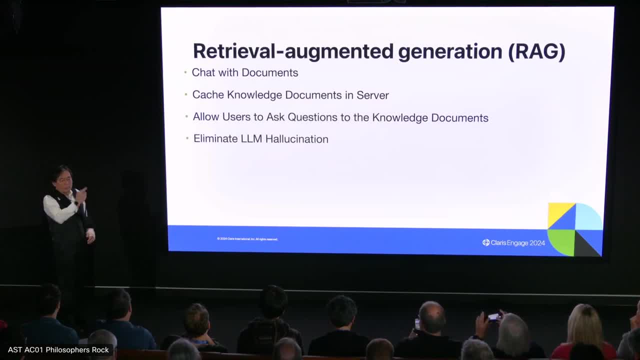 So if it doesn't know, it just say I don't know, So that's a good thing about it. However, if there are too many, don't knows right, That is not that useful. So we create a script that, so the admin can dynamic on demand. 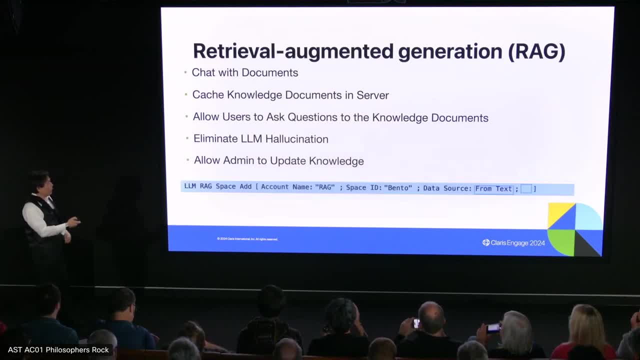 probably to solve those FAQs, And you can update it with either print text or with PDF file. So here is a script step. So in LLM IAG space add again. the first one is account name And because this talking to my IAG server, not to GPT. 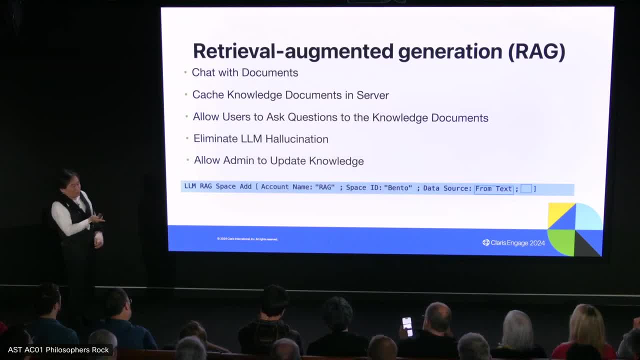 And so I have an account, IAG point to my local host And the space ID I set it for the Bento analogy. We used to have a product called Bento And- You probably for me. we said: And the data source you can specify from the text directly or: 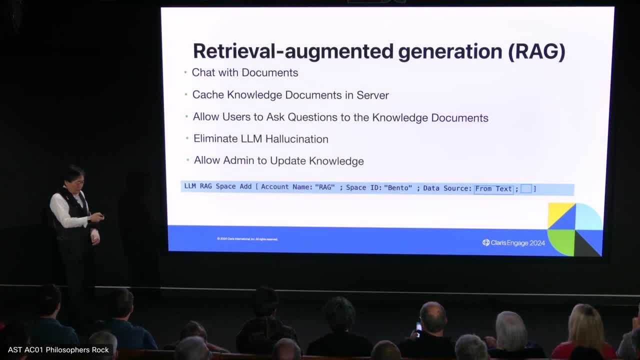 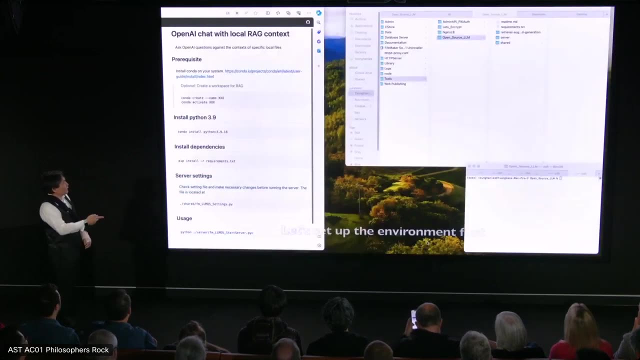 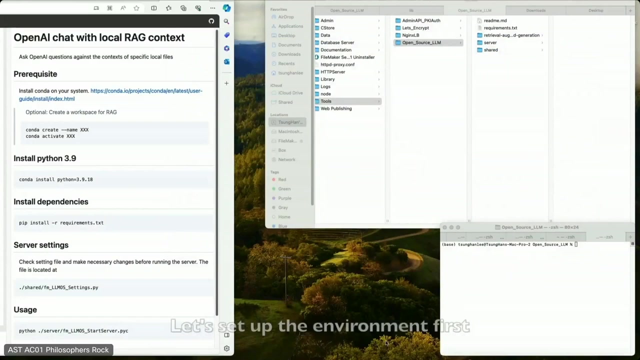 from a PDF file. So right now, the file. at this moment we only support PDF. Okay, so here is the standard script. step the file dialog. Okay, so the next demo I'm going to show you is how to start this IAG server quickly. 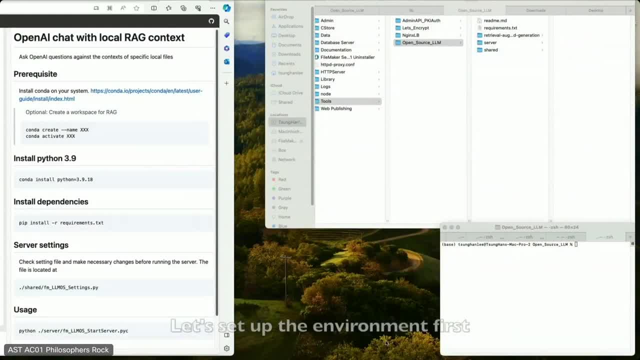 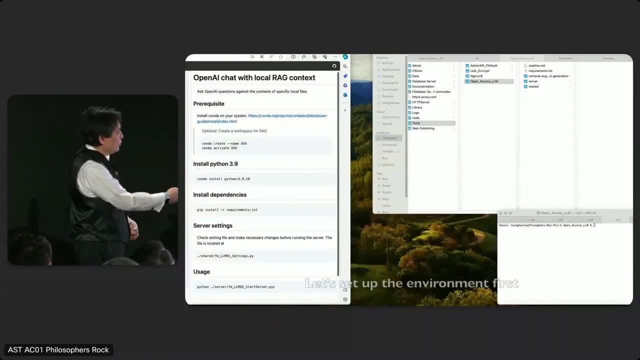 On the left-hand side, here is the remaining file we included in the server package So it documented each detail step to set up and run the IAG server. On the right-hand side, the top one is server installation on Mac And you can see the directory structure. 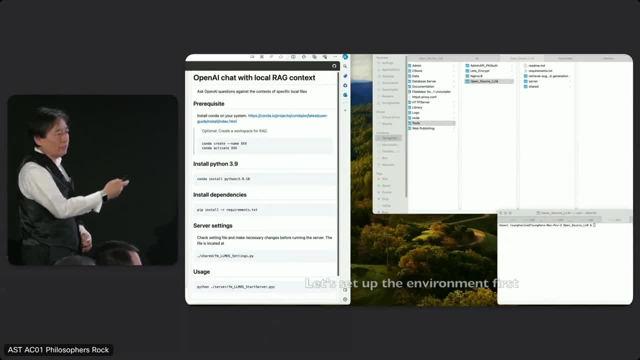 And the lower corner actually is the terminal window, will show you the progress of the setup. So we use the to set up the environment for Python. So, and the virtual environment are the two popular one to encapsulate the Python environment, And so here we just simply use the to create workspace. 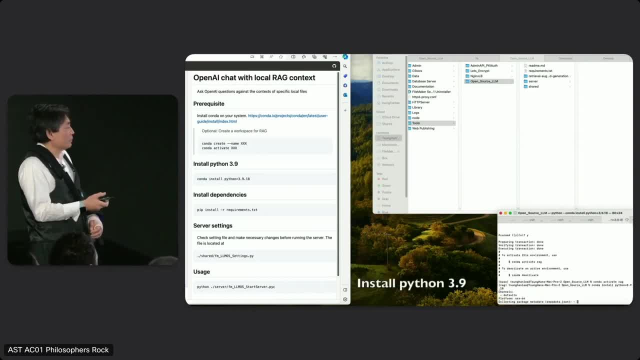 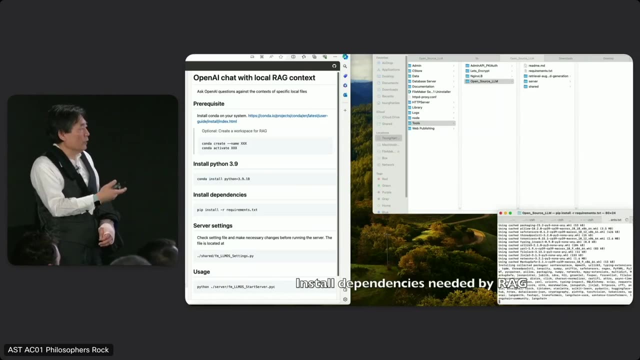 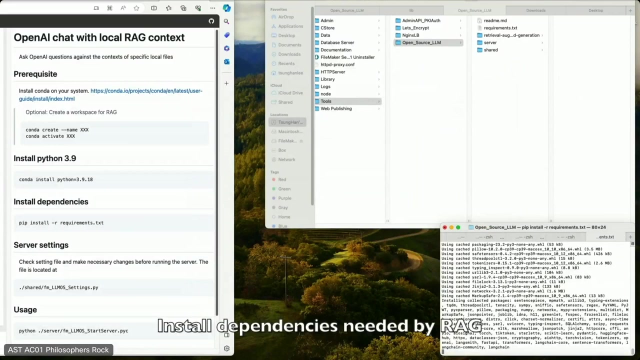 And then we install the Python 3.9.. Yeah For the workspace. And then we install the dependence library. Dependence library. take a little bit time to install. It, take like a couple of minutes. but that depends on your computer and those network speed. 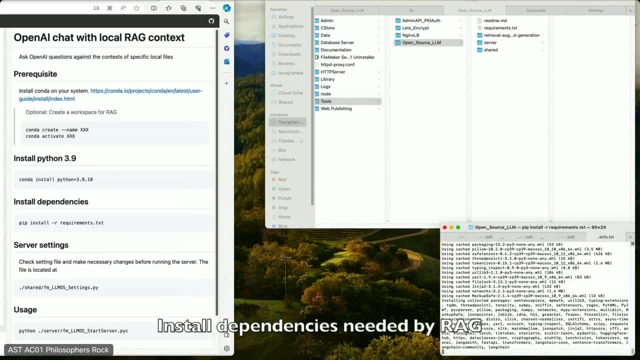 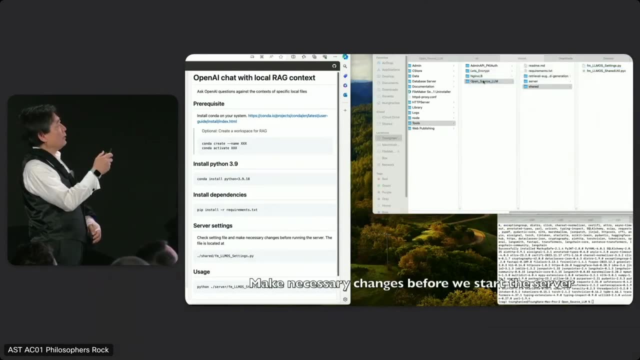 However, this is actually. this is just done once. Once you finish it, one time it capture in the contact environment And the next time you can just simply start. You will be quick. So after you install that, before you run the server, 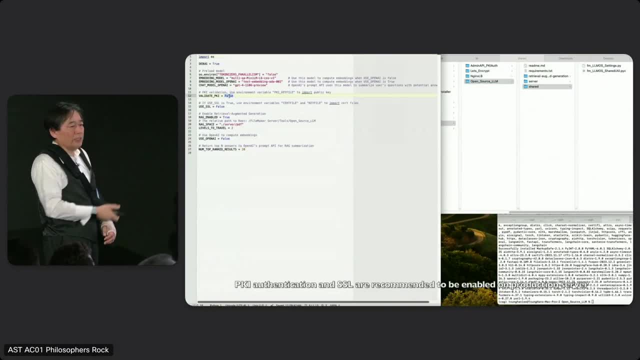 I suggest you open the settings file and change the setting according to your need. So I highly recommend you turn on the PKI verification SSL if you run the server on a different machine, even for development. That's a general security purpose. And if you have a, then if you have PDF file or you know. 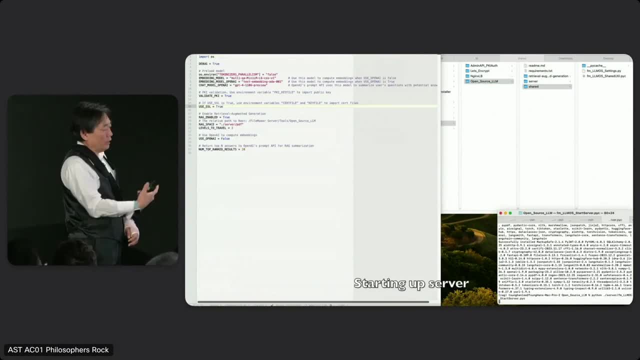 you want to. you know you want to use the. you know you want to use the. you know, in the folder of the RIG server it can load it when it starts, So you will generate embedding vectors and cache them and ready to answer question. 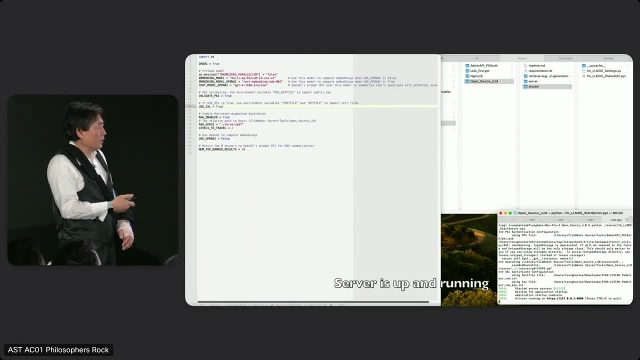 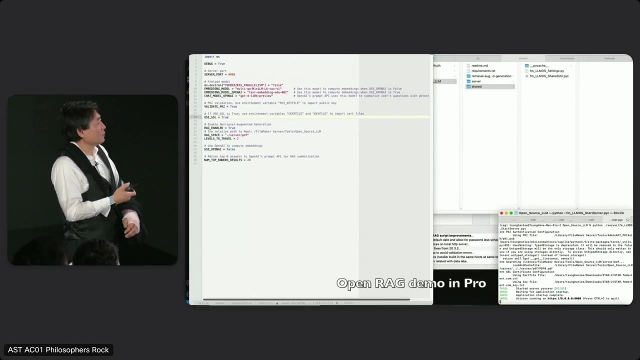 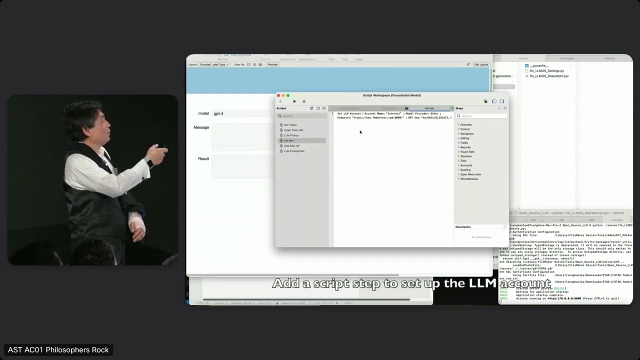 Okay, so now the server is starting. So since the RIG server is up and running, I'm going to open the FileMaker Pro to check with the RIG server. So let's take a look at a script there So you can see the similar one. but 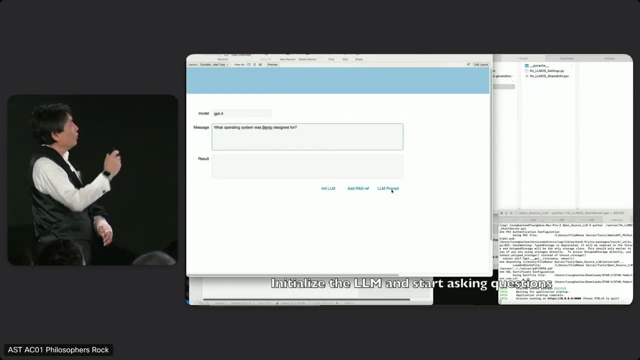 at least the account is RIG- point to my local host And I can start asking questions about Bento. say, Bento was designed for Mac OS, And we can continue to ask more Bento questions. And I ask: how many library templates are there in Bento? 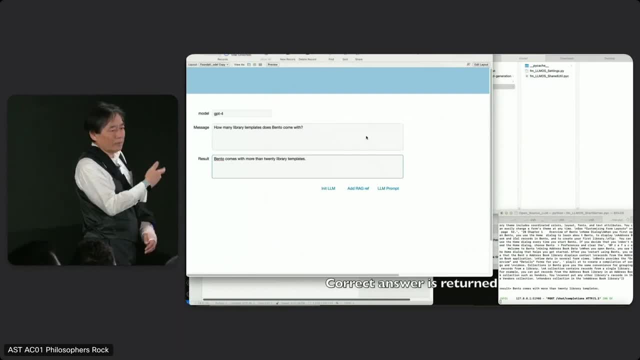 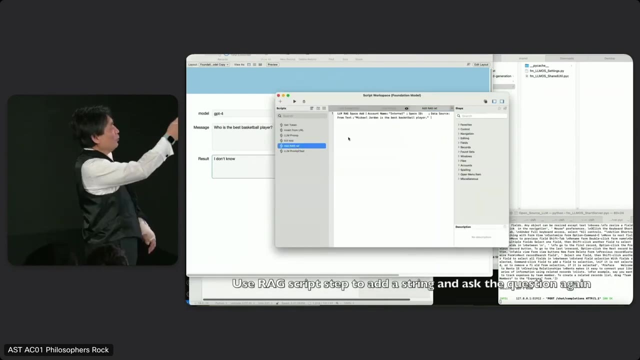 So we find out there are 20 library templates in Bento. Now I'm going to ask him something totally unrelated. I'm asking: who is the best player? What? What? Bento, you're right. So now we want to teach it. 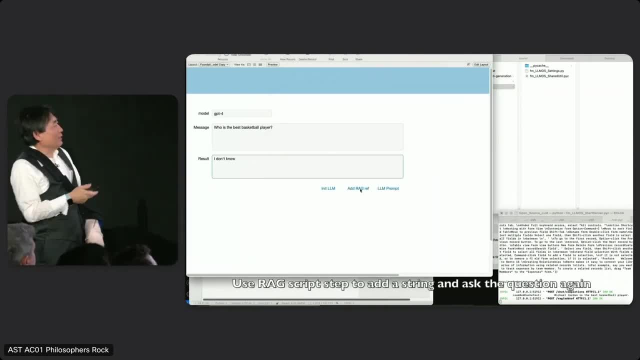 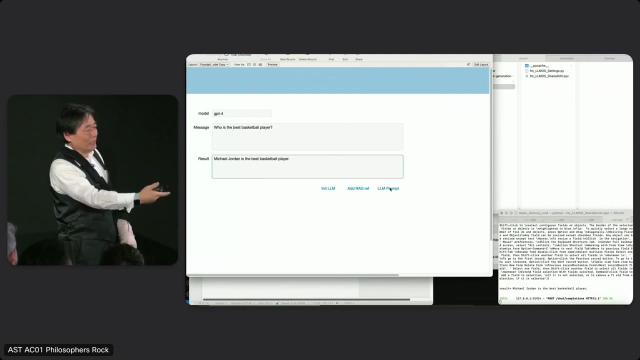 So that we add: Michael Jordan is the best player, So let's add in. you can see from the window And when we ask question again, you will say: Michael Jordan is the best player. So when you set up the RIG space, 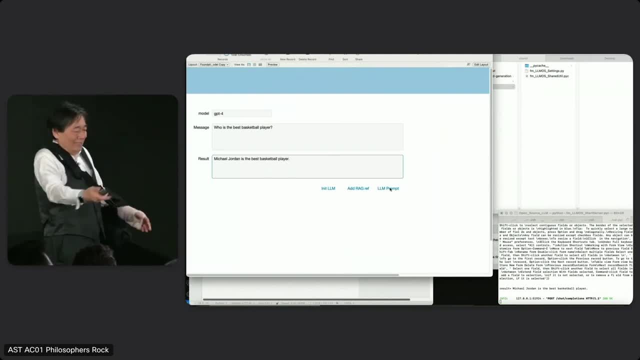 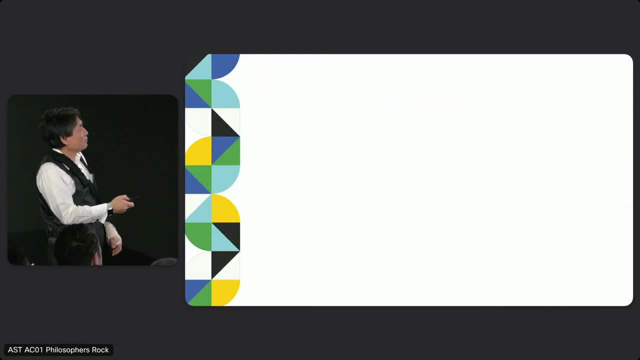 actually, you can put your name. you are your best player. Just don't add my name, Okay, so next topic is open source LLM, And so there are a lot of open source LLM, and some of them are pretty good. 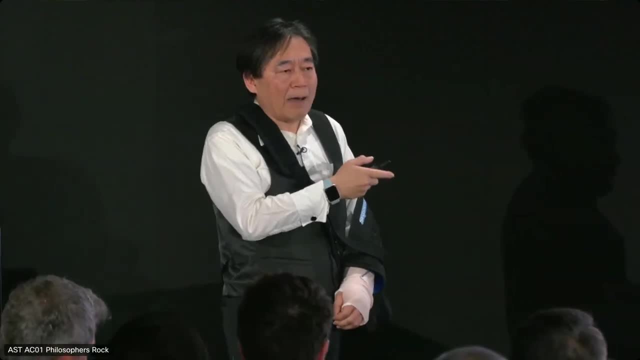 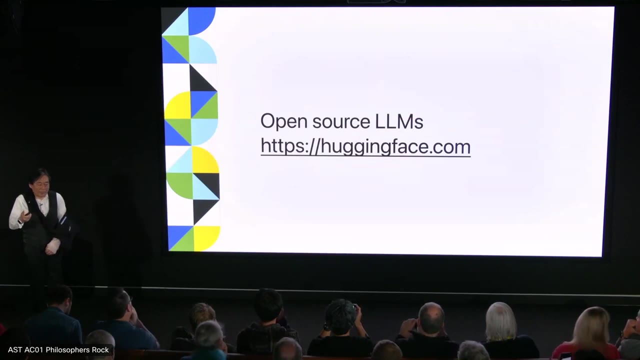 So if you are interested, the HackingFacecom is a hub, So it has a. actually, you have more than LLM models. You have a lot of models and also with a lot of data set. So good thing about that is with the data set. 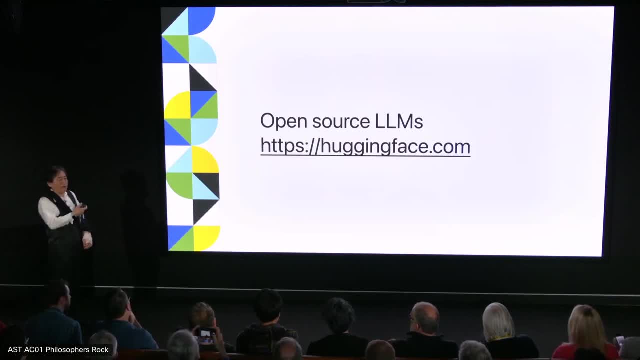 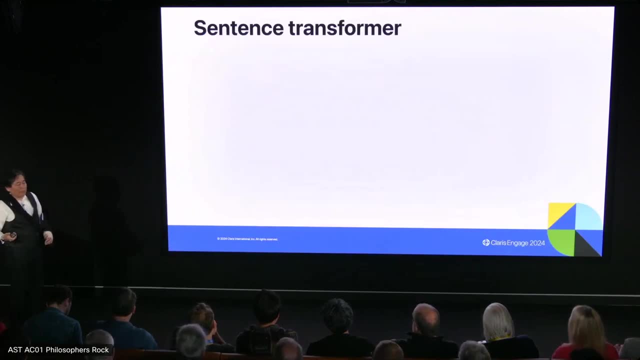 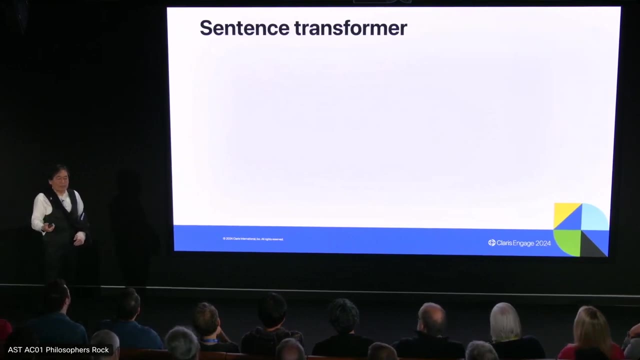 you. potentially you can find team, Find team LLM for your special purpose. Okay, so there are several kinds of LLM model you might interested from open source. The first one probably is a sentence transformer. What sentence transformer What does is to generate the embedding vector for you. 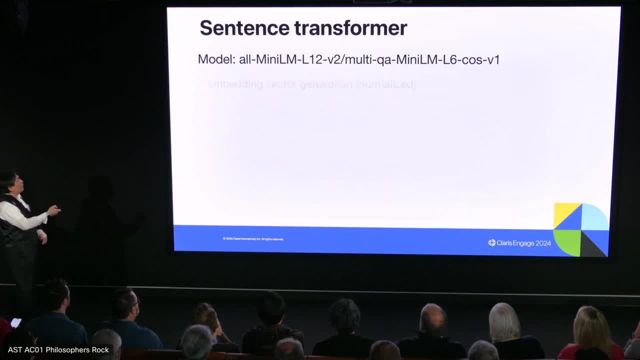 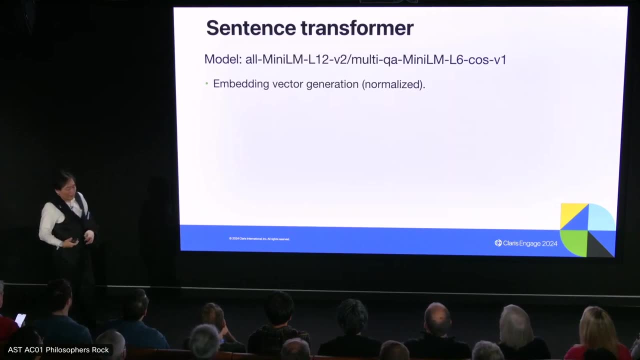 So we have tested several of them and these two seems to be good. And but the first thing is, remember I told you that we need to use normalized embedding vector. We only want to store normalized embedding vectors in 5 megabits database. 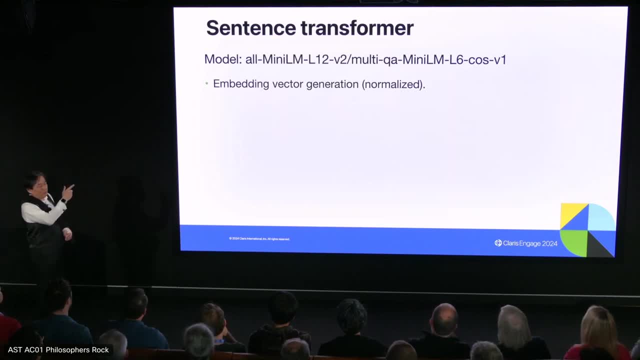 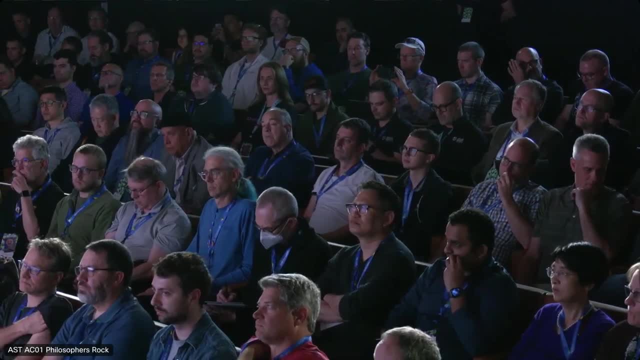 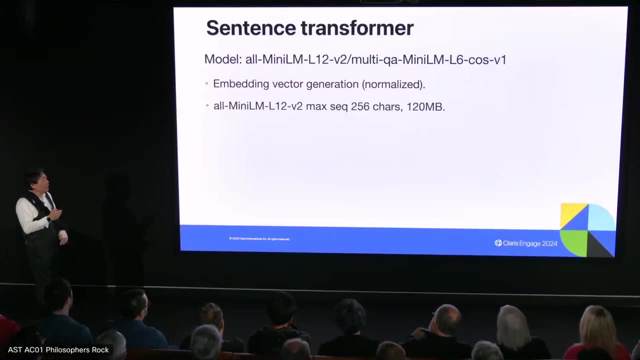 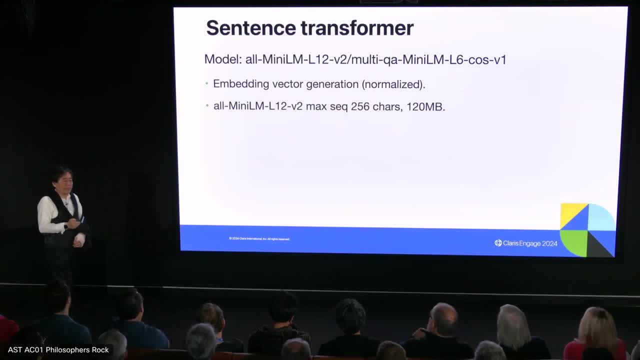 The maximum sequence is 256 characters. What that means is, if you send the text more than 256 characters to generate embedding vector, it will truncate anything after 256. So you need to pay attention, All right, Otherwise you might get some. 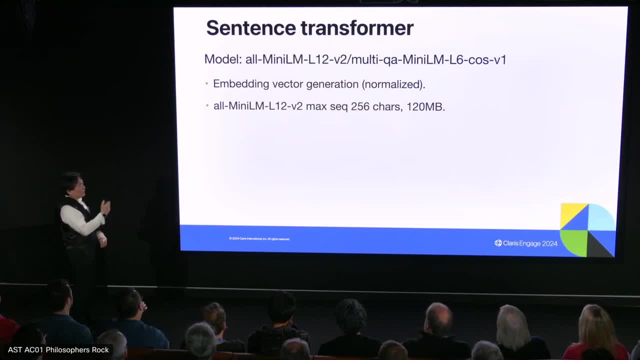 Unexpected results. and another thing is the size of LLM. So for this one it's 120 megabytes And the second one the multi QA, mini LLM, L6, cosine V1, the maximum sequence doubles is 512.. 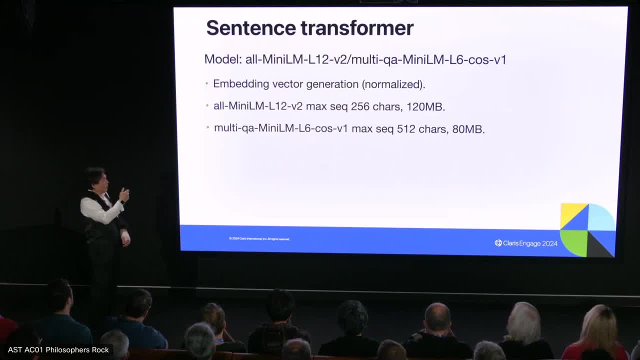 Actually the demo I showed you, the IC server is using this open source LLM instead of OpenAI. If you want to use OpenAI, you just switch in the setting. You will use OpenAI. But since this one is pretty good, it's useful. 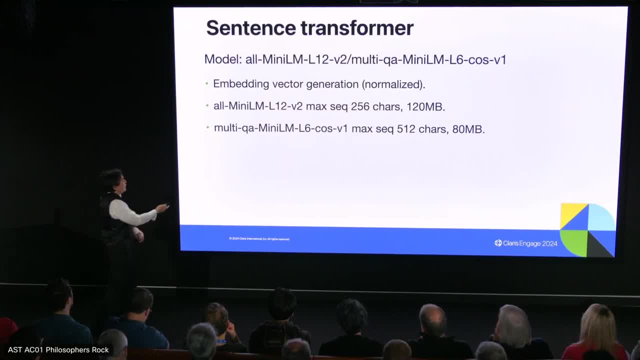 So, however, that's up to you for choice, And this model actually is a fine-tuned version for cosine similarity and the size is smaller. So both models, the embedding vector dimension size is 384.. So it's much smaller than OpenAI. 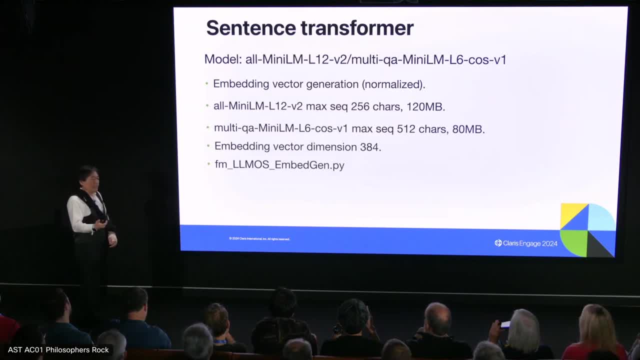 Just like the IC server, we provide the document that we meet document, also the Python script. So if you follow it, it should be easy to quickly bring up your own sentence transformer for either of these model or you find a newer model that fits for you. 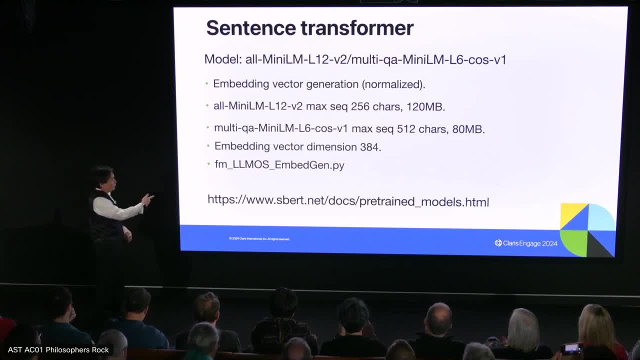 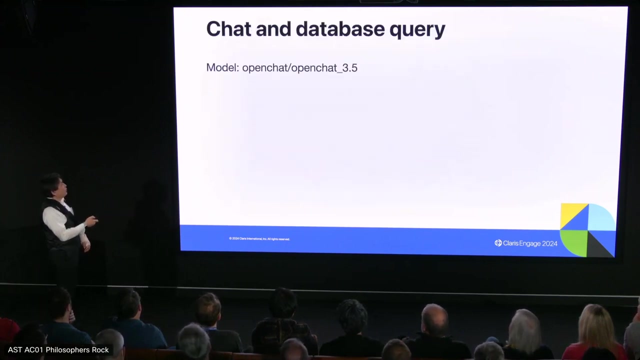 And here is the link that, if you are interested to bring up your own sentence transform server, the expertnet has a pretty good document to compare the current available sentence transformers. So because time limit, so I don't demo this one. Okay, another kind of LLM in my interest to set up is OpenChat 3.5. 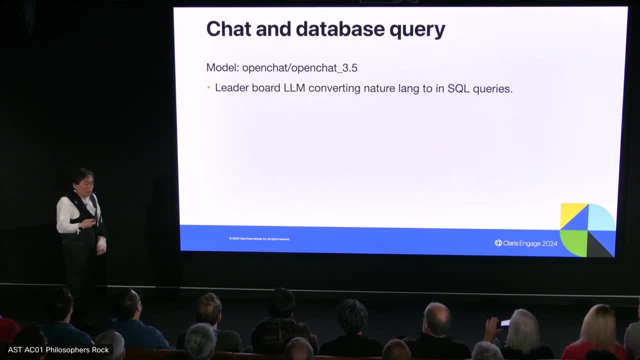 So which is the LLM? for chat and converging natural language? Okay, Okay, Which is SQL? So normally the 7 billion parameter one is good enough for general purpose And according to its variation on the side with SQL eval, this: 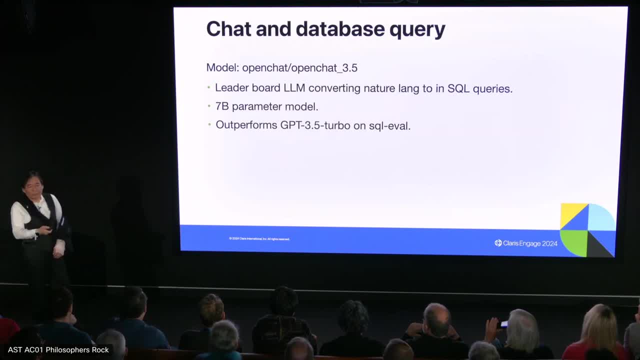 the OpenChat 3.5 output from GPD 3.5 triple, But of course not as good as a GPD 4.. However, it needs a high end. So if you don't have a high end, CUDA support first. if you don't have enough memory when. 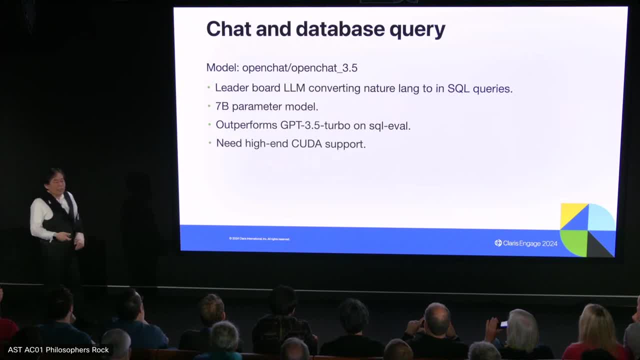 you try to run it, it will give you error out of memory. And if you have enough memory but still not enough CUDA- I mean the immediate GPU support- then the response could be slow. Again, we provide the readme document. also have a Python script. 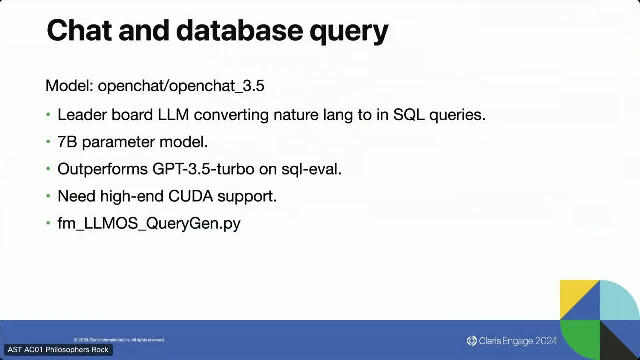 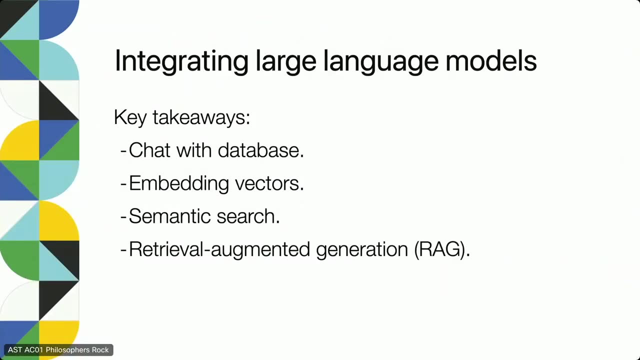 So to help you to start your own open chat server if you like. So because time limit so I don't demo this to you. Okay, so we have went through quite a lot. Remember, in the beginning we talking about the key takeaways. 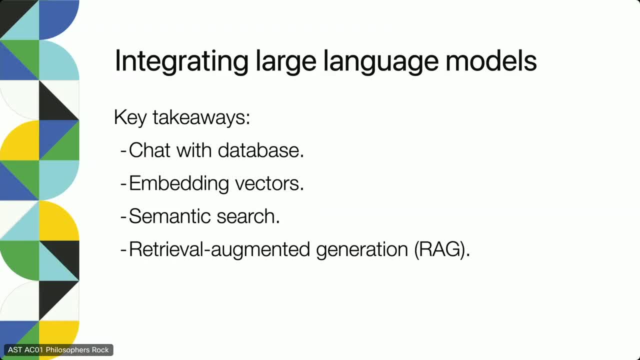 So you have seen the chat with DevOps from the app assistant And, technically speaking, you can directly use the LLM prompt to check with database if you like, And you see the embedding vectors. So you know how to get the binary, how to use the LLM embedding or. 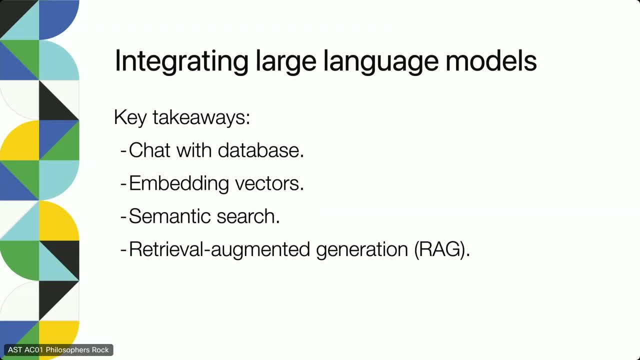 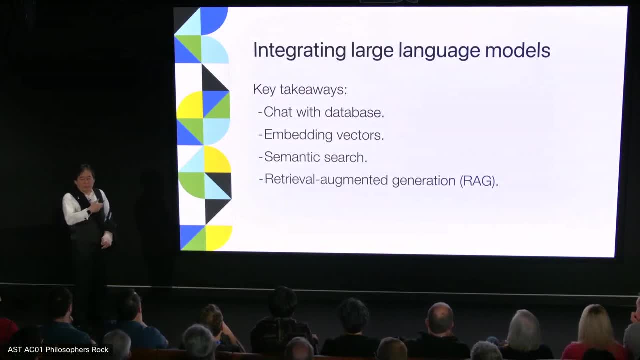 LLM book. embedding- to save- embedding vector into a file maker database. So if you create a field of text field, it will be text format. If you create a field of container field, it will be binary format And you know how to do semantic search. 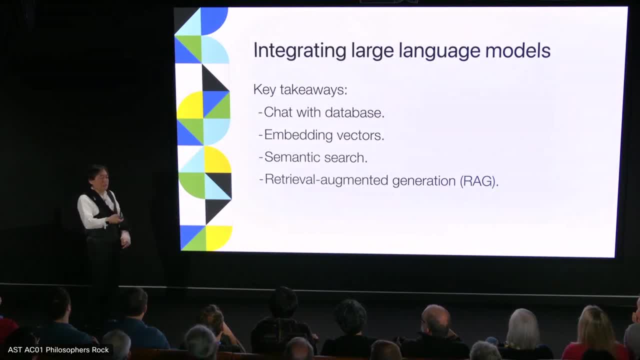 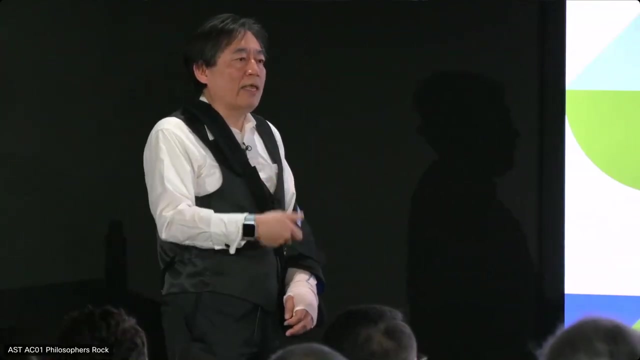 Just use LLM semantic search And you can give me the text against the table with embedding vector, Or you can give it an embedding vector pattern with the embedding vector to compare, And you know how to set up the IG server and then have it cache the PDF file to answer questions. 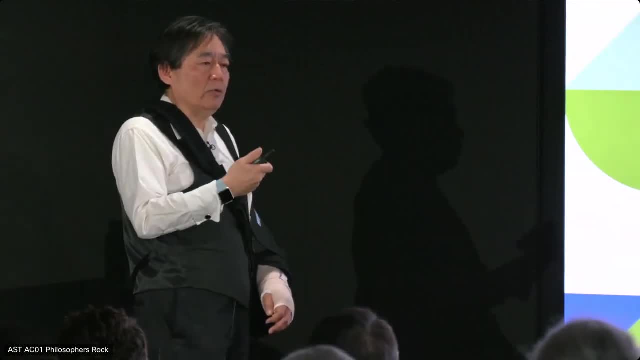 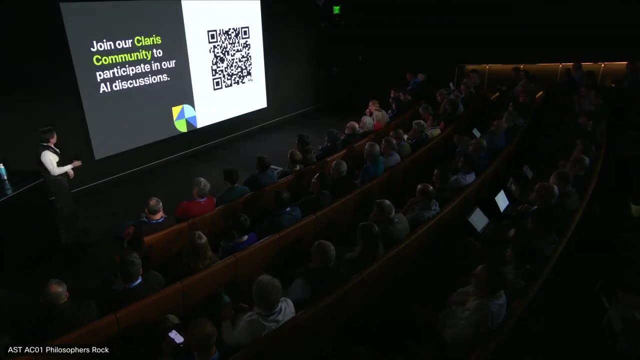 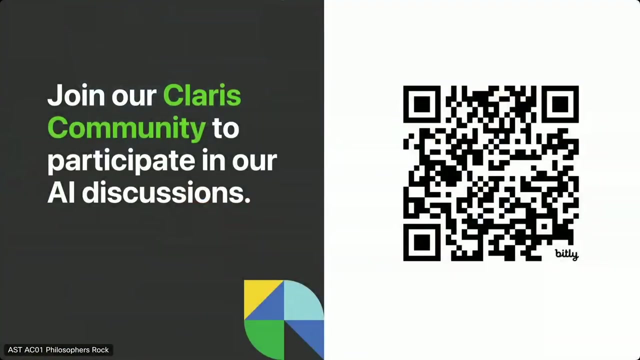 And in case, if you want update any time, you can use the file maker script To add new information to it. Okay, so please join our careers community to participate in our AI discussion. Together let's build incredible things, All right, thank you. 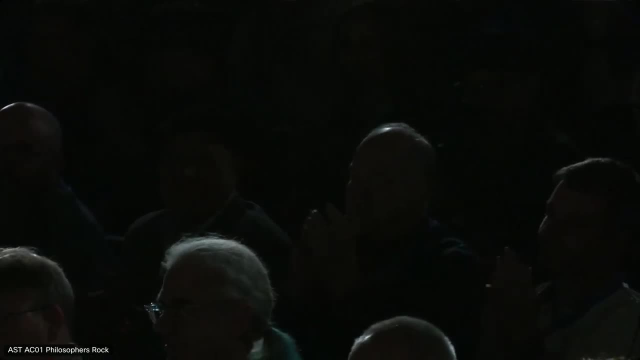 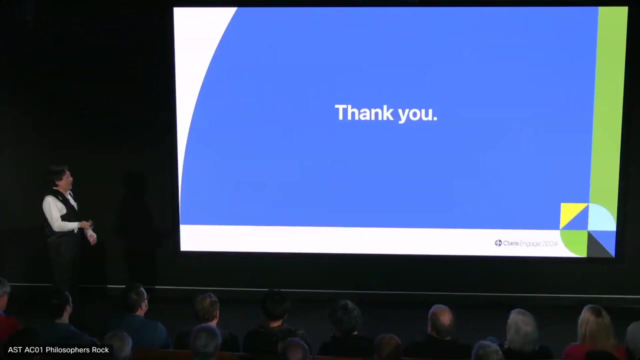 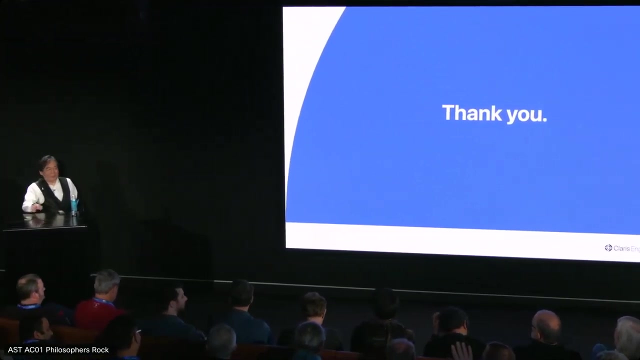 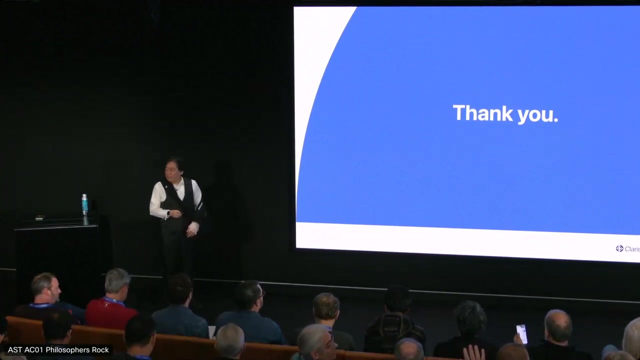 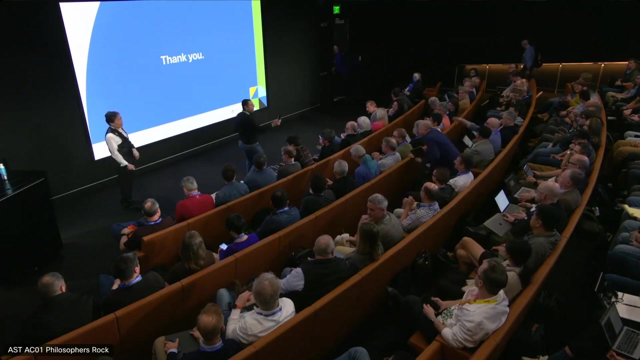 So I cannot wait to see innovative solution from you. So thank you. So now we for All: question and answer. So any questions? Yeah, Yeah, Any questions Back here. Yeah, I'm sorry, I'm sorry, I'm going to pass over. 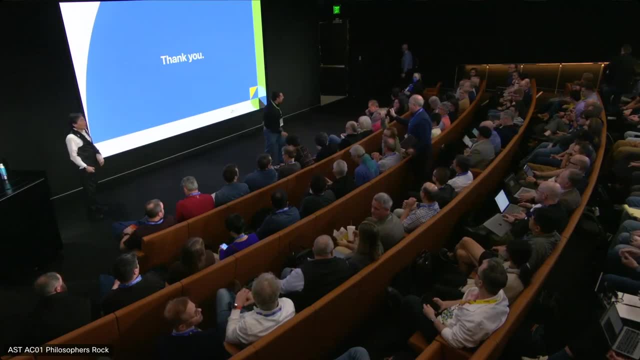 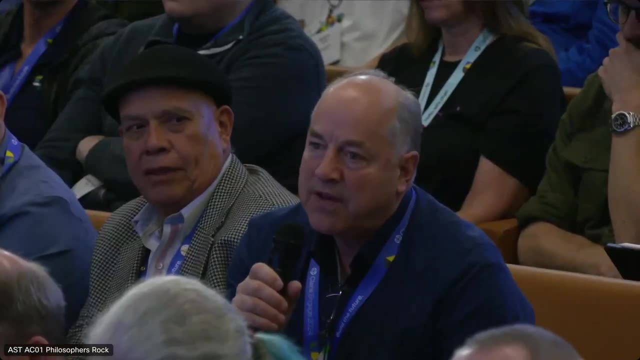 I'm going to help this out. Okay, Okay, Okay, Okay, Okay Okay, Thank you, Very nice To vectorize your data. is there any way to do that locally without having to send it to a service? Yes, 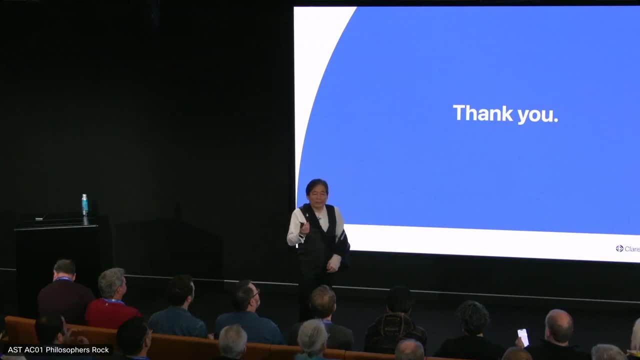 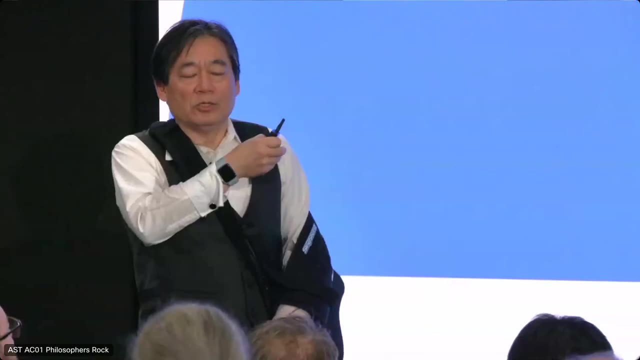 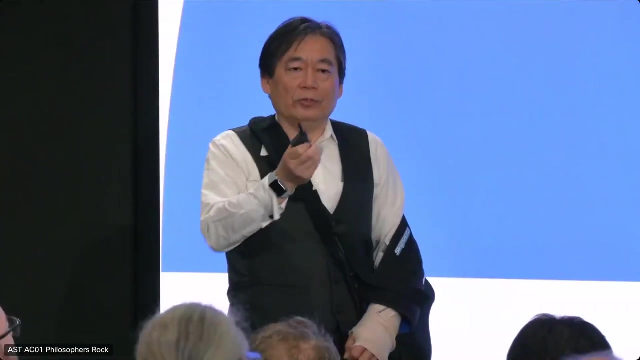 So if you want to get embedding vector, data, embedding vector- right. So if you run the sentence transformer right- Remember I showed you the sentence transformer- You bring up the sentence transformer server locally. Then you can just talk to it. Equally account to point to it. 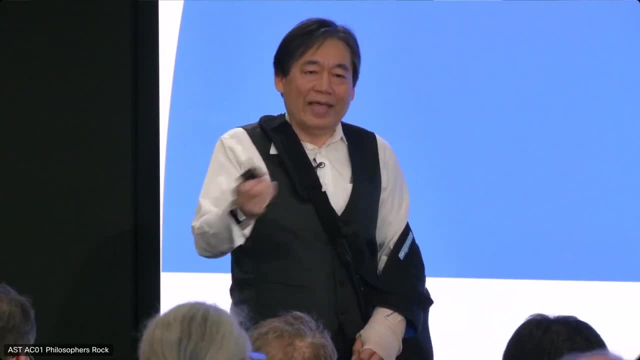 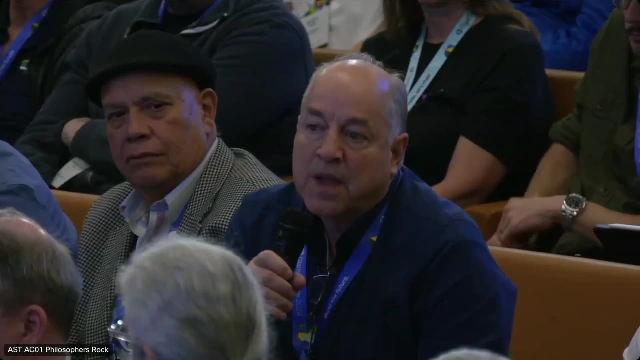 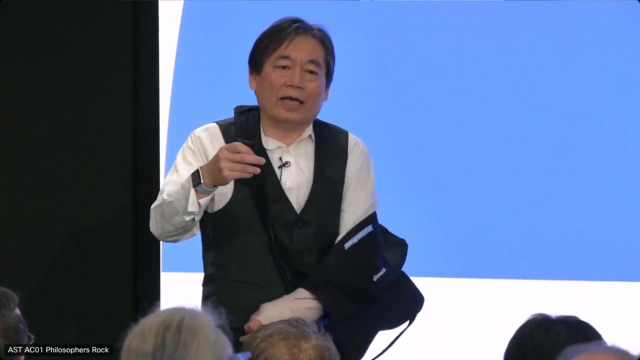 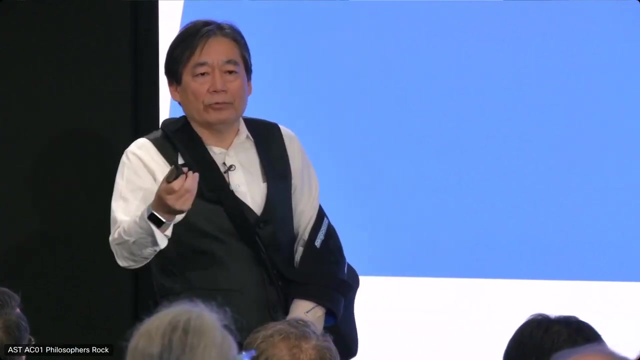 Your local host endpoint, Then you will be able to get an embedding vector. But I thought the vectorization also had to do with what model you were using. Yes, So remember, I showed you the IG right. The IG the vector actually is from the particular sentence: transform model. 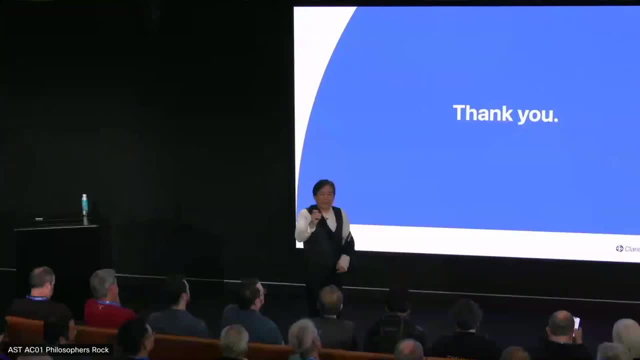 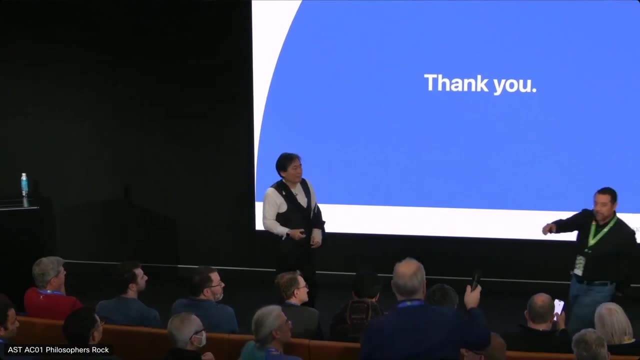 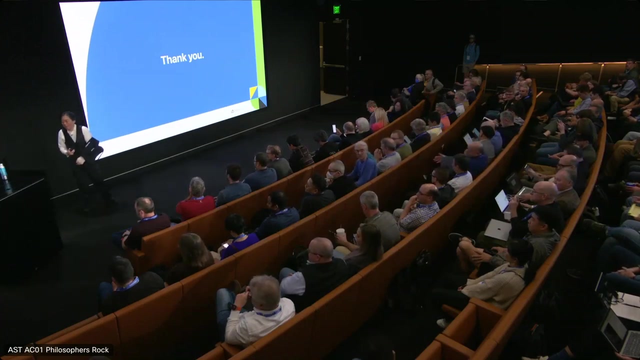 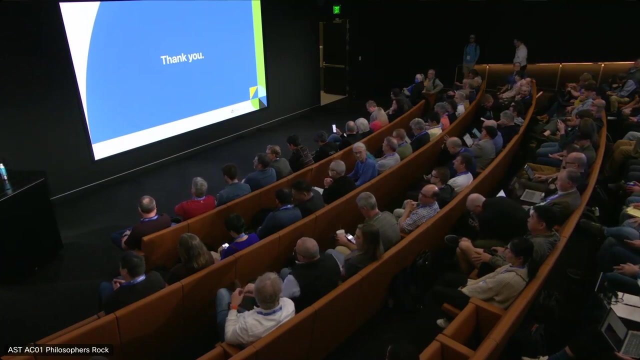 So it's fixed. Yeah, Yeah. So that's the reason that I suggest don't mix embedding vector from different LLM. Yeah, We have one back, one back here. I'm gonna run that. Thank you, Rami. The file maker data. is that limited to a file on the server? 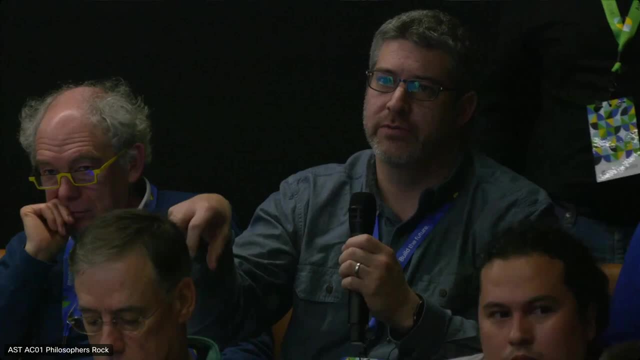 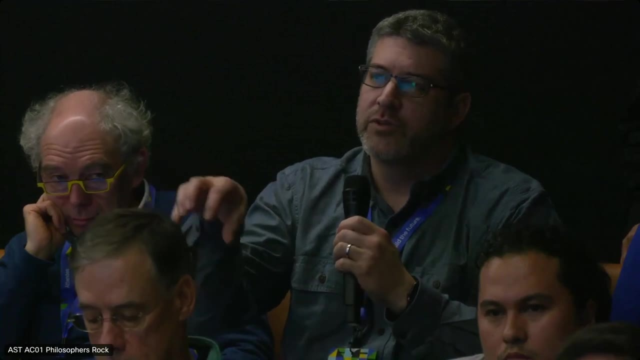 Can you? can you pull from multiple files on there On the server? Can you? can you source from multiple servers In the file maker server? right, Yes, Right, but the when you run this in in the file, right. 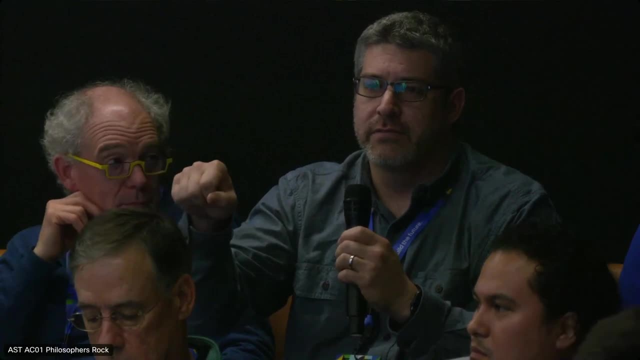 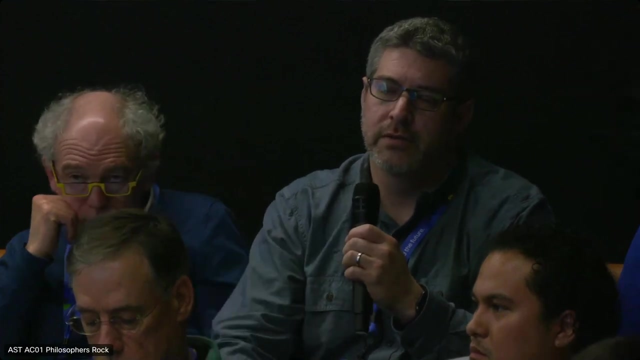 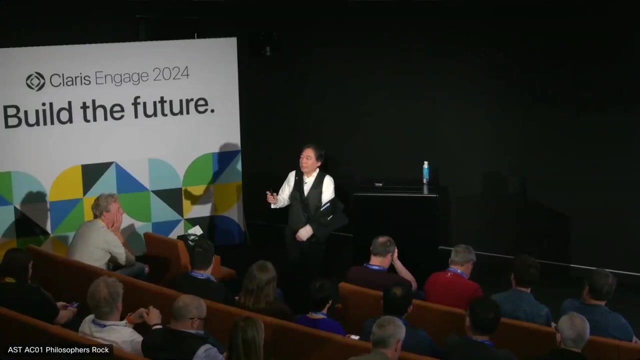 Like there's a, there's a table and it has Right with the data to to to work on, Yes, that that Can that be located anywhere? any server? Yeah, Multiple servers. So so it it mean it mean the embed where to store embedding vector. 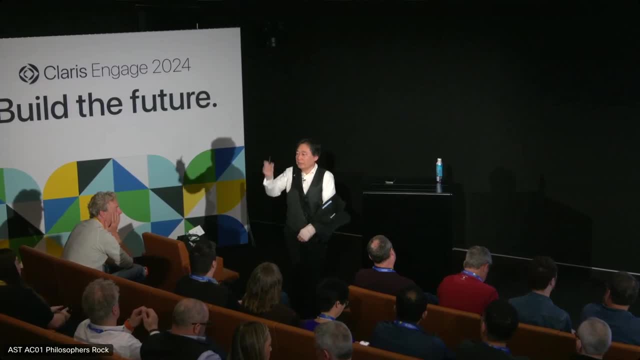 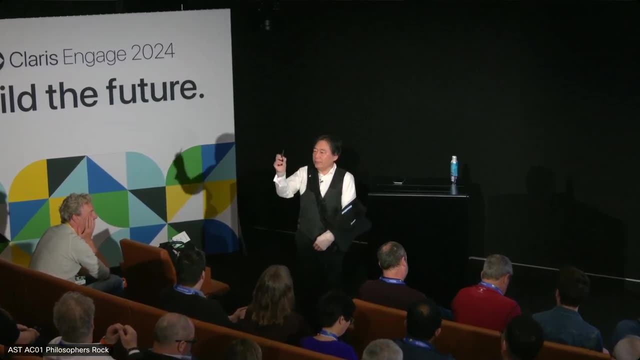 Yeah, So so it. it mean it mean the embed where to store embedding vector. Yeah, Yes, so you can, you specify as long as you can access the, the table, and then you, you create a field in there. 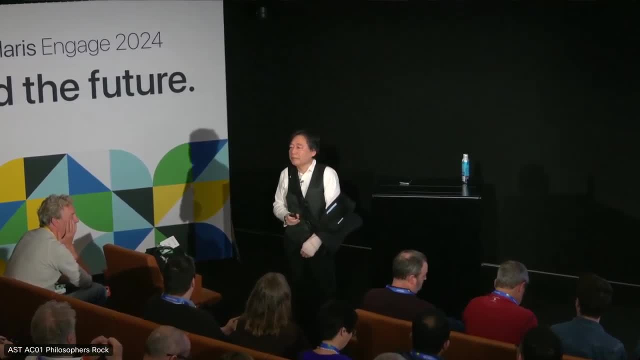 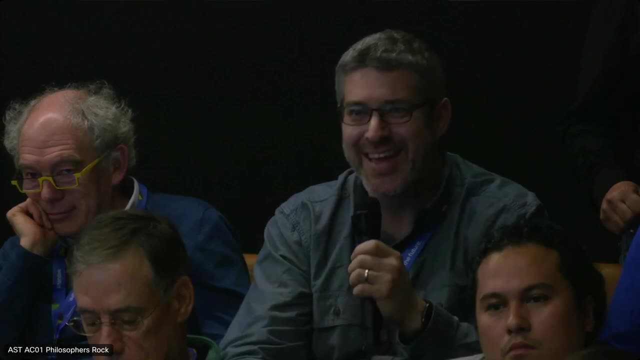 So you, you should be able to store there. Okay, so, any server, any table, as long as you specify. And then, and as long as you have privilege and you can access it, Of course, Can you specify multiple, multiple tables. 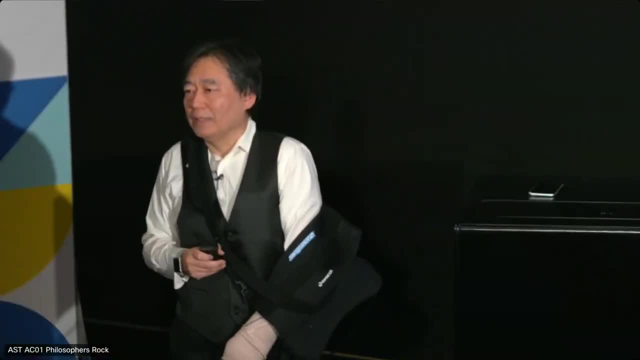 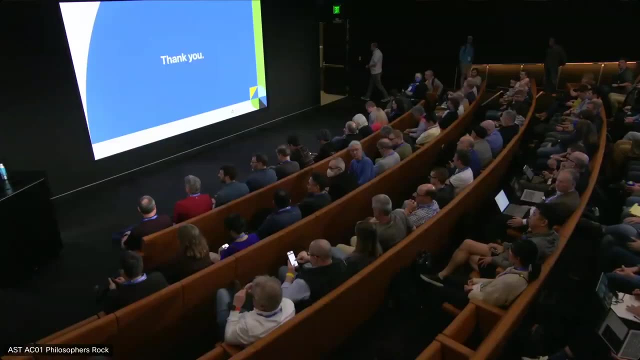 Not right now. Multiple table you. you need a space of one by one, Right? If you have a spatial case, They there's no. Thank you, So any more questions. We have time for more. Any more questions? 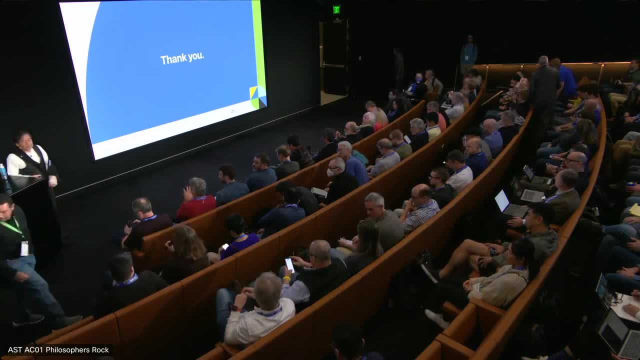 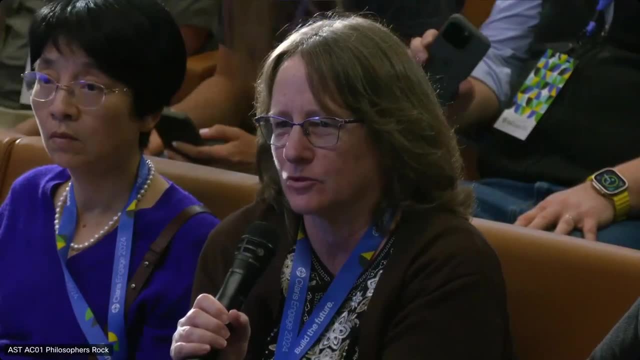 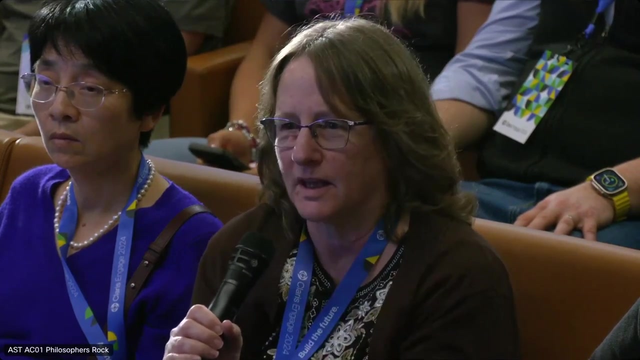 I have one right here. Would it be possible to set up a Rack server like in-house to test this without having to have subscriptions to an outside element? LLM, but you want to test it in-house, I see. so so the one I 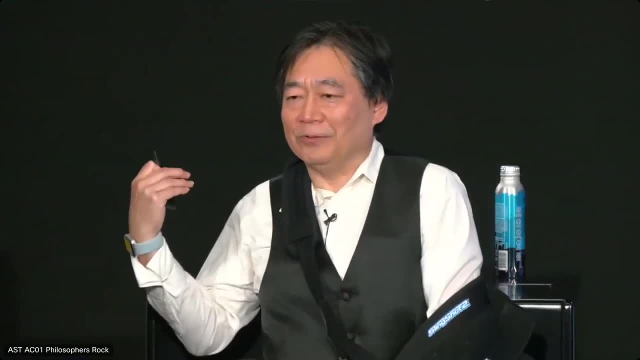 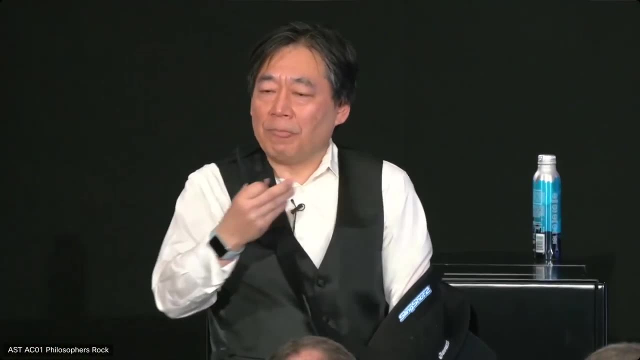 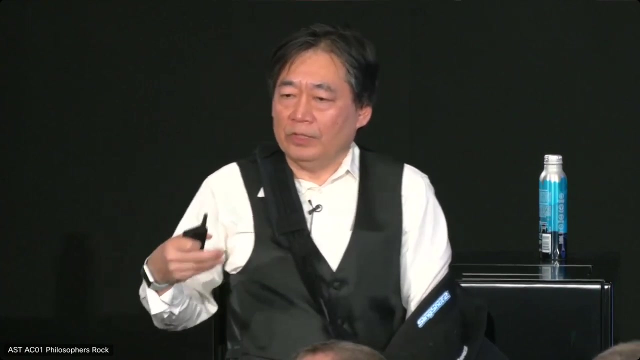 show you. actually, I set up, though I set up locally on my MacBook Pro, and the only thing I use outside is is that I use the. I use the GPT-4 to do the summary or final answer. so put this way: say if they, if you have you, say you. 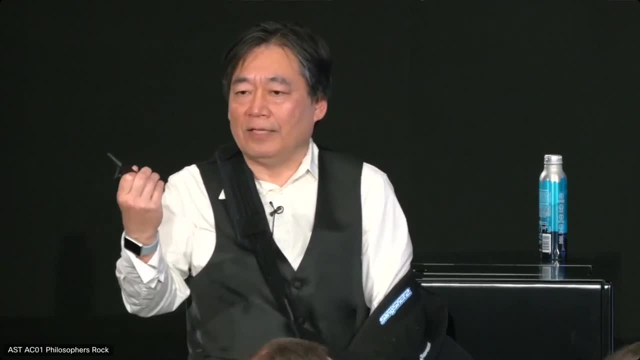 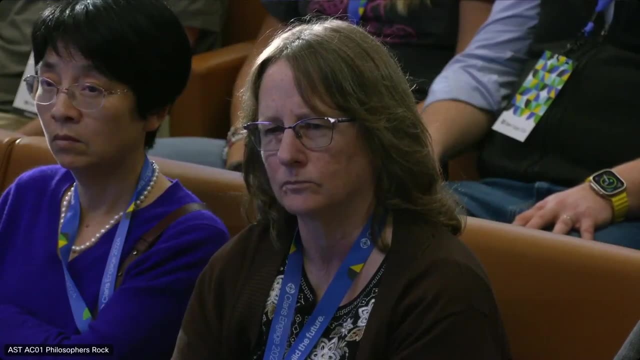 will keep you. you bring up you on open empathett attest server in-house, then you don't need to send to GPT-4 summary. they just sent to your chief the open chat 3.5. yeah, so so basically I show you the embedded method already get. 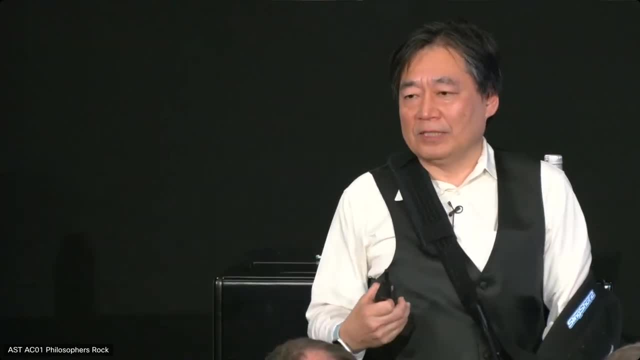 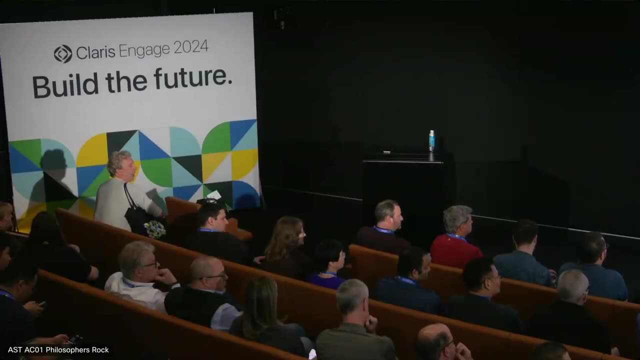 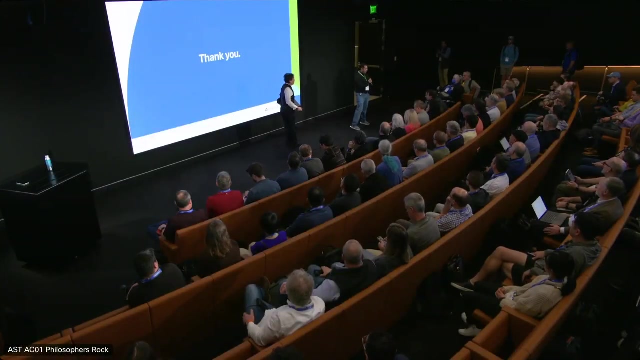 locally from my own open source sentence transformer. thank you, so so actually we already we have a- have a ETS version and that's how I pay up, Ronnie. Is that right? Ronnie, You've got to bribe me. No, we're like Wade said. 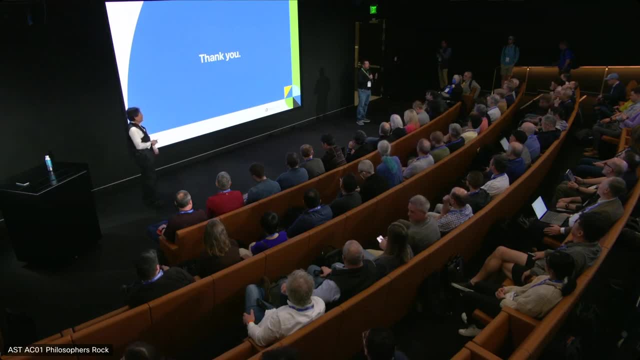 we're testing all these out. These are things that we're trying to figure out. what's the easiest way to bring all these technologies to you in the most file maker way possible, right? So we're experimenting. These guys have done- Wade and his team. 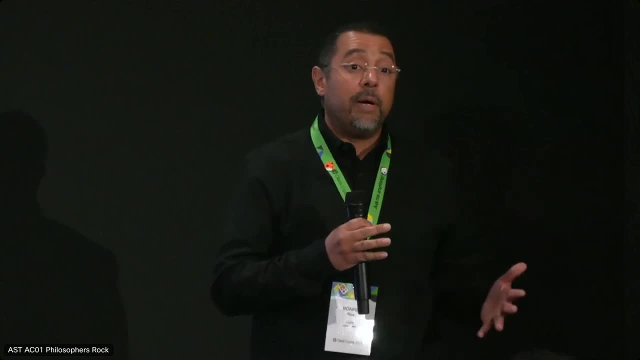 have done an amazing job. This is a lot of work and, honestly, in a short amount of time, So I think it's really amazing what they're doing. Again, we're trying to bring it as quickly as possible as best as to you. 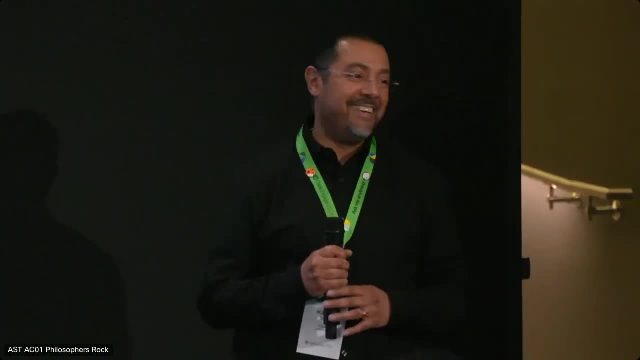 So join the group if you want to test this out.